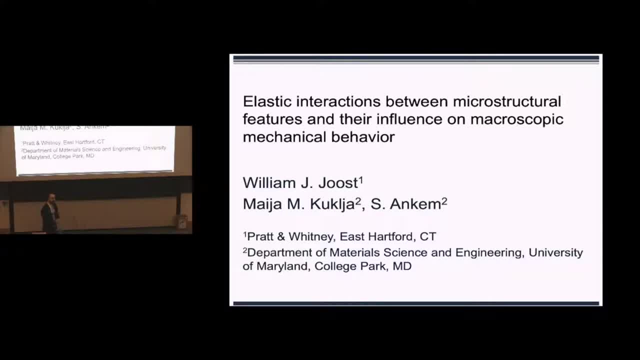 Ancum. They are wonderful people to whom I am eternally grateful. As you maybe all know or will have experience at some point, having a great PhD advisor is so important to your satisfaction during your PhD, the success in your career, So I really am very grateful to the two of them. 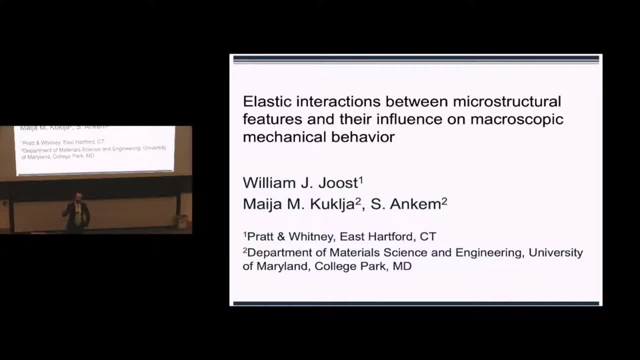 In any case. so what I'm going to talk about today is how elastic interactions between microstructural elements, in particularly titanium alloys, affect macroscopic behavior. I've generalized the title a little bit. You'll see there's nothing in there about titanium. That's because. 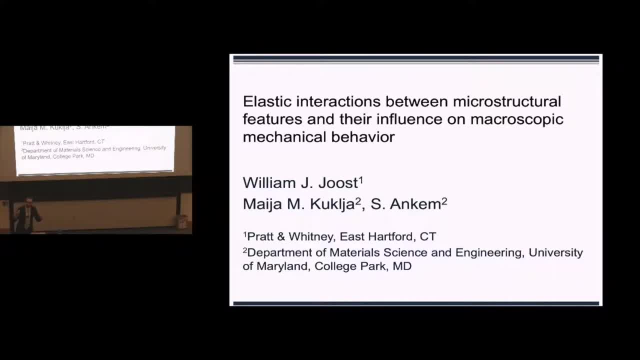 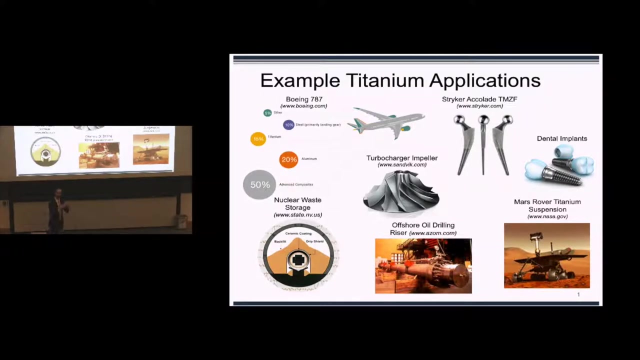 it's a few points. I will highlight how this could, in principle, be applicable to, perhaps, the work that you're doing. Also, since writing this title in abstract, I learned a little bit more about the folks that I'm interacting with today and tomorrow, So I've rearranged the furniture a bit. There is some added content that introduces some work in atomistics. It's all cohesive with the narrative, I hope. I know no abrupt gear shifts. We won't lose anybody, But in any case, there'll be a little extra to learn that goes beyond elastic interactions. So, as I mentioned, this entire talk is focused on titanium and titanium alloys, So I want to spend just a few slides here covering the background of some applications and some of the 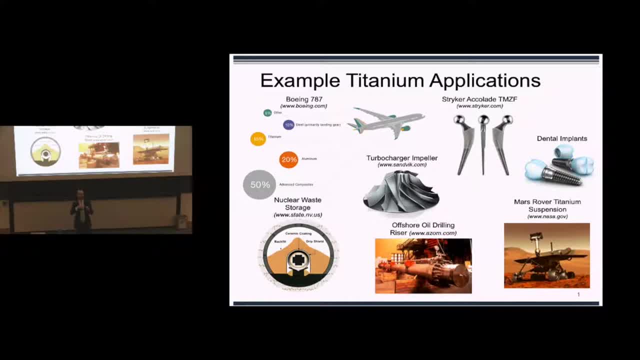 basics, the elementary bits of micromechanics that you will need to take with you for the rest of this talk so that it works. it makes sense that you hopefully learn something and go do fantastic work of your own. So, first and foremost, titanium alloys. find a whole broad range of applications from oil and gas, space aerospace. Brad and Whitney has a whole number of turbine- or not turbine, excuse me- compressor stages that are made out of titanium. biomedical applications, the Mars, Spirit and Opportunity Rover suspension components. 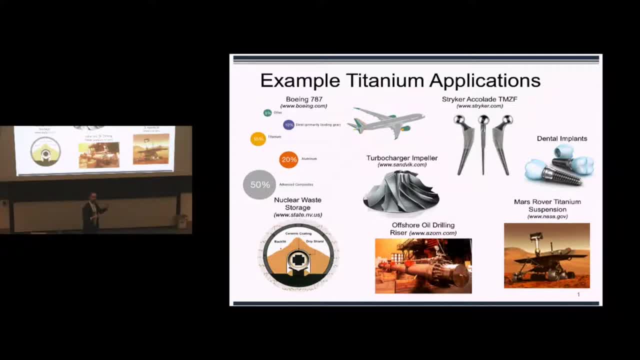 They're all made of titanium alloys, And so if you look at all these applications, you'll find, I'm sure, some number of common themes in those requirements, But one in particular is long-term mechanical stability right. These are systems that require that the geometry of what you have put in place remains for some relatively long duration. 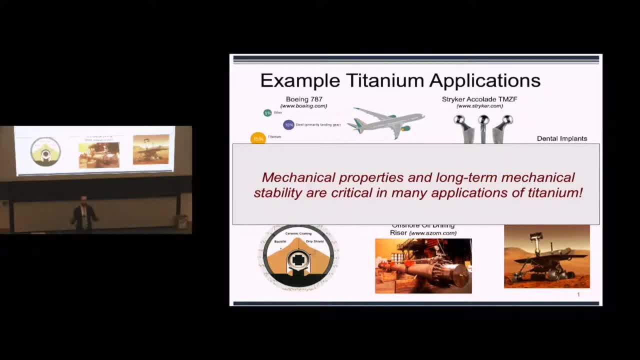 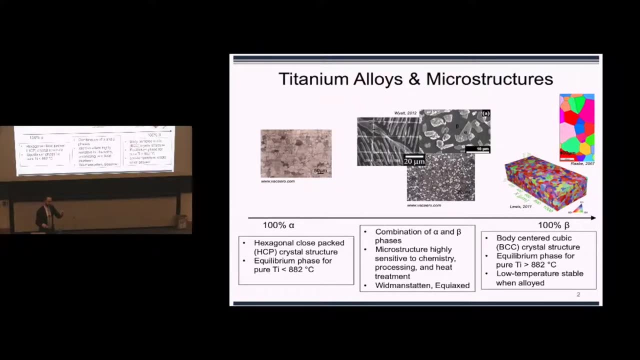 They do not sustain a large degree of strain over time. Certainly you wouldn't want your hip implant, your jet engine or whatever else it is to change geometry dramatically. So this is all very interesting. Before I dive into the details again, I do want to provide some background, since you may not all be titanium metallurgists. 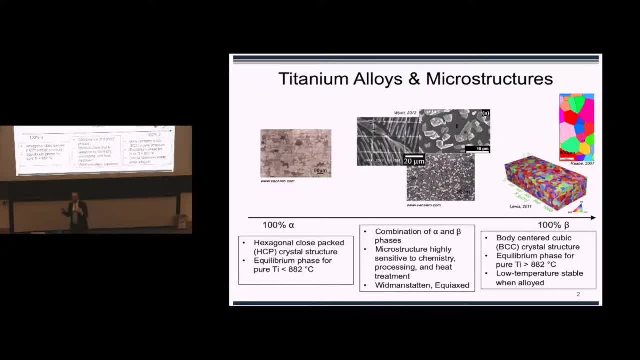 So, first of all, titanium. you can bin it a handful of different ways. The ways I've done it here is by the phases that are present in the different alloys. So on one hand you have alpha. So alpha is the room temperature equilibrium phase of pure titanium. 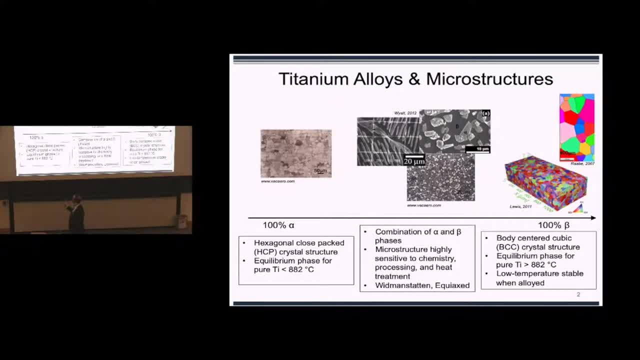 It is an excitable post-pack crystal structure. It's stable up to about 880 degrees C. If you take pure titanium and you heat it above 882, you form the beta phase. This is a body-centered cubic crystal structure, But very frequently in engineered titanium alloys what we do is we use this isomorphous phase transformation. 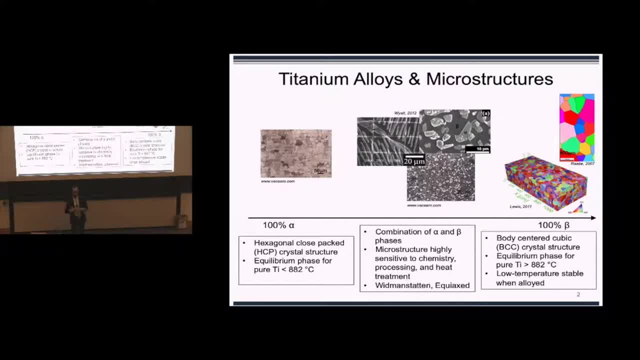 and we introduce either chemistry or, more often, chemistry and processing to create microstructures that contain both alpha and beta. Again, there's this large zoology of these microstructures. You could bin them. You could do it in any number of different ways. 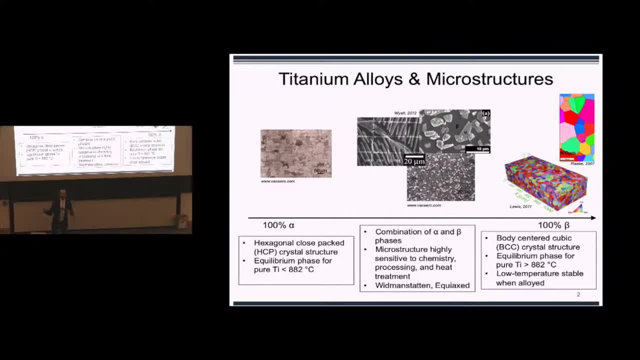 The way I've done it here is to say that we have in general, microstructures that are equiaxed, That is, the particles are sort of roughly spherical in a matrix, either alpha in beta or beta in alpha, And platelet, Lamellar, Widman-Statton- there are a number of different terms for this kind of microstructure. 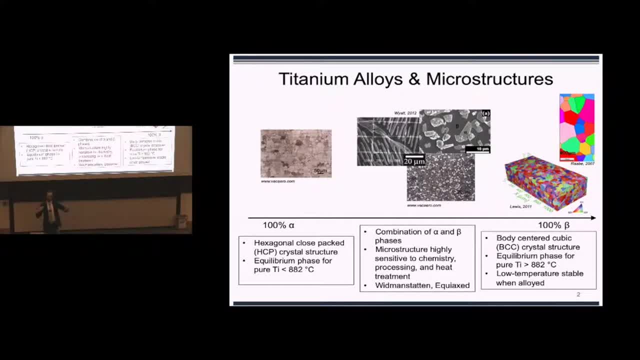 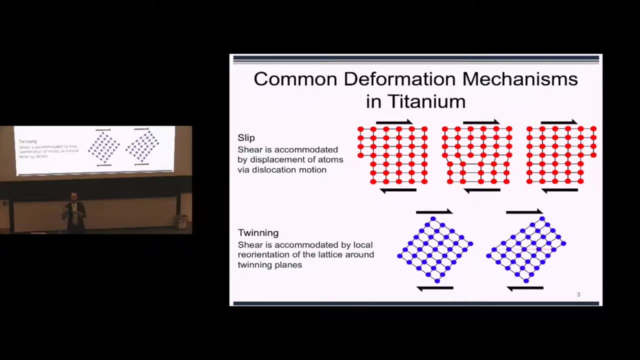 But in any case you have long, flat interfaces between alpha and beta. So this is the sort of world of titanium alloys put on one page. When you load a titanium alloy it can deform by a variety of different mechanisms, But for today's talk I'm going to focus on two that are dominant in some classes of titanium. 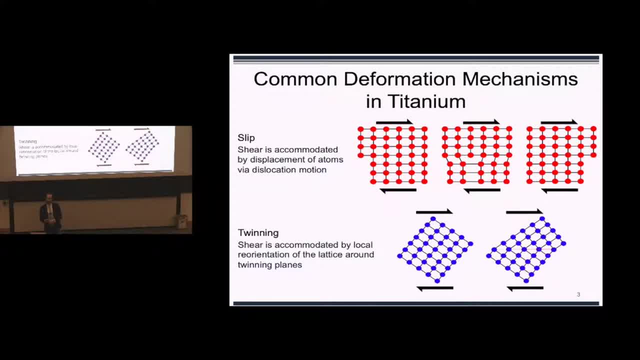 So the first is deformation by slip. Many of you are probably familiar with slip. This is the glide of dislocations that allows the system to accommodate shear. So as the dislocation moves, the lattice is adjusted by one Berger's vector for dislocation that moves past. 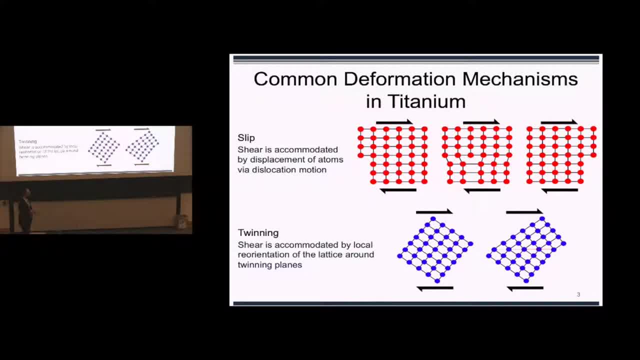 So again, this is probably something everyone at least has notional familiarity with in here. The second deformation mechanism that is important in some titanium alloys is twinning. You may or may not have come across twinning This again in slip. we're accommodating shear. 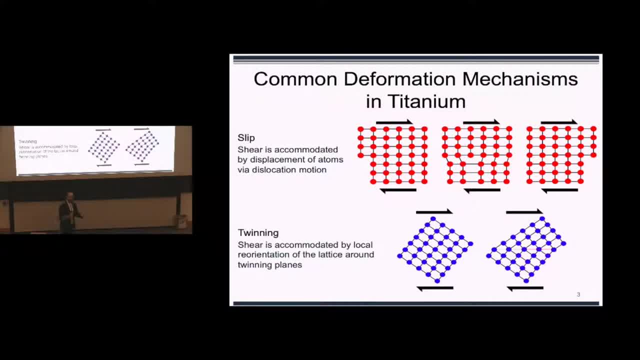 We're accommodating shear by moving dislocations In twinning. we're also accommodating shear. But we're accommodating shear by reorienting the lattice- the crystal lattice of the material about some plane. So here you have a rectangular lattice and you apply a shear and you reorient the lattice about this. 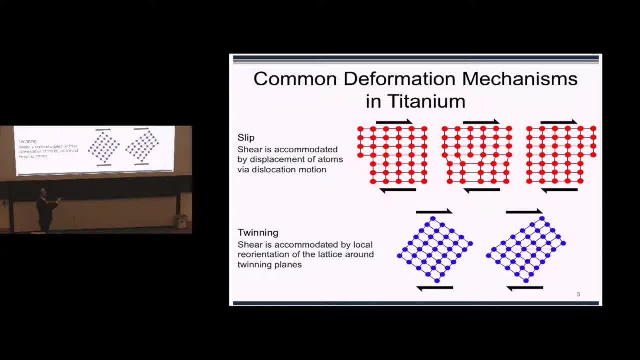 which is called the twinning plane, And you can see here sort of schematically, that this collection of atoms has accommodated shear. Okay, so that's In some sense how titanium atoms deform. Let's cover a little bit more background, that will be helpful. 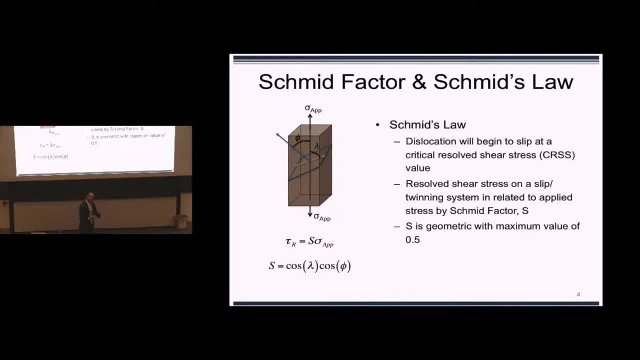 I want to talk about Schmitt's law and the Schmitt factor, Again, something perhaps you've come across in your coursework or your research, And basically the idea behind Schmitt's law is that when I take a block of material, be it titanium or something else, 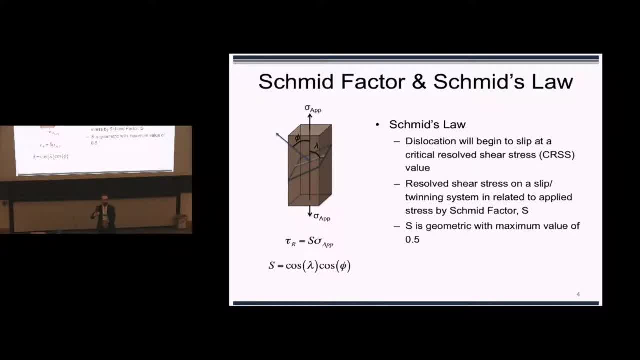 and I load it up, I can calculate how that applied stress resolves onto the slip or twinning systems in my material. The magnitude of that resolves shear stress. I should pick a side. The magnitude of that resolves shear stress is calculated as the Schmitt factor multiplied by the applied stress. 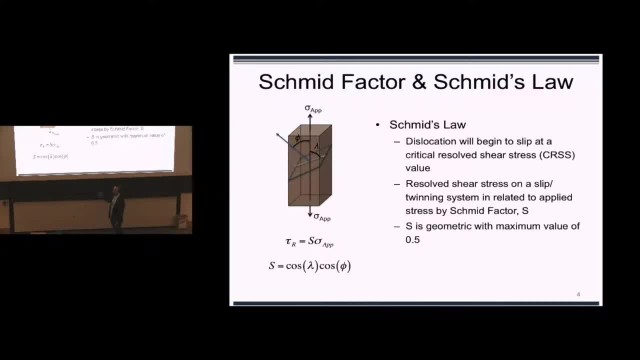 So some amount of applied stress resolves, and that fraction is S, And that fraction is generally calculated geometrically. It has to do with the angles between the applied stress and the slip and twinning planes. A key feature of this, because of the geometry of how this is laid out, is that S has a maximum value of 0.5.. 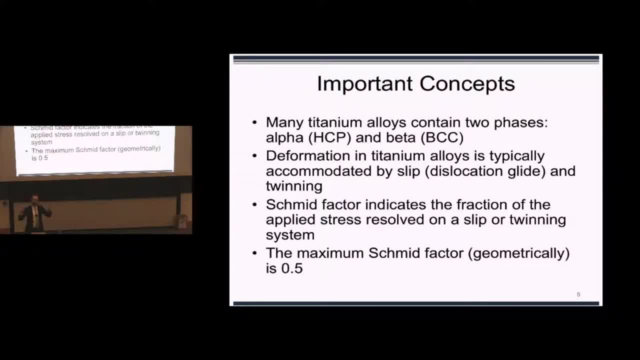 Okay, so this is what I just said, And I'm going to say it one more time because you will want to incorporate this information into RAM for the next 45 minutes or so, such that the rest of the talk will be helpful and useful. So again, titanium alloys in general contain two phases. There's a whole bunch of other stuff that could potentially be going on there: An alpha phase that is HCP, a beta phase that is BCC. These phases have different crystal symmetry. 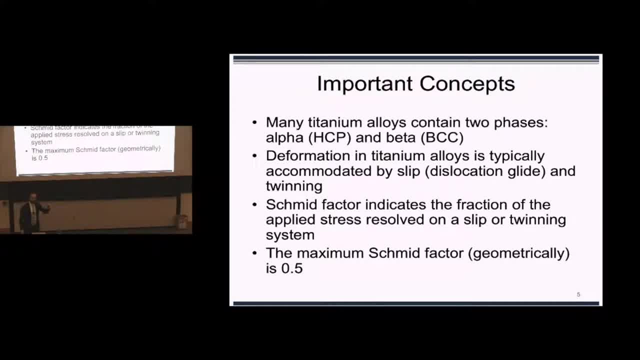 That does come into play later in the talk. Deformation generally occurs by slip, glided dislocations and twinning. The Schmitt factor indicates the fraction of the resolved shear, The fraction, excuse me, The applied stress that's resolved onto the slip or twinning system. 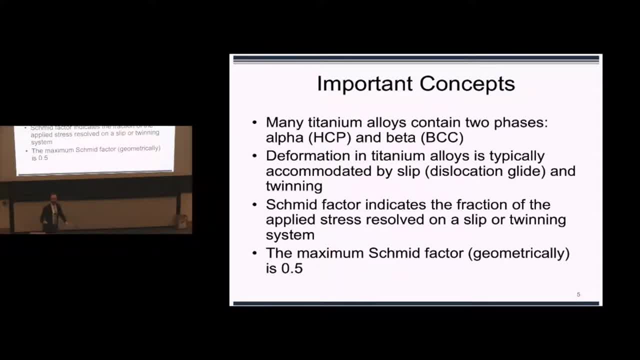 And in general, not in general. geometrically, strictly speaking, the Schmitt factor can have a maximum of 0.5.. Okay, so keep this, Put it in here, And we're going to keep going forward. So when we look at titanium alloys I mentioned in the first slide, 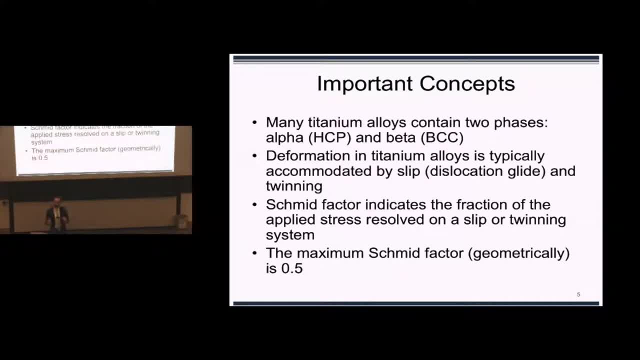 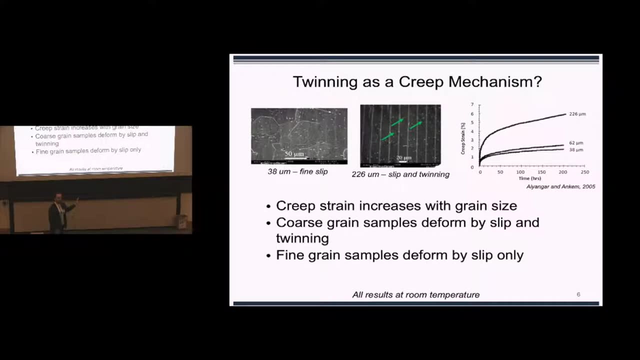 they have a lot of applications where long-term mechanical stability is extremely important, But they also exhibit a few characteristics that, in that context, are perhaps a little bit troubling. For example, in some cases titanium alloys creep at room temperature. So what I have here are some results from our lab, where we took a single phase alpha. 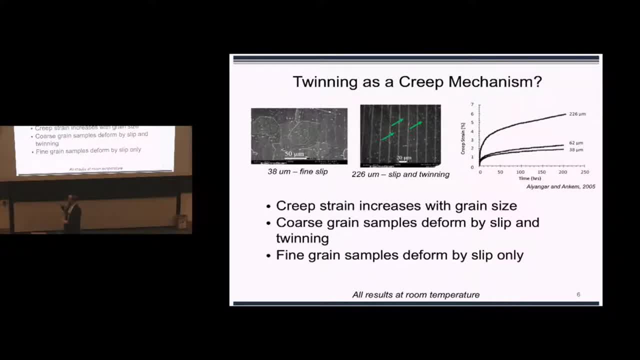 So there's no beta here. A single phase alpha microstructure at relatively fine grain size, 40 micron. We took the exact same material and we heat treated it such that we produced a version with 230 micron grains And we ran a fixed load creep test. 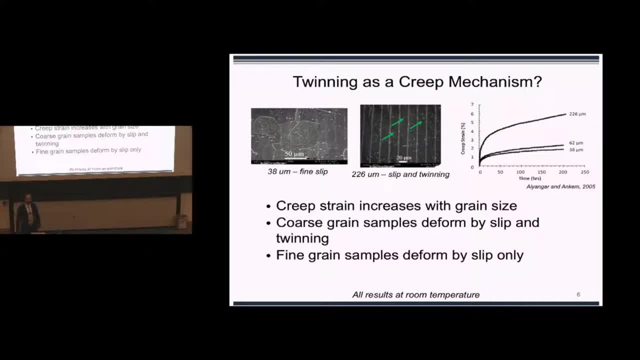 You take the sample and you hang a weight off the bottom and you wait patiently. And so what we found after running this? we found that the heat treated it at a rate of 0.5.. And so what we found after running this test for this particular material is that in some fine grain samples, 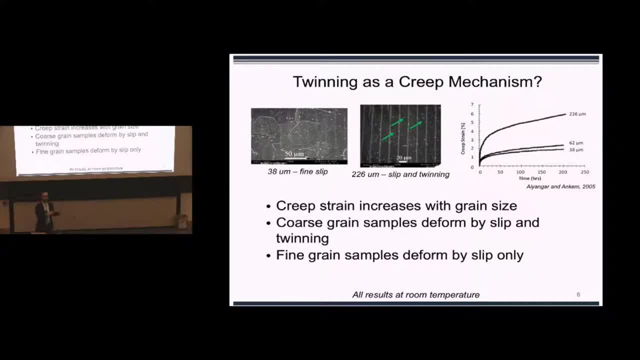 we do get appreciable creep strain. This would be bad news for a lot of engineering applications. But in any case, the fine grain samples show relatively little creep strain associated with deformation only by slip, Whereas in the coarse grains case what we find is deformation by twinning associated with a dramatic increase in creep strain. 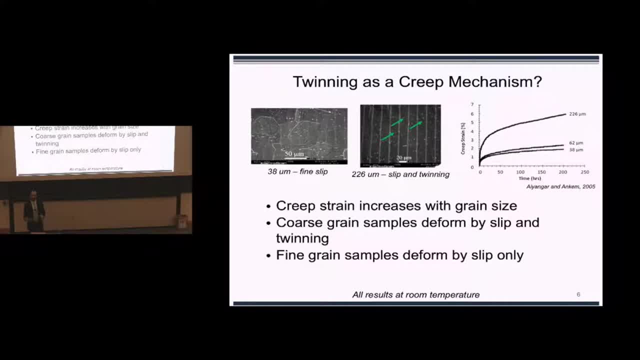 I am not aware of any sort of high-performance engineering system from that first slide that can accommodate 6% creep strain. But that is bad news for engineering design, in most cases using titanium alloys. So if anyone in here works in titanium or you've worked in some of this sort of stuff before, 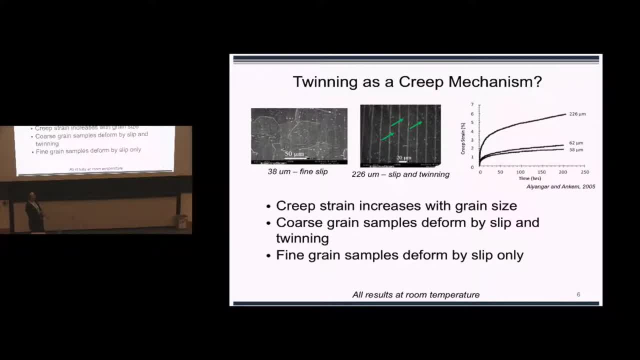 you would raise your hand and you would say, okay, well, that's fine, But we would never use this alloy like this for these applications, right, Specifically because of this kind of behavior. This is maybe academically interesting, which is fine by itself. 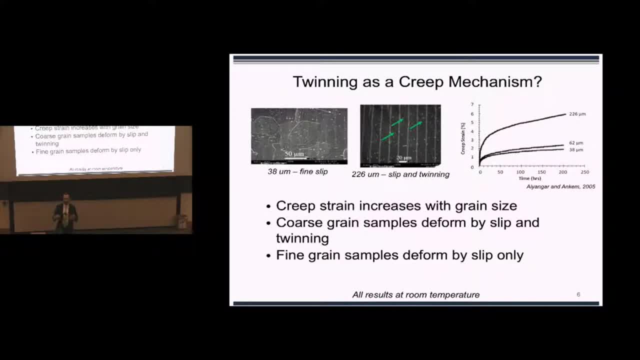 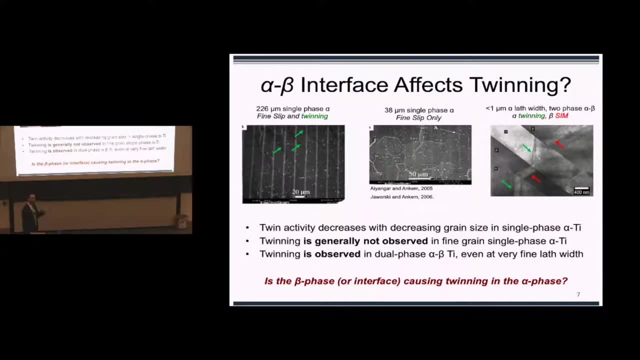 But in the real world we would alloy this and process it as to introduce a beta phase and to give us some resistance to this sort of creep behavior. What's very interesting is that in some of these alloys, when you do that, you still observe this exact kind of behavior that can be very detrimental to performance. 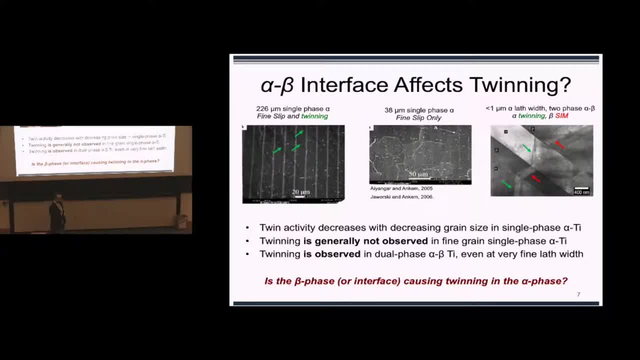 So what I'm showing is the same two pictures. I've got a coarse microstructure here with twinning that has relatively high grain size, relatively large grain size, relatively large creep strains. I make the grain size finer. It transitions to slip only. 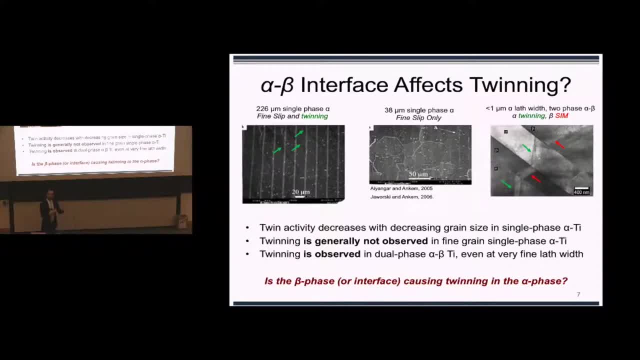 This is very common among HCP metals. It's not just unique to titanium. Now I alloy it and I process it. Very importantly, I do this in such a way that the alpha phase here has the same chemistry as the alpha phase in these samples. 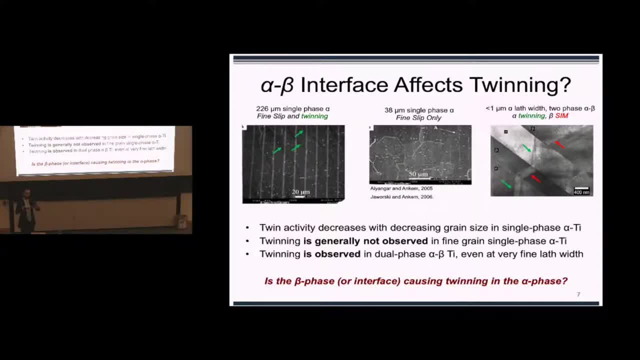 The bulk chemistry of this alloy has to be different, because I've stabilized the beta but I heat-treated it in such a way that the alpha phase that precipitates out is the same chemistry. So there's no chemistry effect here. I have very fine grain size, very fine alpha feature size in this case. 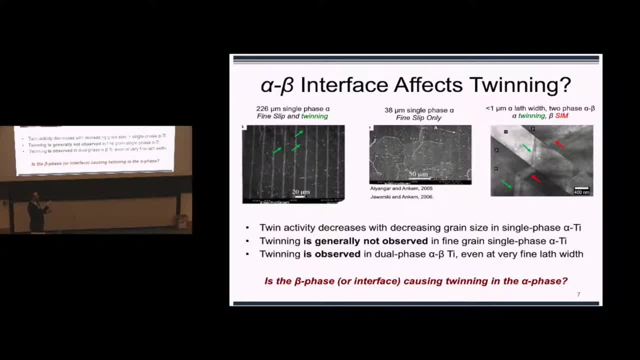 So I go coarse: twinning, fine, no-twinning, extra fine with beta. and twinning comes back. And when I look around these microstructures in post-creep tests, I find that samples that have creeped in a population that is distinct from the others. 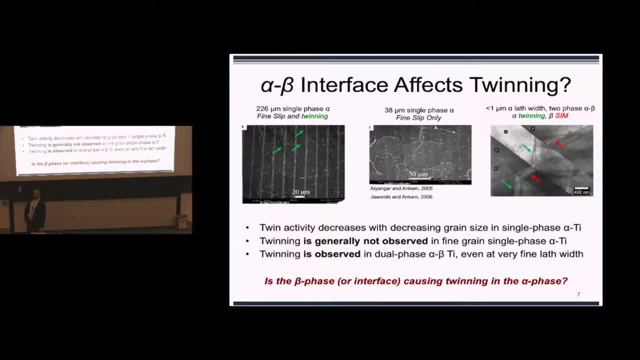 show these features. These twin bands run across the microstructure and just sort of unzip as the sample creeps. It doesn't happen all the time. We don't really understand why. We didn't really understand why at the start here anyway, But in any case we see this. 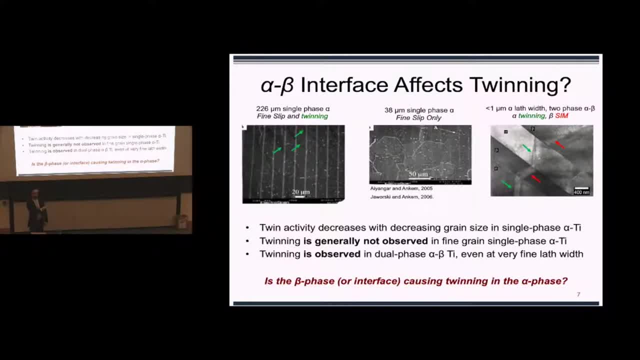 And the question we posed is: okay. well, obviously, we have no beta phase here. We have beta phase here, No twinning, yes, twinning. Is the beta phase or the interface between the alpha and beta phase responsible? Well, the beta phase is responsible for the formation of these twins. 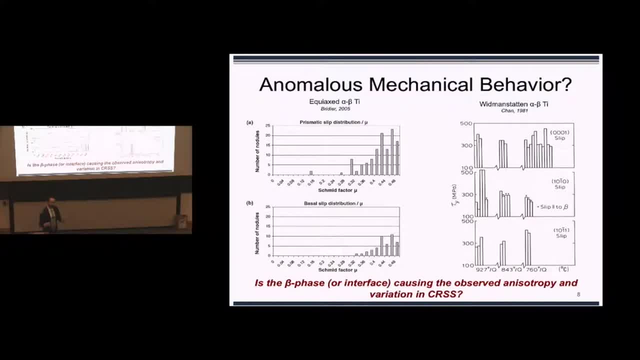 So let's look at something kind of in a similar vein but a little bit different. So again, I mentioned that Schmitt's law, generally speaking, would tell you that if you apply a tensile stress or whatever stress to a sample and you resolve that stress onto a slip system, 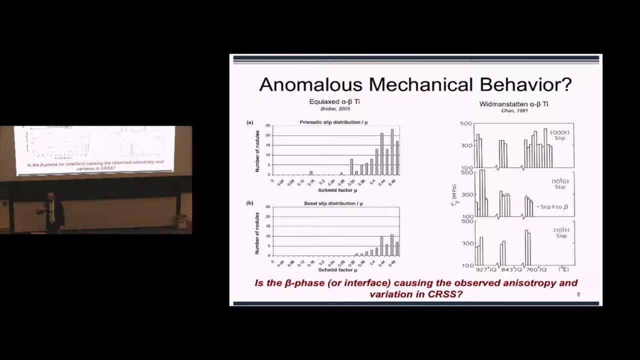 at some critical value, at some critical resolved shear stress, the dislocations will start to glide, And so, in principle that critical resolved shear stress should be more or less constant within a material, There are reasons that that could be untrue. What we find is, in dual-phase alloys, that there is a wide variety of critical resolved shear stresses that are reported. 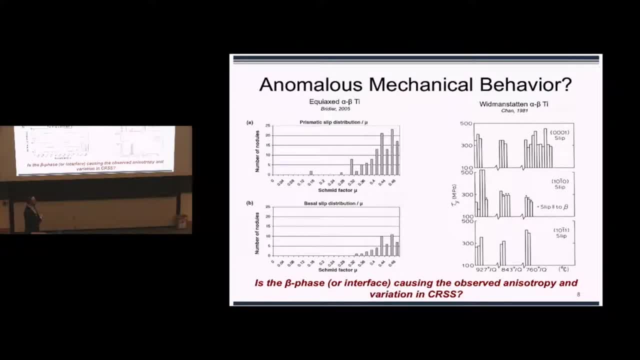 So I have two examples here- These are not from my own work- An equiaxed alpha-beta, And what we see is essentially what they did is they pulled a sample and they went in and they looked at every alpha particle in the microstructure. 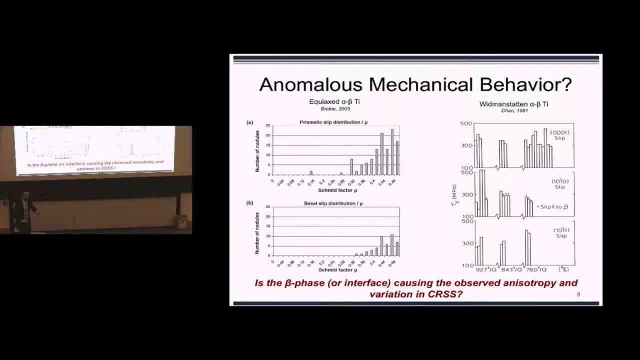 and they categorized the Schmitt factor for slip in those particles And normally what you would expect to find in that case is deformation only for very high Schmitt factors. You would see sort of these guys, But what they find is deformation at very low Schmitt factors. 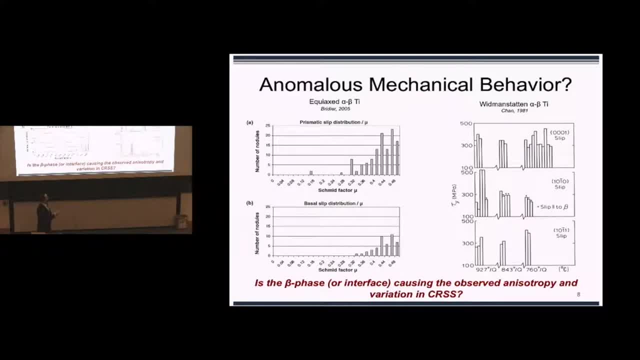 some very strange behavior here and it's not clear why. Similarly in Lamellar Wittmann-Staten-type microstructures. so again, this is where you have alpha and beta plates. what we find is that in some cases, I'd say the best way to look at this is just to focus on this particular data here. 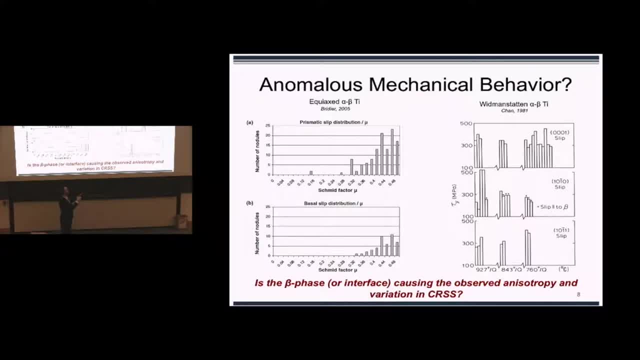 So you have one particular heat treat, one particular slip system and the range of critical resolved shear stresses for basal slip in these is a factor of two. So now again we have this question: Okay, is the beta phase responsible for this? 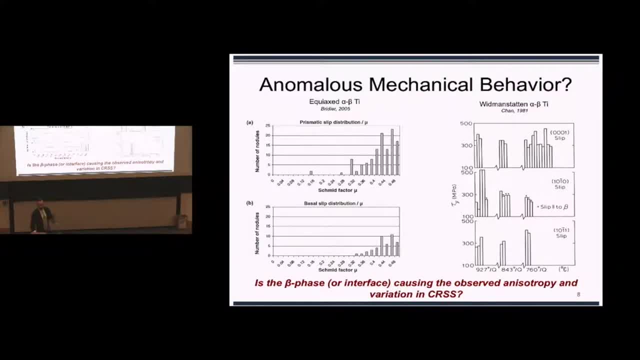 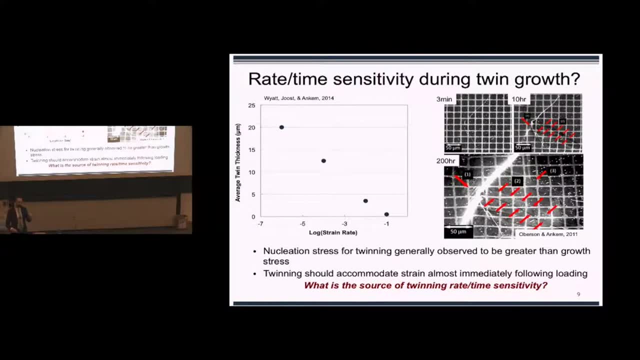 What's going on here? So the last little piece of background here that stimulated this research. again, if you've kind of worked in this space, and particularly if you've worked in twinning, you would ask yourself: well, this sort of sounds all like nonsense. 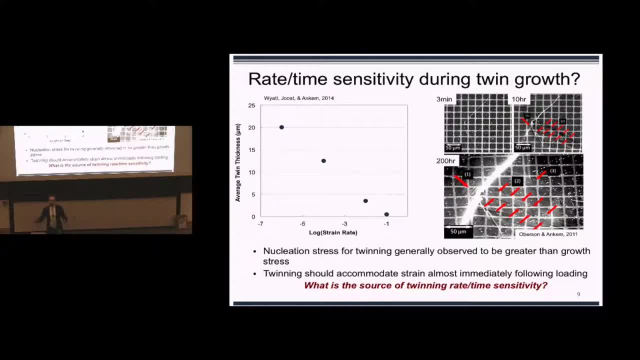 because twinning is generally assumed to happen very, very fast. If you go back to the classical papers from twinning, they assume, or they state, that twinning growth occurs roughly at the speed of sound in a metal, the logic being that in almost all cases, 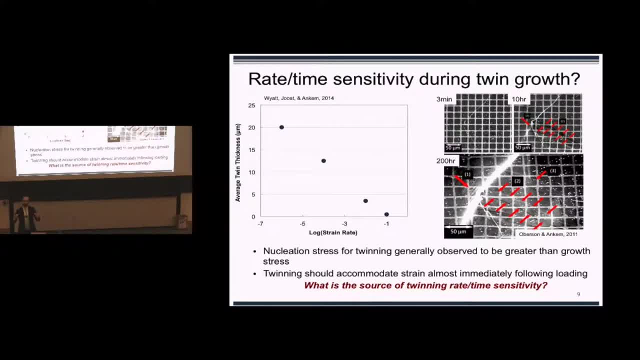 the stress. The stress required to nucleate a twin is greater than the stress required to grow the twin. So once you hit that nucleation stress you are way over the growth stress. The twin will accommodate as much strain as it possibly can before it encounters some other sort of boundary. 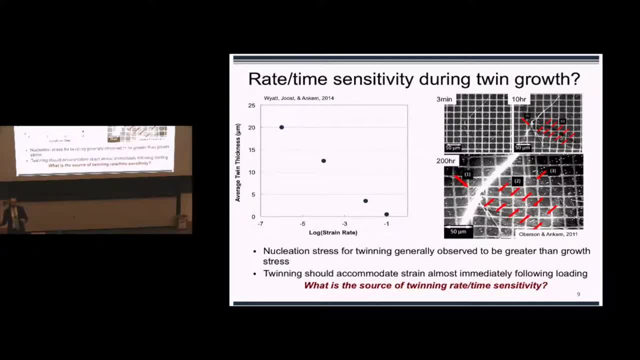 So there shouldn't be a time dependence to twinning And you need time dependence in twinning to get the creep. So what we started looking at was first just straightforwardly investigating: is there actually time dependence in twinning independent of creep? test for titanium. 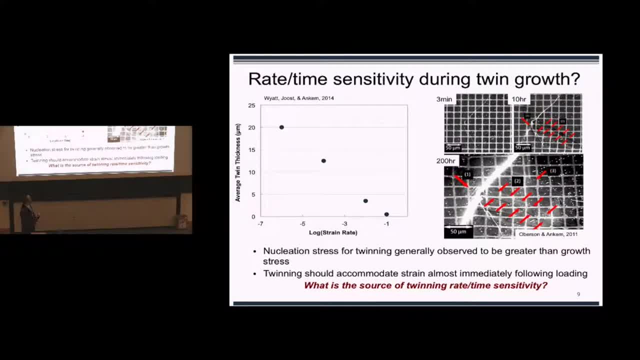 So What we found is we looked at this two different ways. So one is to pull tensile samples at a variety of different strain rates and look at the twin thickness for a fixed strain. So if there's no strain, if there's no time dependence for twin growth. 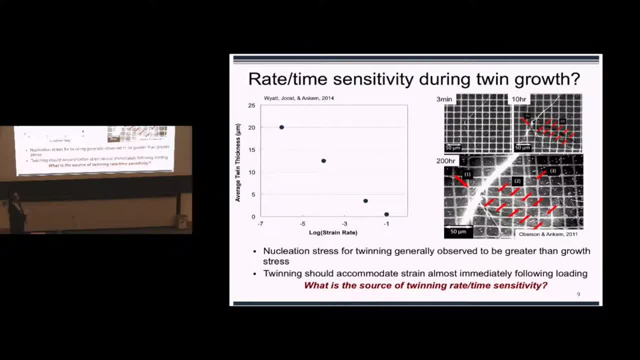 there should be no variation with strain rate, particularly at these sort of low strain rates. What we find is very strong variation in twin thickness. Similarly, and much more straightforwardly right, we can just load up a sample and let it creep for some number of hours. 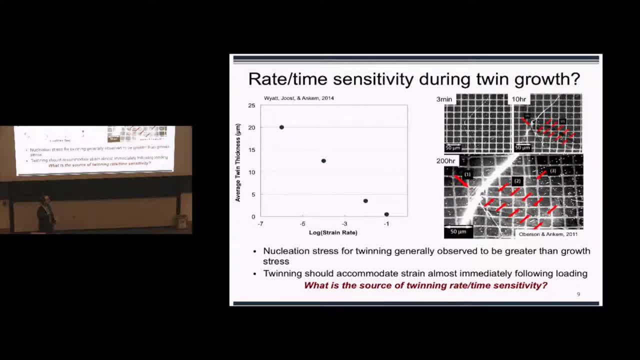 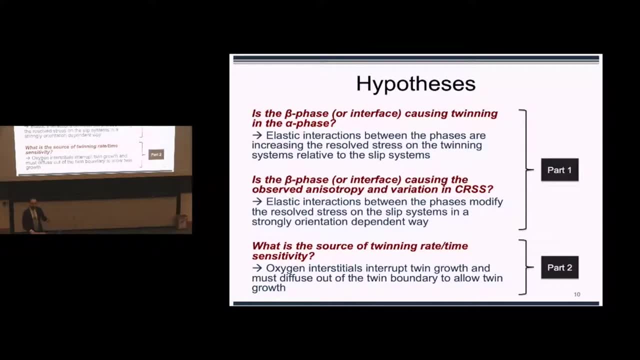 and go and look at the same twin again and again and see if it's growing slowly, And indeed we find it is. So what is the source of this sensitivity? So, basically, what I've just outlined is three big questions that I'm going to go forward in the rest of the talk and try to answer. 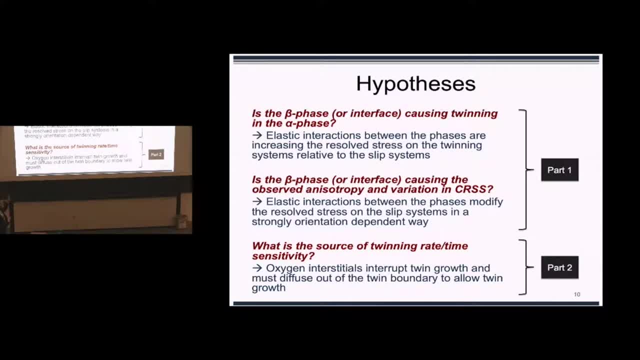 show you how we approach these problems And the way that I've broken this down. so the first two questions are: is the beta phase responsible? Is the interaction of the beta phase, the interface with the beta phase, or whatever it is responsible for the twinning in the very, very fine-grain alpha laths? 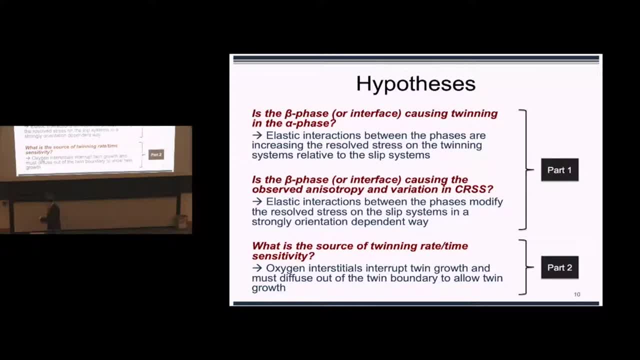 despite the fact that we never see twinning in fine-grain pure alpha. Is the beta phase responsible for this sort of anomalous behavior, this strange distribution of critical result shear stresses in the dual-phase alleys, And in both cases our hypothesis is that it is the elastic interaction. 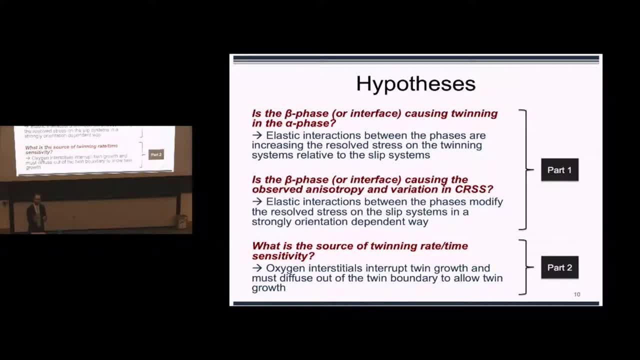 between the alpha and beta. that's creating a local stress field that causes this to happen. So I'll walk you through how we assess that, how we analyze it and what our results are. Now, like I said, I did add a little bit of bonus content. 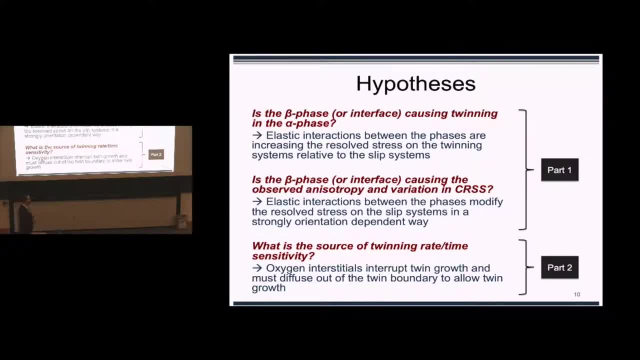 I think, to better fit sort of the group we have. So that is The question of what is the strain rate, sensitivity of twinning. where is that coming from? what is the mechanism? And our hypothesis here is that it has something to do with oxygen reciduals in the lattice. 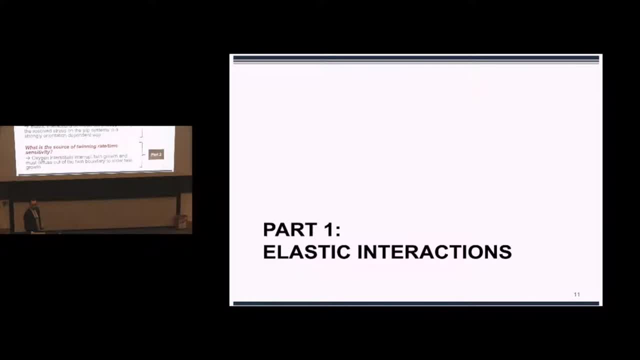 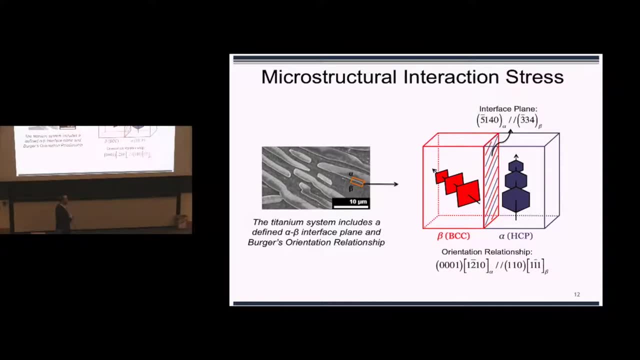 so we'll talk through that. So, without any further ado, we will jump right in to part one: elastic interactions. So imagine that I have a titanium alloy and I go into my titanium alloy and I cut a really, really, really small. 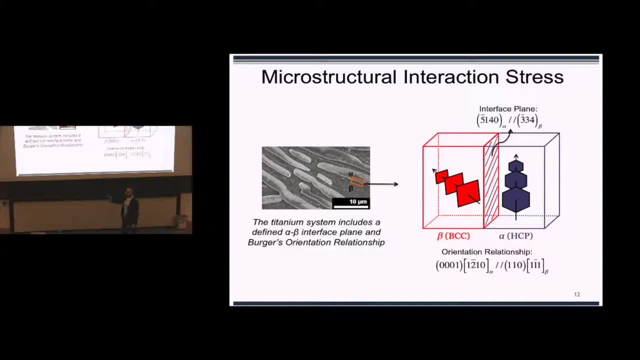 very, very small tensile sample, like this little box. So the first thing I'm going to do is I'm going to take out my. I'm going to take out my tensile sample and I'm going to analyze the crystallographic characteristics of this sample. 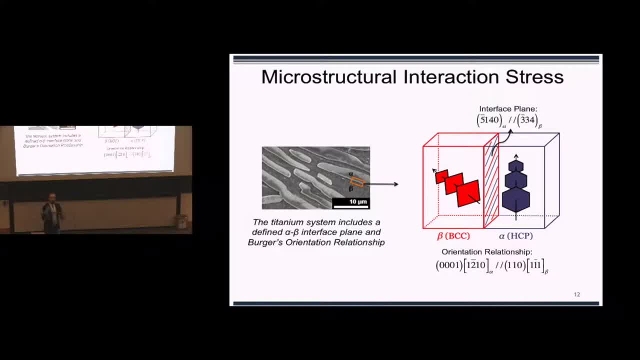 And in a lamellar microstructure, excuse me- like this one. I will find a few characteristics of that interface. So the first one is that there is a defined interface plane between the alpha and beta, right Between the alpha and beta side here. 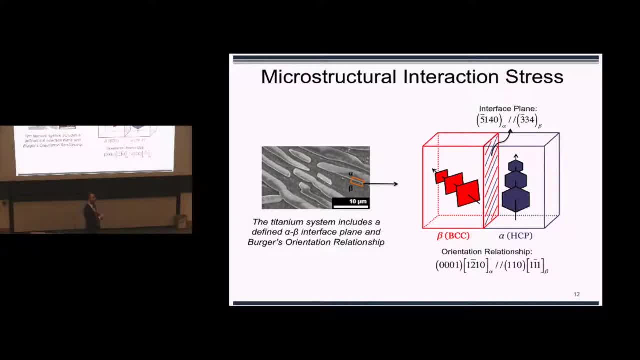 And it's this sort of weird high index thing, The beta, this basically what this means is this plane in beta is bar three, three, four right Some particular crystallographic plane, And this plane in alpha is bar five, one, four L. 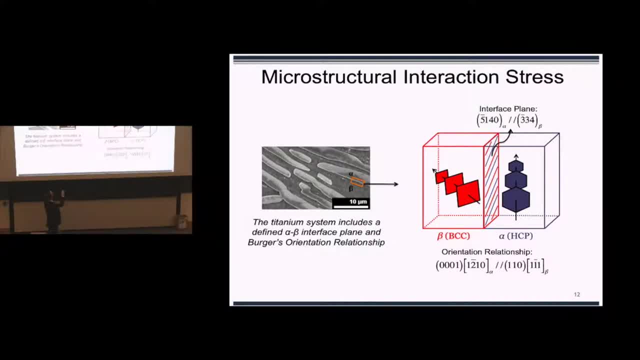 So that's the first thing that I will find on all of these long interfaces here, And the second thing that I will find is that the close-packed planes and directions are lined up. So I have the close-packed basal plane and A direction in HCP. 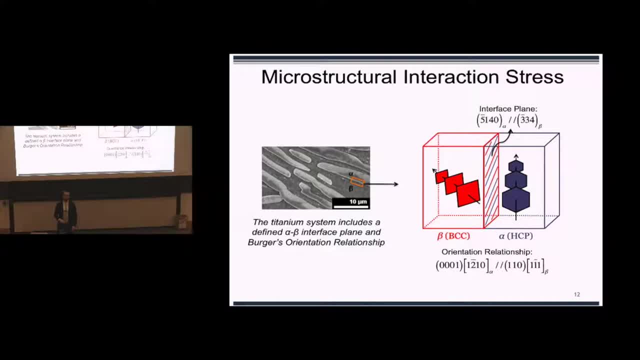 is lined up with the close-packed plane and direction in VCC, So this is broadly true across all of these interfaces here. This has been well merited by experiments. It's interesting, by the way, to note one of the reasons that titanium does this. 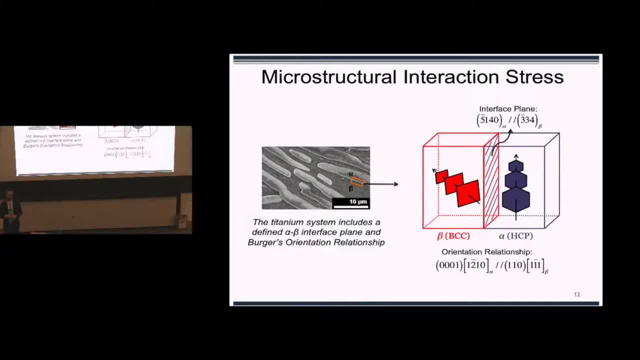 is able to maintain these relationships, whereas other materials- steel for example- doesn't do this, is that the volume transformation, when you transform from alpha to beta, is very small, So it allows the system to maintain this nice, comfortable Berger's orientation relationship. 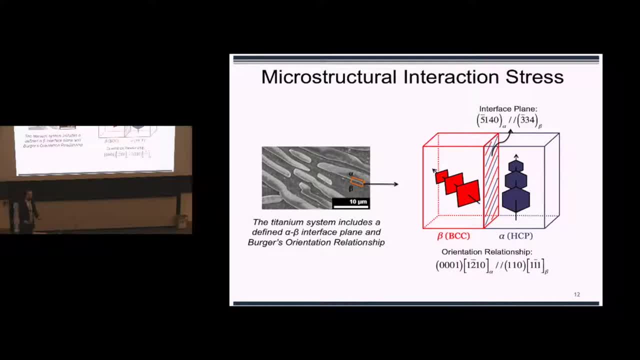 It doesn't have to accommodate a lot of strain when the system transforms from beta to alpha or vice versa. Okay, so I've taken my tensile sample and I've characterized that I have these, these different characteristics. So now I'm going to pull a test. 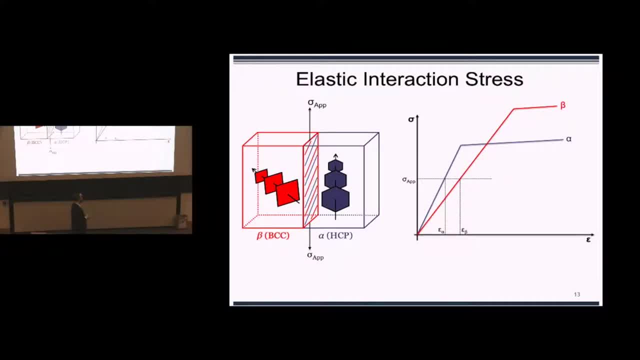 I have a very small instrument and I'm going to, I'm going to give it a load, And so let's talk about what would happen here. Schematically, it works like this: I apply a stress and very, very far out, way over here, somewhere in the distant alpha phase. 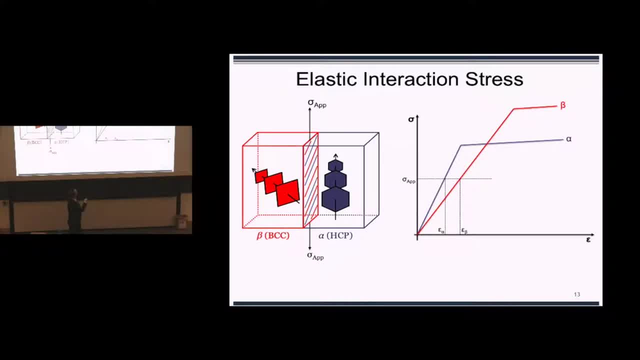 I have a strain right. I can read right off the stress-strain curve here And way over here somewhere in the beta phase. I have another strain here. However, because of that Berger's orientation, I can read right off the stress-strain curve here: 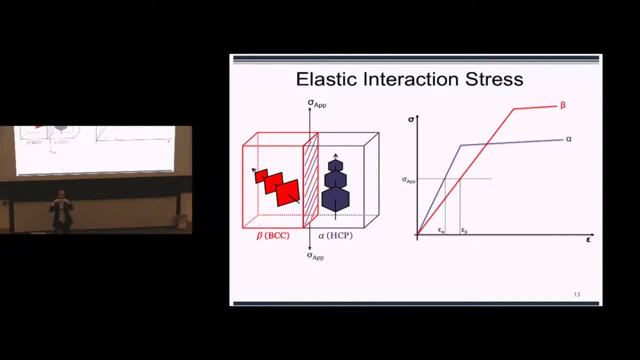 I can read right off the stress-strain curve. here I have close-packed planes lined up with one another. There is very, very effective bonding between the alpha and beta. This is not an interface that slides, And so, from a mechanic standpoint, we call that a traction compatibility requirement. 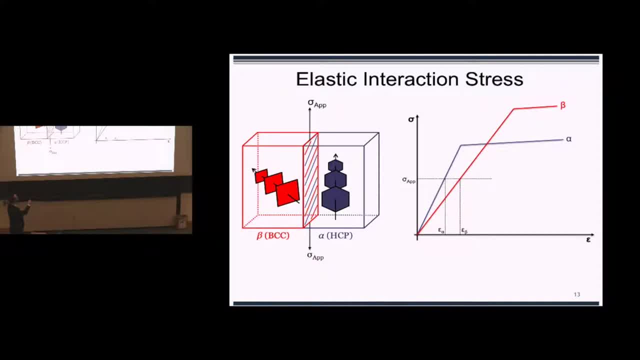 or there's a displacement compatibility requirement. What that means is right at the interface: whatever the strain is in alpha, the strain is the same in beta. Or, more strictly speaking, whatever the displacement is in alpha, the displacement is in beta. 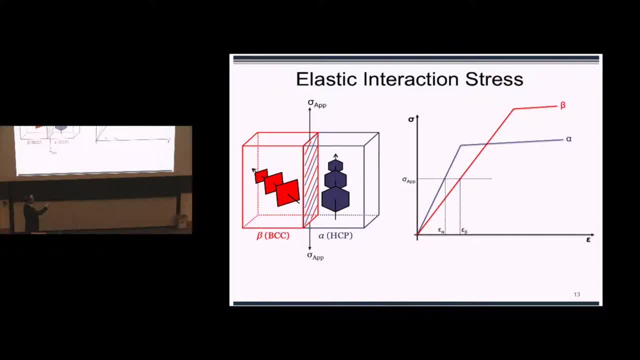 So, even though far away from the interface, the alpha strain is here and the beta strain is here near the interface, it has to be the same on both sides and somewhere in the middle, like this. So now what that means is again right off the stress-strain curves. 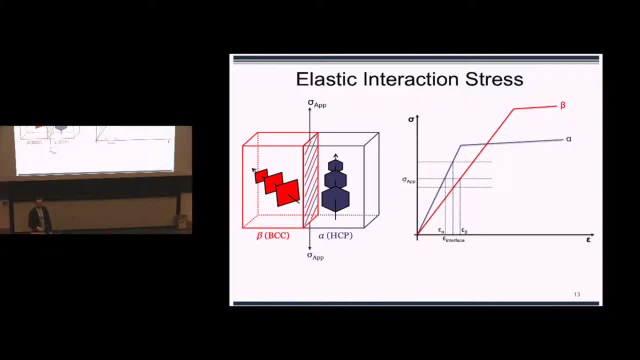 I can read the stress in both of those phases right at the interface. They are here and here, And this again schematically. you can do this in a longer form with a lot of tensors, but it's schematically the source of these interaction stresses. 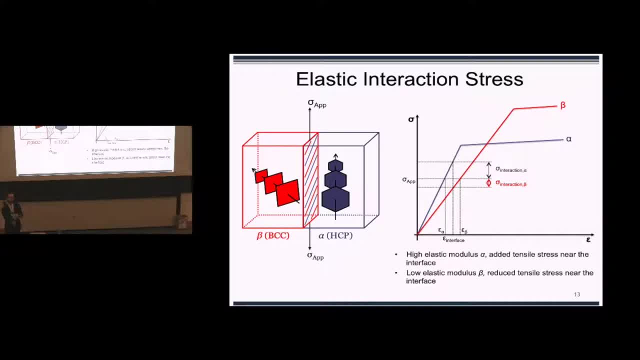 So when you have a stiff material up against a soft material and you pull them in tension, the stiff material experiences a positive interaction stress. This stress that alpha feels right at the interface is greater than the applied stress. And so, if you're kind of thinking about what I said at the start here, 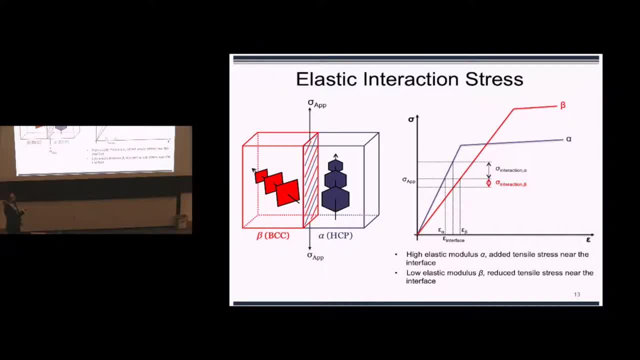 you might start to detect that maybe this additional interaction stress is resolving uniquely onto the twinning systems or is resolving in a very orientation-dependent way that causes that anomalous mechanical behavior and gives us the results that we see experimentally. So that's what we set to find out. 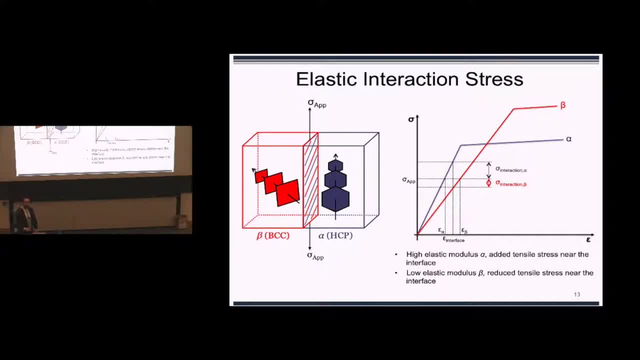 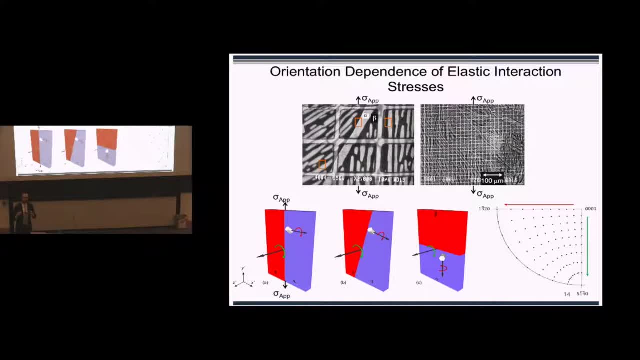 The thing is that this one tensile sample isn't going to answer the question for us. We need to be a little bit more systematic in how we explore this space And indeed we actually have to identify specifically what are the degrees of freedom in this system that we can explore. 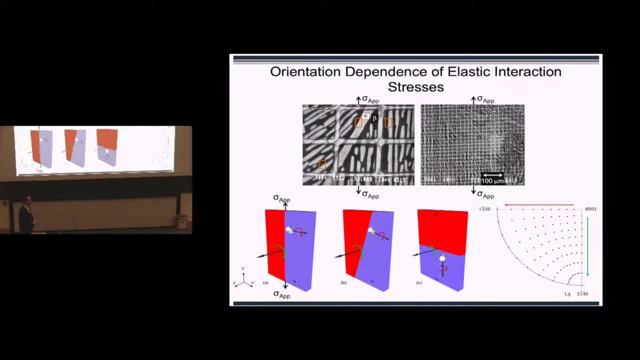 to fully represent how these interaction stresses exist. So the way we do that is the following. So you can imagine, right, I cut my little micro-tensile sample on the previous slide. So let's say now I cut one here and that interface is this angle. 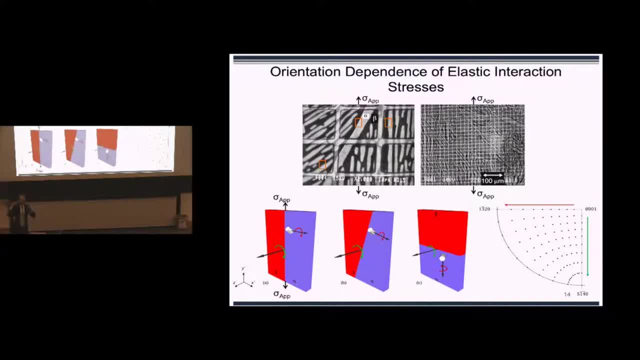 I cut one here in the interface. I cut one here in the interface is vertical right, So this sort of reveals the first degree of freedom. is the angle between that interface normal and my loading direction, And so I've put this picture. 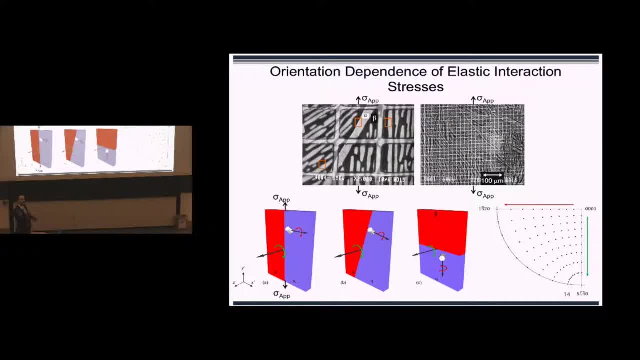 I didn't draw the little boxes because they'd be really tiny, But the basic idea is that that interface can be at any angle relative to the loading direction. But I have a second degree of freedom, So I mentioned that the alpha phase interface plane is bar 5, 1, 4, 0.. 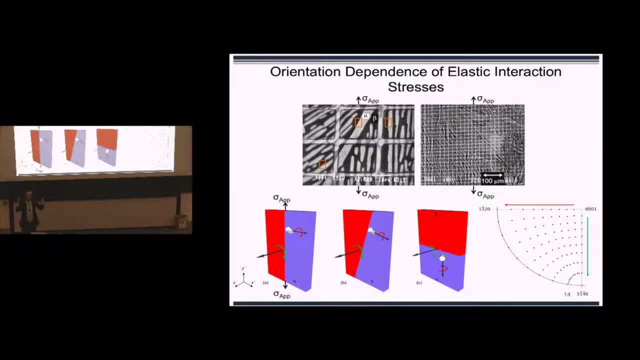 So what is this? This is a very strange high-index plane. But the key is that this is a very strange high-index plane And the key thing when you read that, what you can pay attention to is the zero at the end. 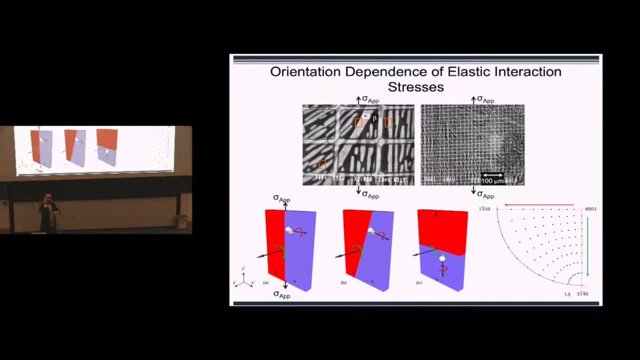 Because what the zero at the end of the crystallographic index for that plane means is that the c-axis is parallel to that plane. right, This little hexagonal, this one probably shows up better The hexagonal crystal structure of alpha. the c-axis cannot tilt towards the interface. 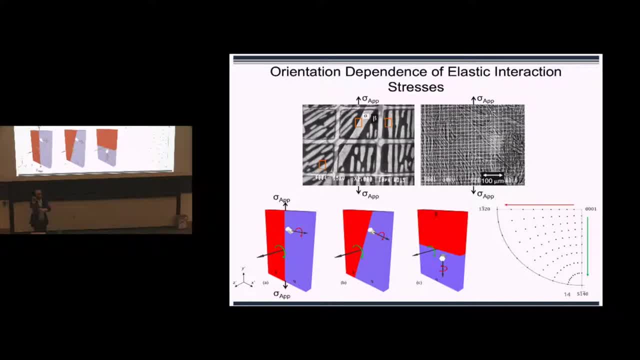 because it would break that defined interface plane. However, the c-axis can rotate right. So if I have my interface plane and I have my c-axis, I have one more degree of freedom in rotation Because of that Berger's orientation relationship. 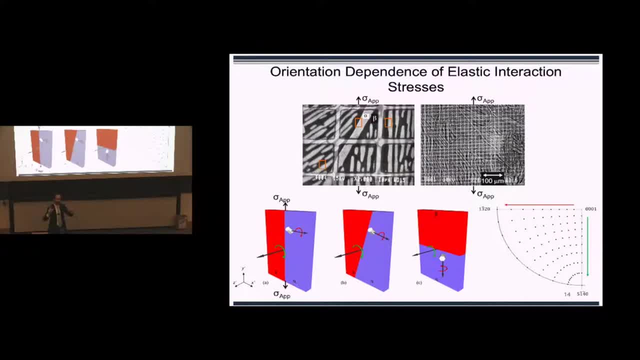 when I rotate, alpha beta goes along for the ride. They rotate together. So these are my two degrees of freedom. So what I want to simulate in order to capture the entire space is sort of roughly shown here I have the first degree of freedom. 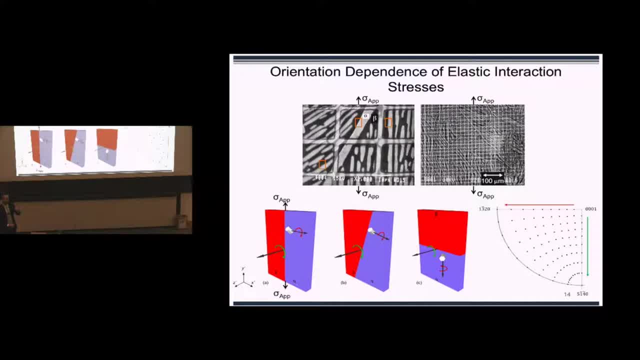 which is I'm going to change the angle of this interface as I pull the samples And for each of those interface orientations I'm going to rotate the crystallographic orientation. So I've plotted this on a stereographic projection. here I will say some of you may look at stereographic projections all day, every day. 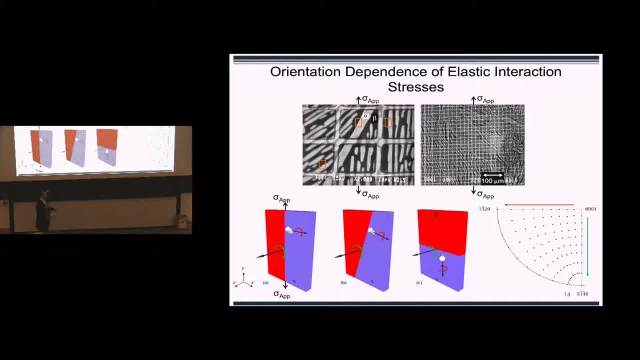 in which case this is very natural. Some of you may not. For those of you who are in the stereographic projection world, this is the alpha-001 projection. So basically what these points mean. each point represents one simulation And it tells me the orientation of the applied stress relative to the c-axis of alpha. 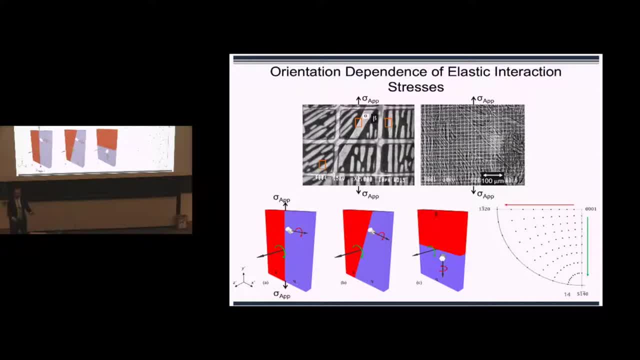 If none of that made any sense to you, because you don't really work with this stuff, don't worry about it. The important thing to take away is that this is a way that I can- you know, this is a way that I can map- map every single one of these simulations. 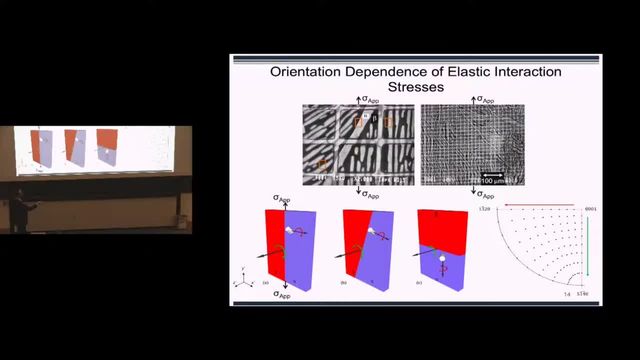 So if I run one simulation here and I get a value of four, I can put four. and I run a different simulation here and I get nine, I can put nine, And so I can plot on this little quadrant the results from all my simulations. 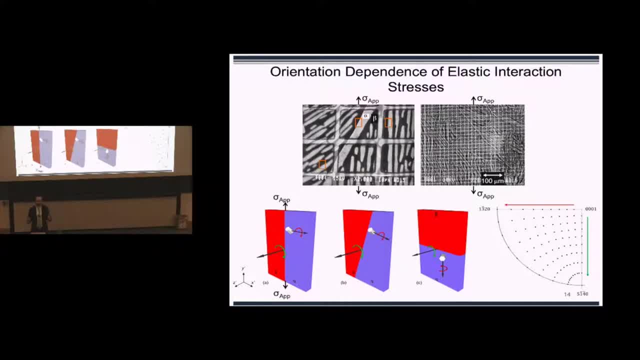 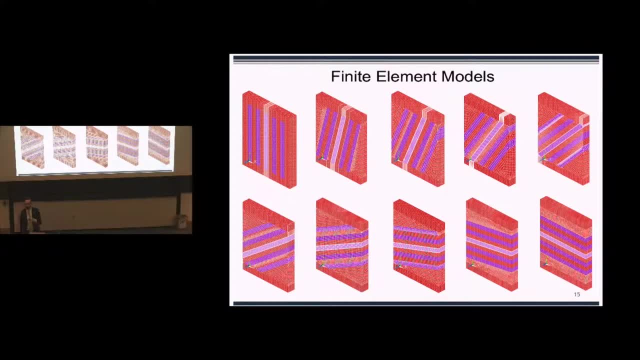 and it's telling me how things change with orientation space. So, specifically, what we do, there are a couple different options in terms of simulation techniques, but in this case we chose to use the finite element method, so we can just directly and explicitly measure microstructures. 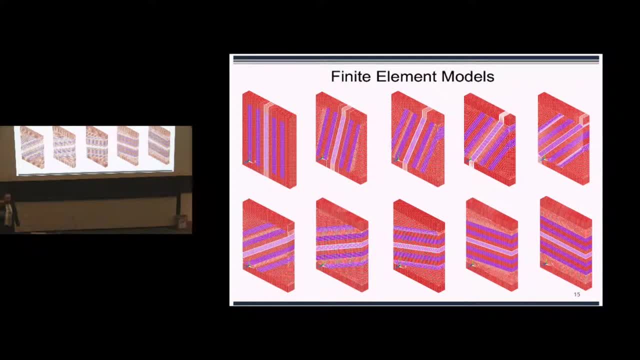 So, in order to capture the first degree of freedom, that change in the orientation or the interface plane, excuse me, we just literally build microstructures in ANSYS. So here you have them, from vertically oriented platelets- alpha platelets, to horizontally oriented alpha platelets, in ten degree increments. 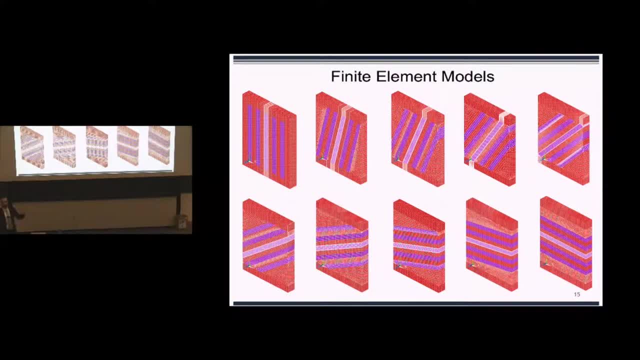 I'll point out for those of you who do finite element work, and those of you who don't do finite element work for that matter- you'll see this center platelet, very, very fine mesh. That's, of course, because we're particularly interested in 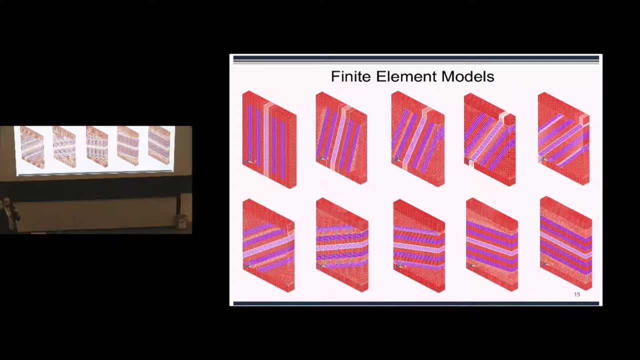 capturing the stress around that. But another key element here- this is a hard lesson learned- is that the mesh on the platelet for each of these is identical in every single simulation. We just take that mesh and rotate it by ten degrees and then we sort of you can see some of these. 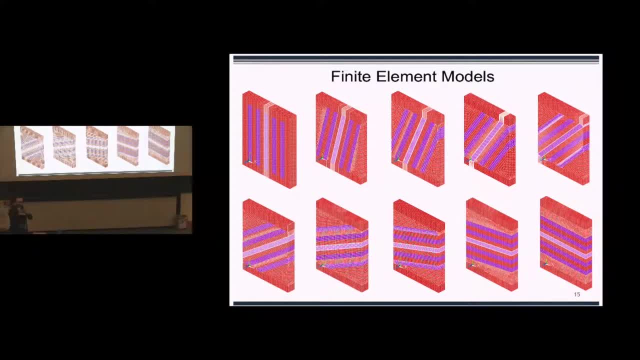 this is kind of I don't know what's going on here. it's a little bit weird. We basically force the nastiness of the mesh into the corners, away from the part of the model that we're interested in. however, is necessary to accommodate having identical mesh in every simulation. 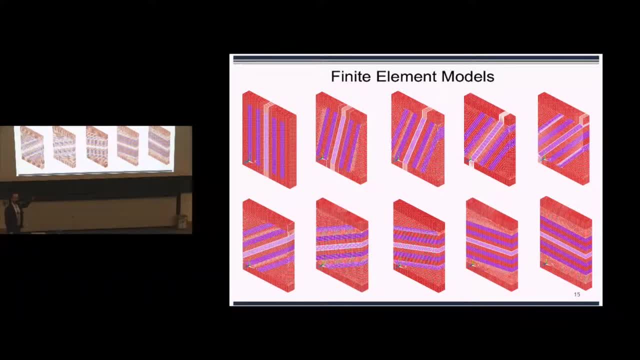 This means that mesh effects are gone. So that's the first degree of freedom, is the interface plane. The second one is the crystallographic rotation and the way we represent that here is we actually introduce the elastic, the full anisotropic elastic stiffness tensors for both phases. 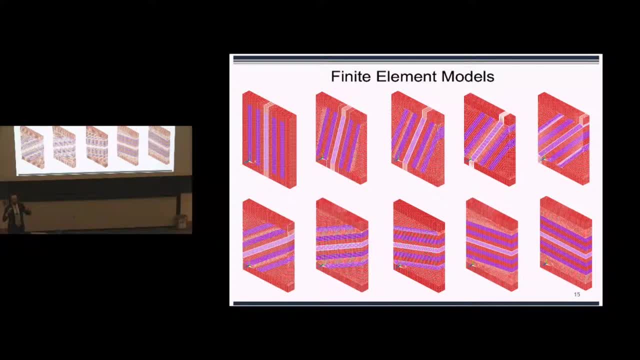 and from that stereographic projection we know what the orientation should be. we do the tensor rotation, we provide that to ANSYS as input. So this gives us 91 simulations that cover that whole orientation space. and again, the point here is that we're going to pull each of these elastically. 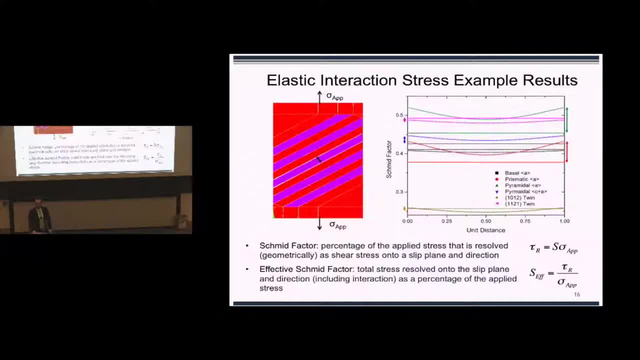 and we're going to look at how the stresses evolve and we're going to look at how they change and we're going to look at how the general structure of the interface changes. and we're going to look at the general structure of the interface. 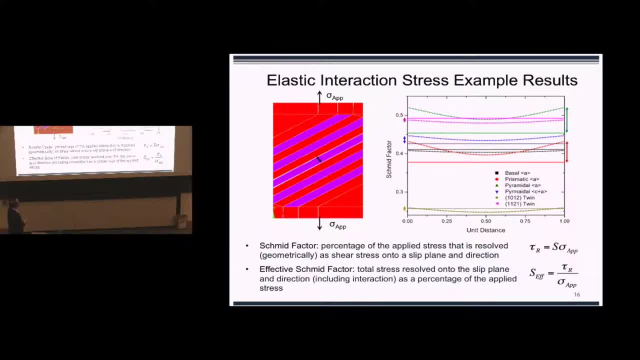 so let's take a look at one of those. I could show you all 91,. it would be a very long seminar, also not very interesting. So we'll just look at this first one before we start looking at things overall. So what you see here is I don't know whatever particular orientation this is. 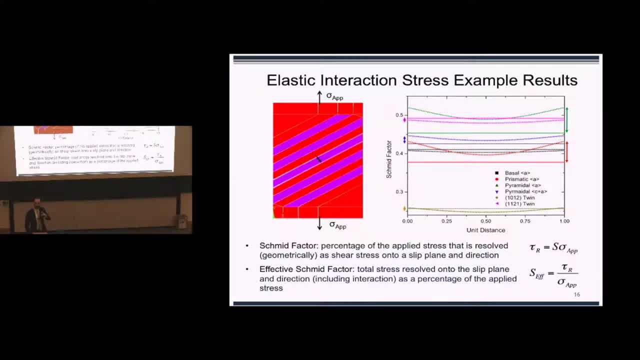 and what I'm looking at again is the stress from one side of the alpha platelet to the other side, And so I've plotted these results here to track where I am in orientation space. I can calculate without my model blind to finite element. 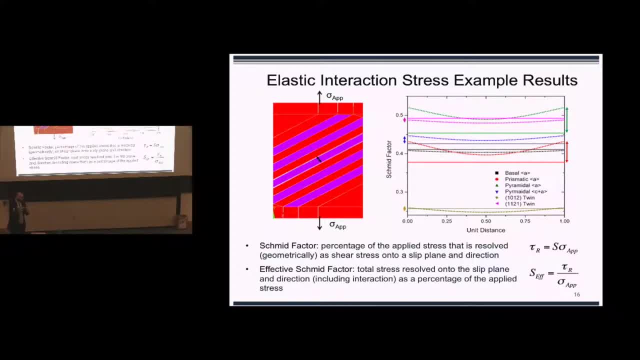 I can calculate the Schmid factor. I know where the basal slip planes are or the basal slip systems are, and I can calculate the Schmid factor onto those basal systems, prismatic systems, just geometrically, just from orientation. So what I get is these straight lines. 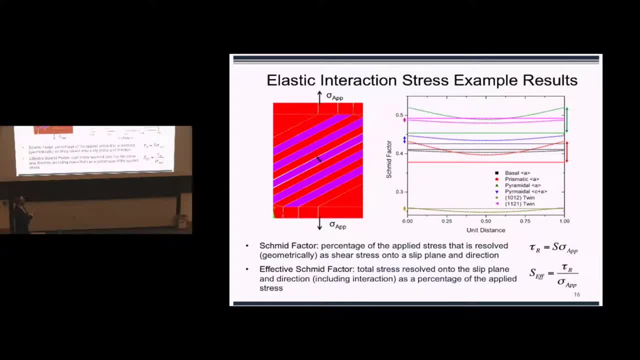 So, for example, I'll draw your attention to the prismatic slip system here. So this is the Schmid factor for this simulation on one of the particular prismatic slip systems. So again, the way you can read this is about 37% of the applied stress. 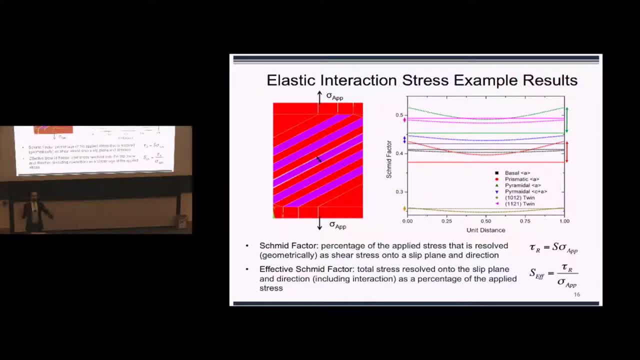 is resolved onto this prismatic slip system from a purely geometric standpoint. But what I can also do is I can take the stress tensor at every point along this line and I can resolve that from my simulation onto that exact same system And I can plot those results. 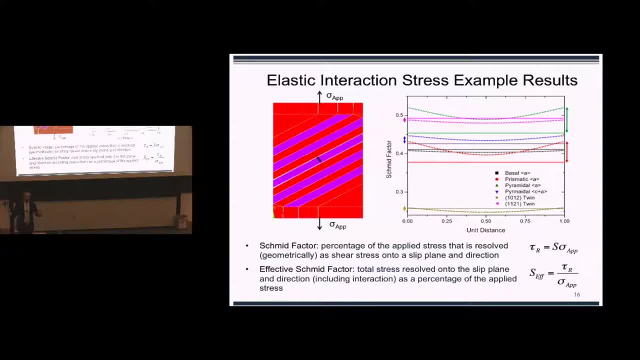 in these dots, squares, various orientations of triangle, And so the difference here is that that flat line, that smooth flat line, is purely geometric. It is the effect, it is the magnitude of the resolved stress on that slip system, due to the applied stress alone. 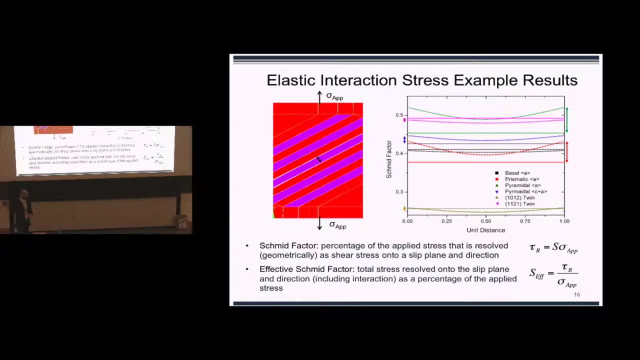 And my simulation results are the magnitude of the resolved shear stress on that slip system due to the applied stress and the elastic interactions. This is the elastic interaction stress that I'm talking about, And so what you can see is that in these simulations, in this particular simulation, 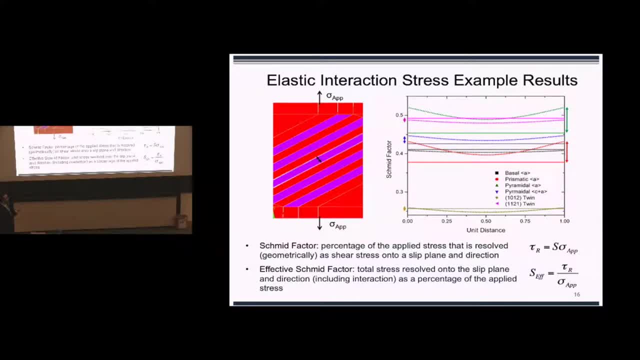 the elastic interaction stress results pretty strongly on the prismatic system, not really at all onto basal. It does some interesting things with reordering. So for example, if you did this just geometrically, you would think that basal would be the highest slip system. 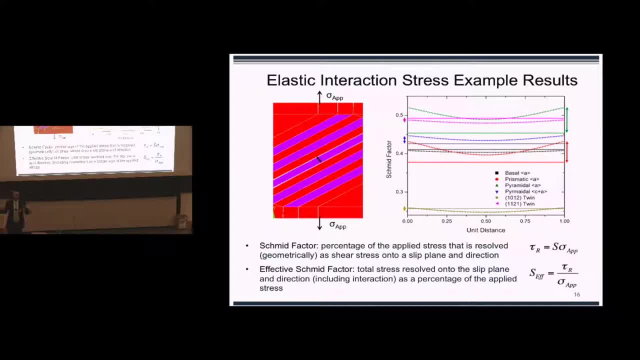 of these two. but in fact, with the interaction stress it's prismatic, So it moves the pieces around quite a bit. So now we see we have some evidence that these interaction stresses are significant. So let's try and map this onto the entire orientation space. 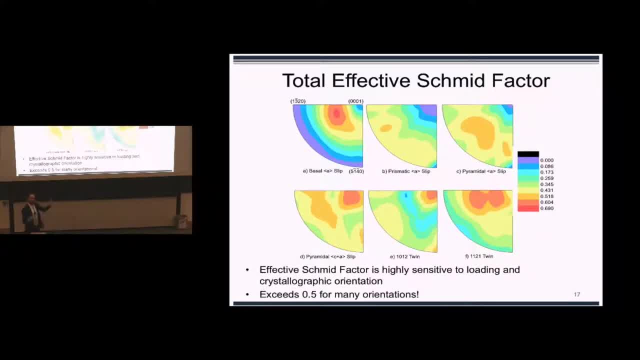 and see how things look. So here it is, and again, these quadrants represent all of the simulations You're looking at. results as a function of orientation, And so what I have first is the total effective Schmitt factor. This is the geometric 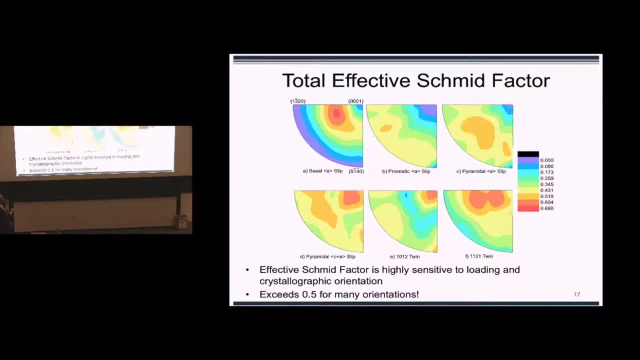 plus the interaction stress as it resolves onto each of these slip systems and the two twin systems, And so what you can see is two things. Two things jump right out. So if there was no orientation sensitivity, there would be none of these colorful contours, right? 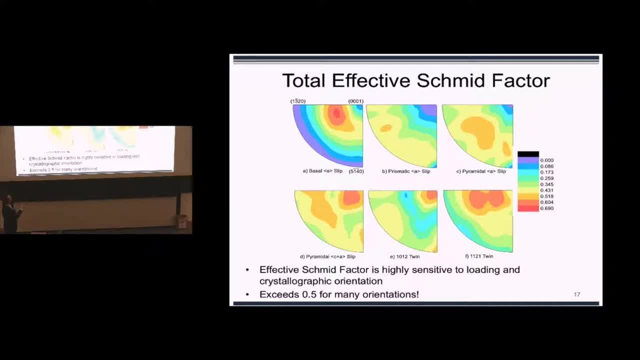 It would just be orange and blue and yellow. There's colorful contours here. So this tells you, for example, this particular orientation: with the interface plane oriented a certain way and the crystallographic structure oriented a certain way, there's suddenly a hotspot. 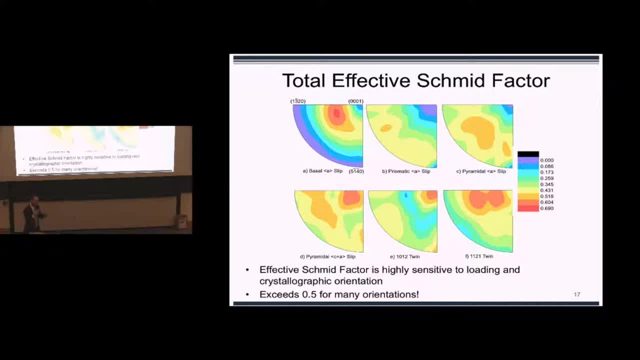 this high, high degree of resolution, of resolved and elastic interaction stress on that slip system. And another interesting thing is that the magnitude of this, when you add them up together, is much greater than 0.5.. I said geometrically it has to be 0.5.. 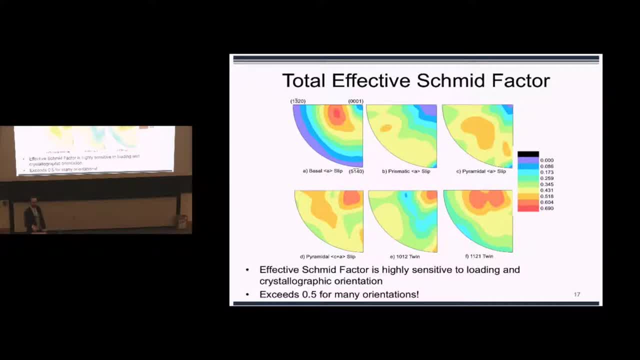 It can't go higher. It does go much higher because of the added contribution to these stresses. So again, if you think about Schmitt factor over dinner or in your free time, you might point out that, well, actually hold on. 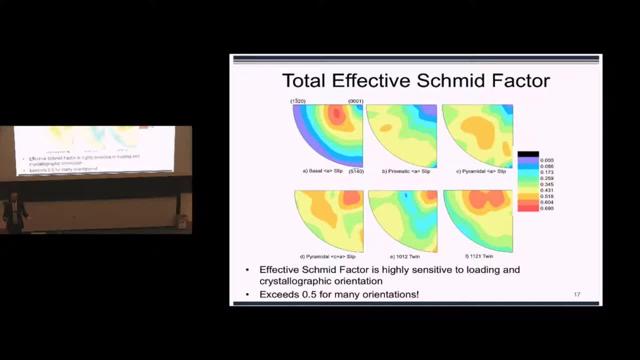 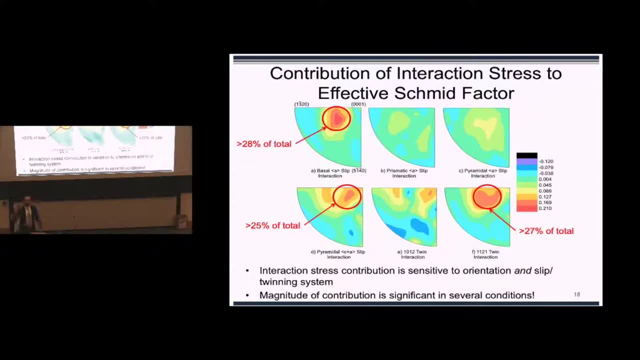 Schmitt factor is orientation, is naturally orientation dependent. It changes. It changes with angle. That's exactly how it's defined. So is this just Schmitt factor changing with angle? So what I can do is I can subtract the geometric part and look purely at the contribution. 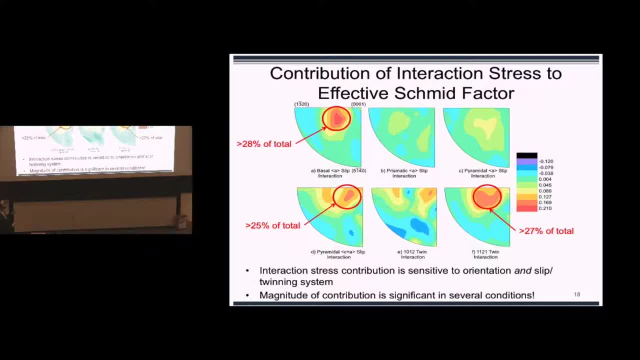 of the elastic interactions in this system, And so what we find is: so now, this has no geometric component, This is purely elastic interactions, And this has two to me. you know, of course, everybody's excited about their own research. 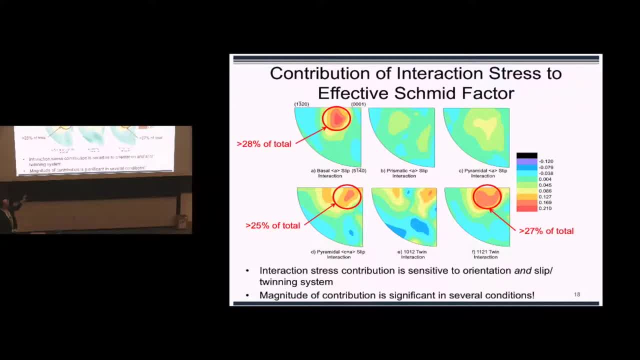 But to me- I look at this, oh, this is fantastic. So what we have is not only very strong orientation sensitivity in some systems, But only very strong orientation sensitivity in some systems: The prismatic slip system, which is a very common one. 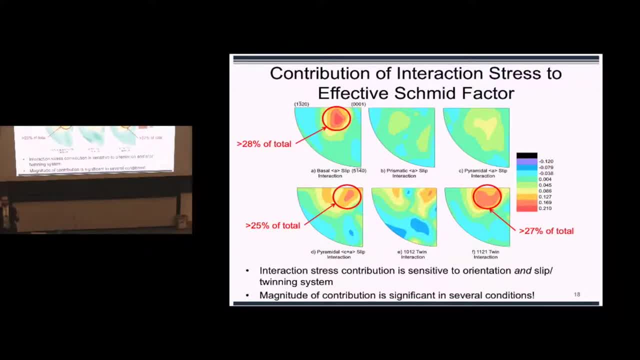 in titanium, basically just kind of along for the ride. as far as interaction stresses are concerned, Whereas the basal system has this hotspot, There's this node in orientation space where the elastic interaction is going to really push the dislocations along, And the magnitude of this is large right. 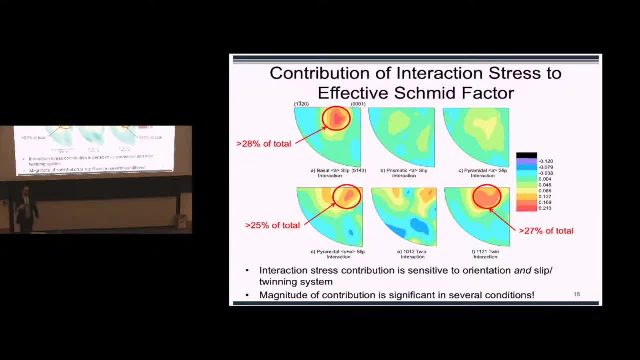 30% almost of the total stress that the dislocation feels in these orientations is from elastic interaction right The applied stress. The applied stress is only giving you 70%, So this is cool, I'm excited. Now the question is: and the question? 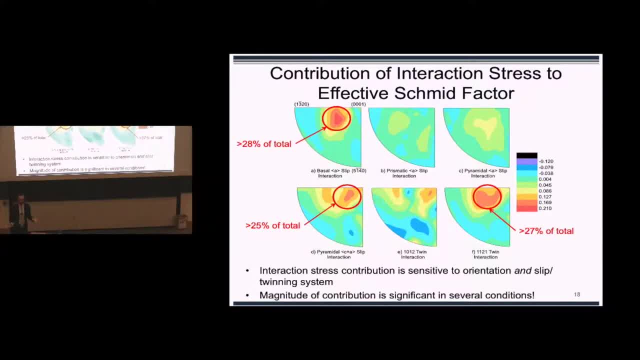 you should be asking yourself: is all right, neat model Will, Is it right? I mean you know it's simulations. Can we somehow investigate the accuracy, the validity of this model before we go forward and try and use it to answer the hypotheses I mentioned at the start? 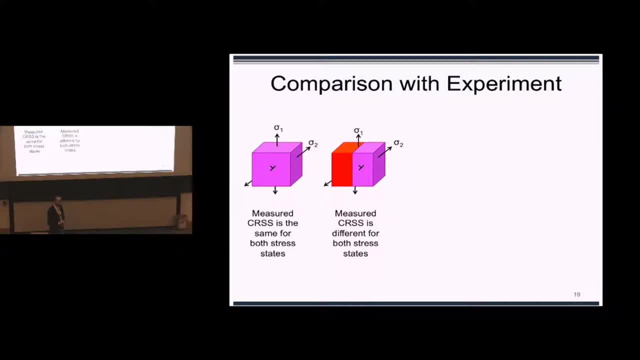 So the way we're going to do this is we're going to do a comparative experiment. It's a great way to validate a model, And the way I want you to think about this, the comparison I'm about to do- is the following: 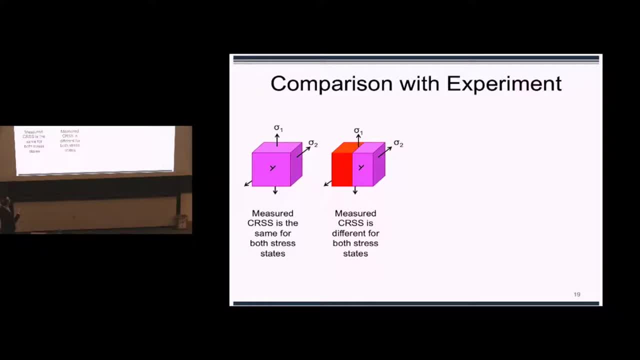 So imagine that I take a single crystal of alpha titanium and I pull it in one stress, I give it applied stress in one particular orientation and I measure the critical results- shear stress- And then I give it an applied stress in another orientation. 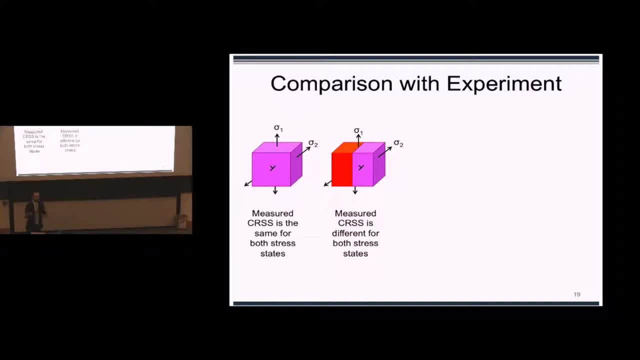 I measure the critical results, shear stress. It should be the same right, Because there's no interaction here. The magnitude of the applied stress will be different because it'll resolve differently, But the critical results, shear stress, should be constant. Now I just showed. 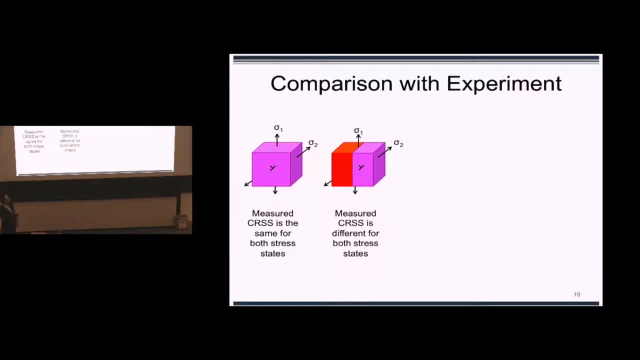 That the interaction stresses are orientation dependent, And what that means is that this test, sigma 1, versus this test, sigma 2, should give me different answers for critical results, shear stress. So if I can find someone, if someone out there in the world, 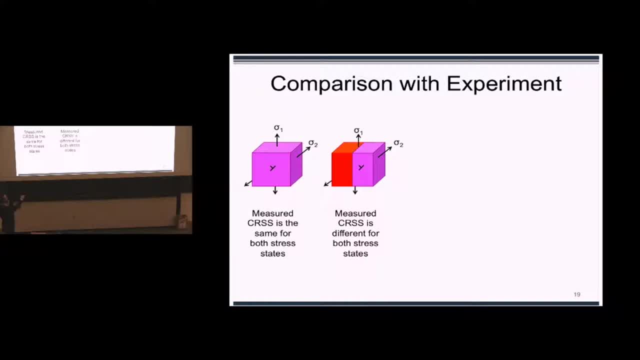 would run this experiment I could compare, would run an experiment where they carefully track the orientation of their systems, of these systems in titanium, and record the observed critical results, shear stress. I can compare that to my model And wouldn't you know? someone did that. 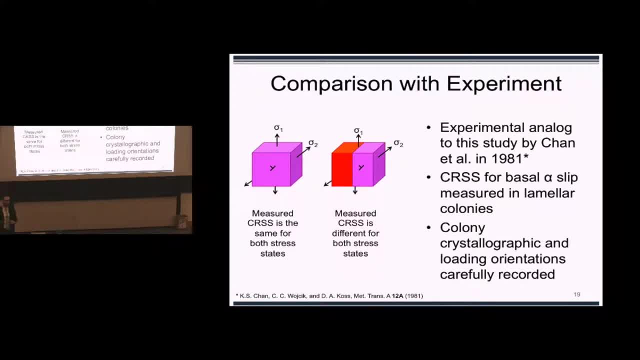 And they did it kind of a long time ago, Certainly before I was getting involved in titanium. So back in 1981, Chan and his co-workers at Stanford ran exactly this experiment, which I actually did not find until after I ran the simulations which 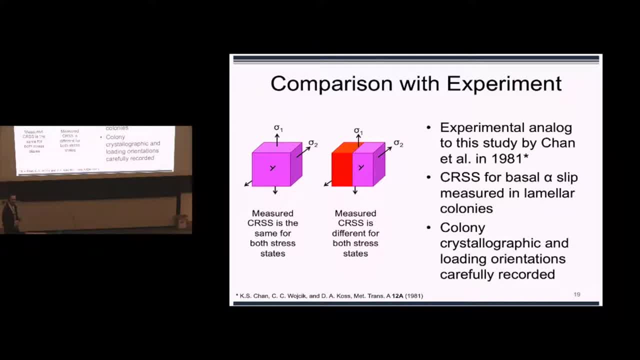 is such a wonderful experience. I can't tell you how happy I was when I found that. So they measured the critical results: shear stress for basal slip as a function of colony orientation. I'll point something out here that I thought was very interesting when I went through this. 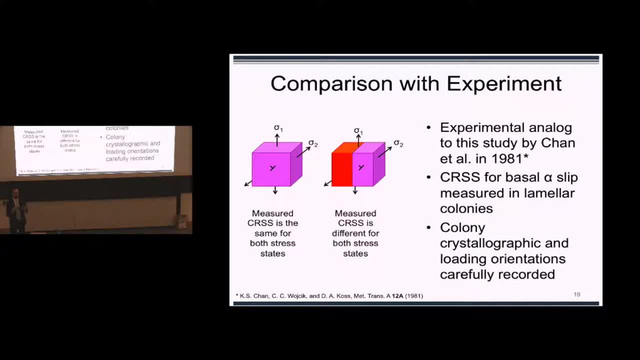 I'm. I'm personally. Uh, Uh, Uh, Uh Uh. I work very hard to maintain a good aesthetic in my publications. right? I like the figures to be very readable. I like the tables to be concise. This paper has a table that is horrendous. 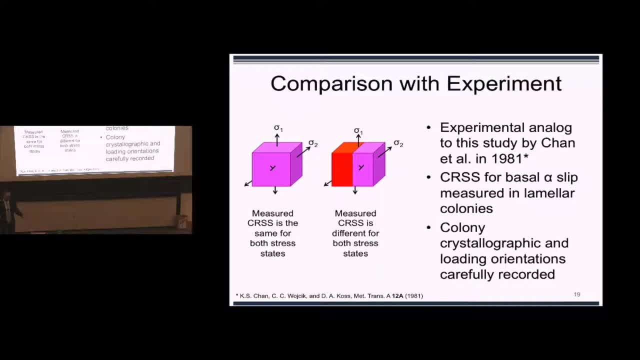 It's like 2 and 1 half pages long. It breaks up the text, You can't figure out where you are, And it is the only reason I was able to do this. So there's something to be said for thoroughness in your documentation publications. 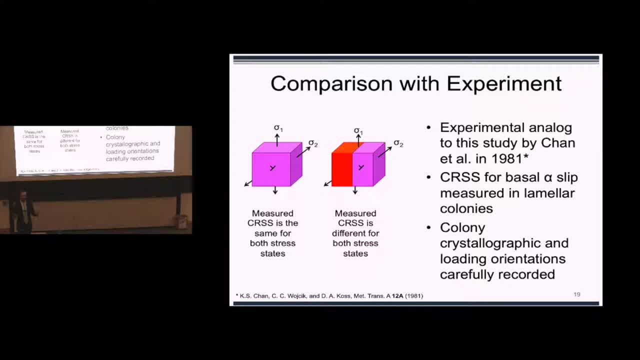 That table includes an incredible wealth of oriented information and a very, very depth of statistics. I mean, there's a lot in there And so I've never, I've never- met these folks. I don't, I don't even know where they are. 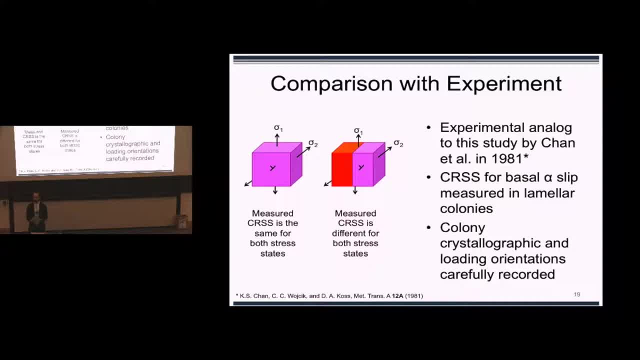 to be perfectly honest, but I was able to take their entire experimental data and just run right away with it because they were so thorough in their documentation. So there's something to be said for that, even in the, even flying in the face of aesthetic. 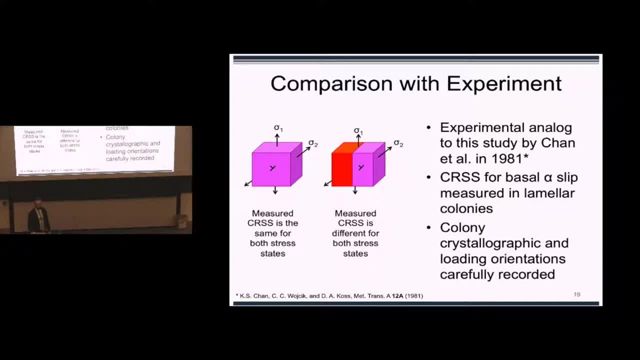 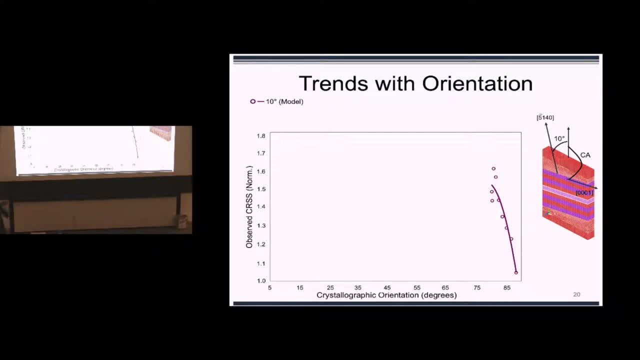 So a lesson there for me and maybe, maybe, for everybody, Anyway. So what I'm going to do is I'm going to show you a handful of plots that look like this, And so, before I show them, I'll explain this one, and then we'll kind of jump through the rest. 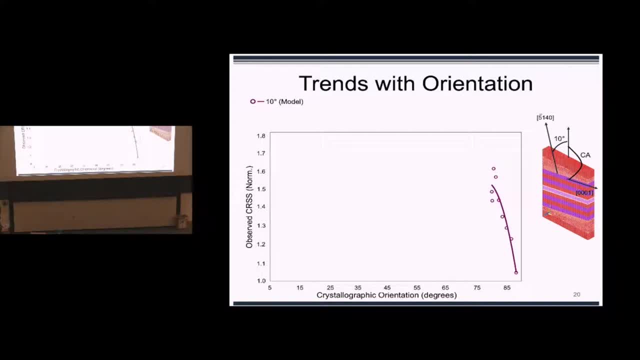 Because there are six or seven of them, I think. So what you're looking at here is a plot of the observed critical resolve shear stress. And so in the model case, this is the critical resolve shear stress. you would observe if the actual value 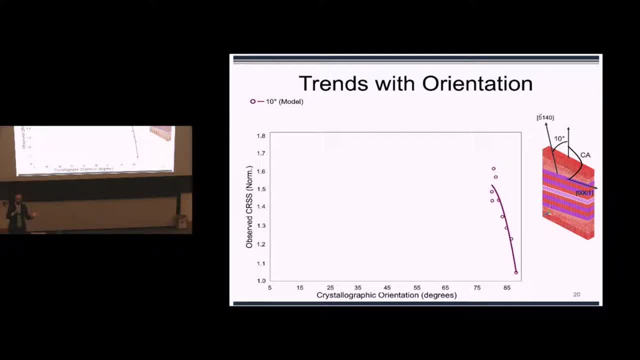 was constant for critical resolve, shear stress. But I account for that variation due to elastic interactions, And so in this particular case, I'm showing the 10 degree model. So this is where the interface is 10 degrees up from horizontal, And then each of these simulation results. 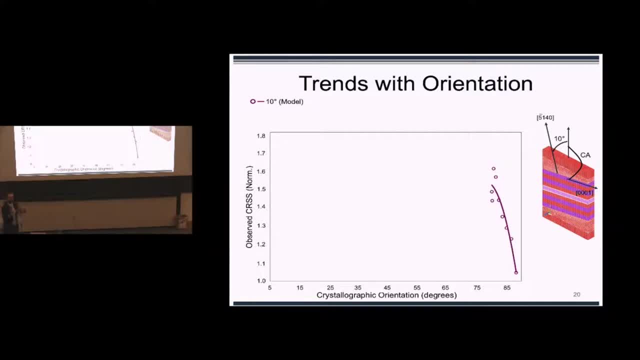 is for all 10 of the crystallographic rotations. So I have one interface plane, I rotate that 10 times And I get these simulation results. So already I have a range of observed critical resolve shear stress for this particular orientation: 60% or something like that. 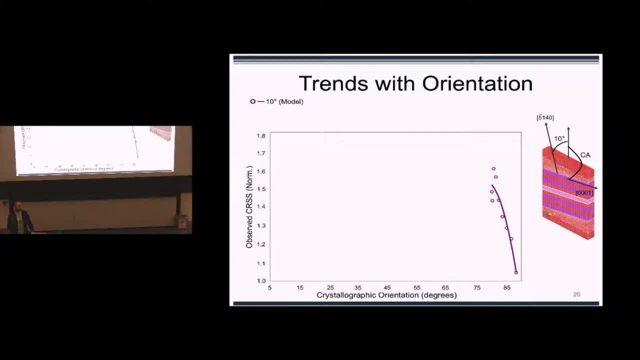 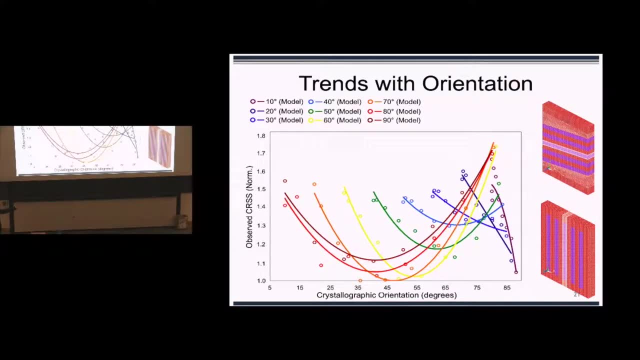 So there's something there. So now I can do this again, And this next plot's very colorful, I'll warn you ahead. So I can do that now And I can plot all of them on there. There's no experimental results here. 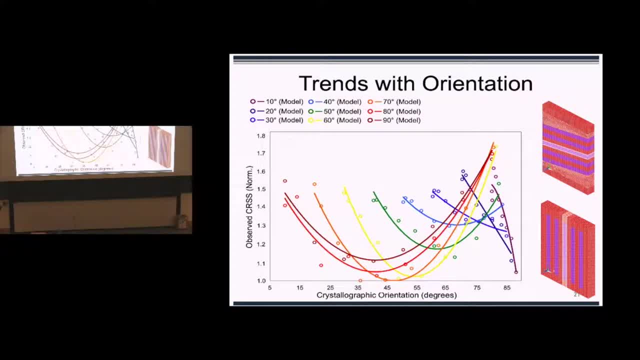 This is purely model, And the reason I show the results here is this. And the reason I show this is only because there's something systematic going on here, right? So you can see as I go from the 10-degree model to the 90-degree model. 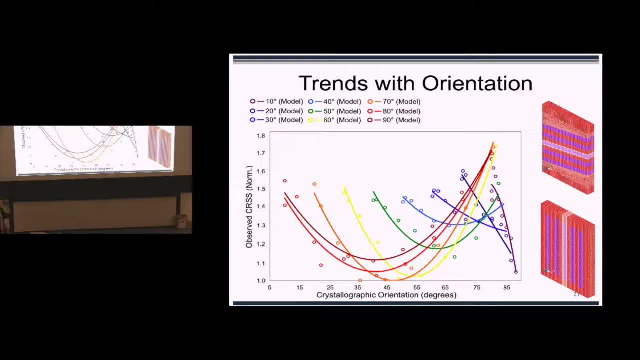 something is sort of happening with this response. I quite frankly don't fully understand this. I can't tell you a priori how to predict that kind of response, but it's comforting. in a way. It opens to me an opportunity for additional research, in so much as it is systematic. 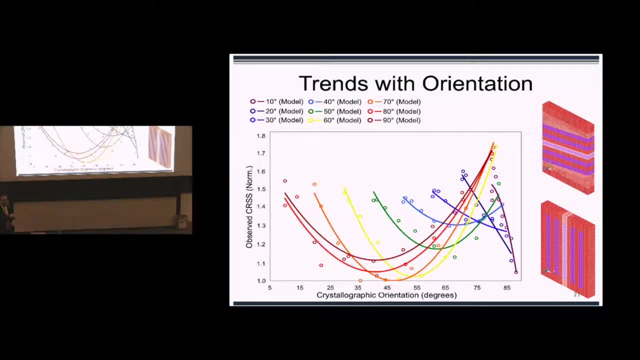 There's something here that's worth understanding. There may be a way to do this again without having to run 91 finite element models. That would be great, But in any case so this is how these results came out from a model perspective. 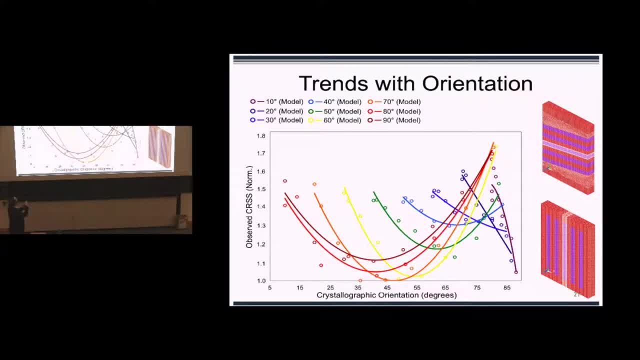 Now, in order to compare to experiment, what I'm going to do is I'm going to take each model orientation where Chan actually recorded data, So it's easy for me to run 91 of these. If you read through that paper, the experiment they actually had to do in terms of running. 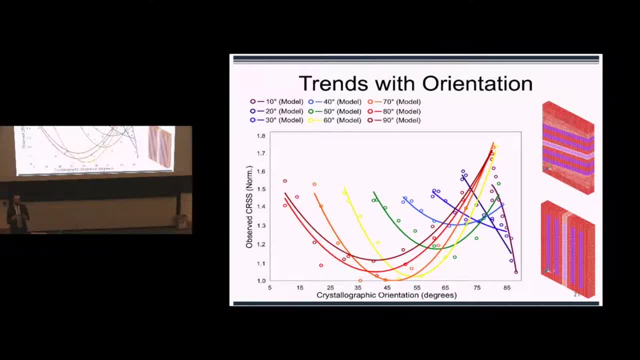 and Laue and diffraction measurements, all this business. they didn't get 91. They didn't. They didn't do all the orientations, So there's only some data. So what I'll show is each of the model results and each of the experiment results for one of these, 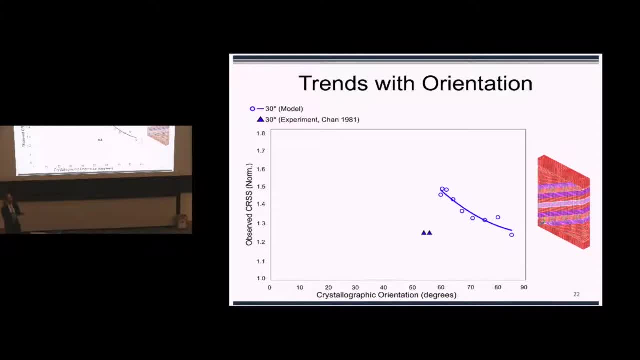 So, for example- here's the first one- 30 degrees. So my data is the dots and line Chan's data. the experiment is the triangles. If you're feeling very generous today, you could tell me that that's a good fit. 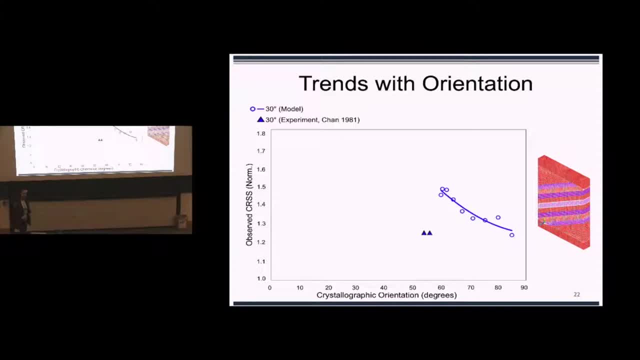 I don't personally think that it is, So we'll come back to this one. But that's the first, And so you plot these, You're doing the research, You generate the first plot and it's like: oh man. 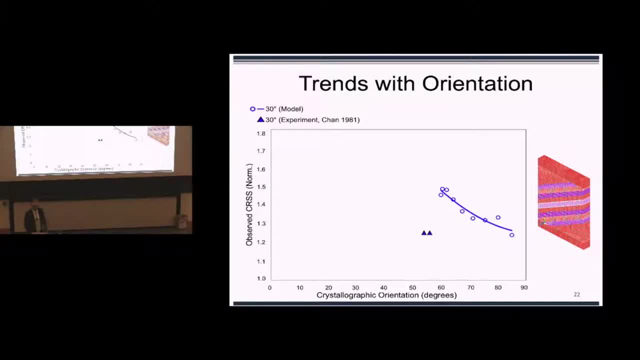 This is going to be a tough day, But then you generate the second plot. So there's nothing. Chan did not take any measurements or did not observe any colonies from 30 until 60 degrees. So here's my model and here's the experiment. 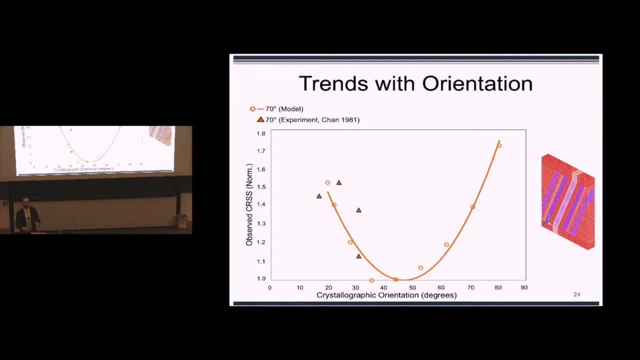 It's maybe feeling a little bit better. We'll go up to 70 degrees. Now we're starting to see some reasonable correlation between the model and the experiment. We'll go up to 80 degrees. Things are again looking quite good. 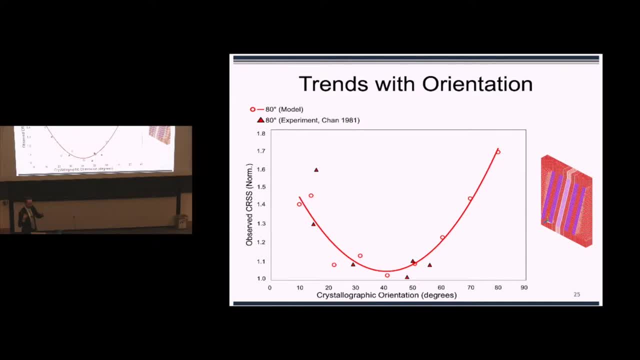 And I'll point out, I'll just mention for posterity, that I found this paper after the simulations. These data were done, So we have again a pretty good fit at 80 degrees and finally at 90 degrees. So you can see, in some of these there's really a pretty robust fit. 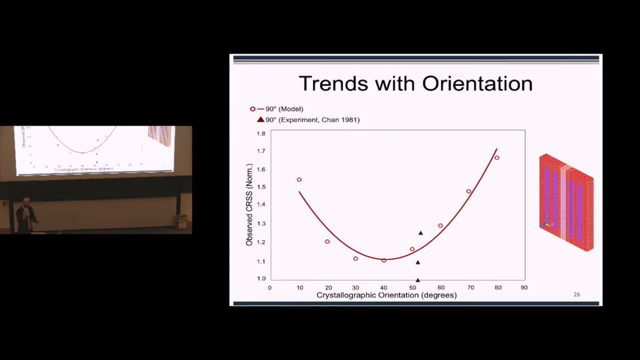 But I'm going to flip through them quickly one more time, because the piece that you don't see when I present the slides this way is these arcs are moving and that experimental data is moving with them, So let's go back here. So 60,, 70,, 80.. 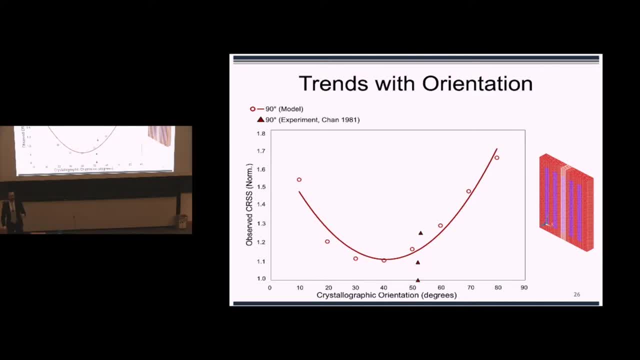 90. So we have so the 30-degree example. not a good fit, does not validate the model. I'm okay with that. So there's something going on at those lower angles that we don't understand, or I messed up the model, or there's something wrong in the experiment. 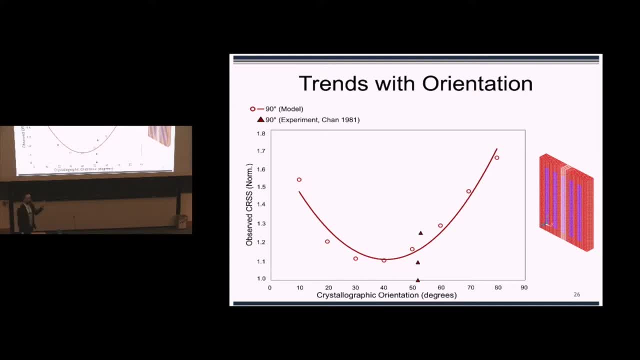 There's work to be done there, But at these higher angles we have really a fairly robust fit or relationship between the experimental and model data. So this actually helps answer. the first one of those hypotheses Is the interaction, is the elastic interaction with the beta. 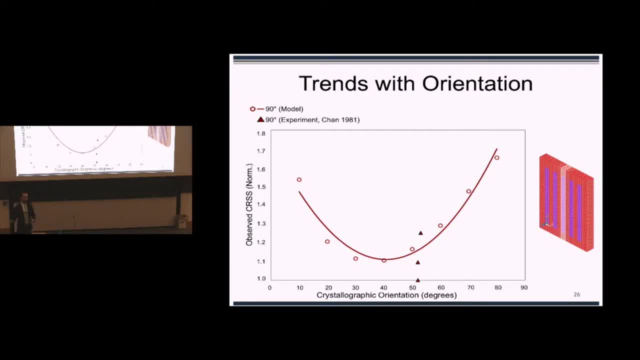 responsible for that variation in critical resolve, shear stress that we see- And I think that based on this it is, or it largely is- We see strong correlation. I'll flip back to this one because it looks better, But we see strong correlation between the predicted variation. 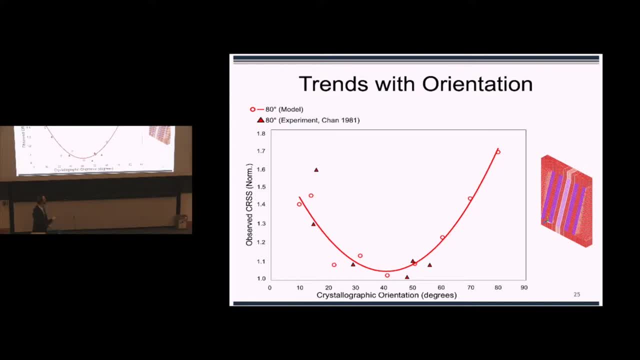 in critical resolve shear stress due to the elastic interactions and the measured variation in critical resolve shear stress due to who knows what, And so this tells us that any other contributions that are also affecting this variation in critical resolve shear stress, of which I'm sure there are some, are relatively small. 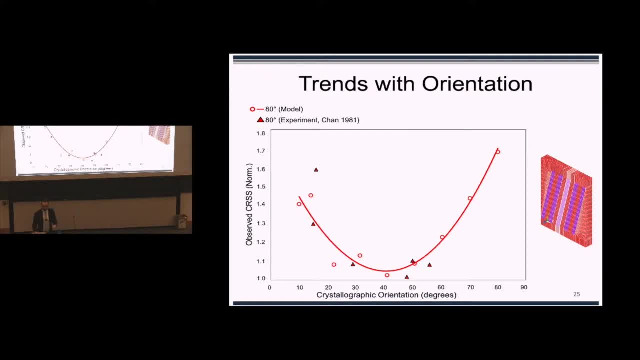 compared to elastic interaction. So that's the first piece. The second piece is this question about twinning. So I mentioned we've kind of talked about dislocation slip here. So is this elastic interaction responsible for the twinning that we see? And so the way that we looked at this was the following: 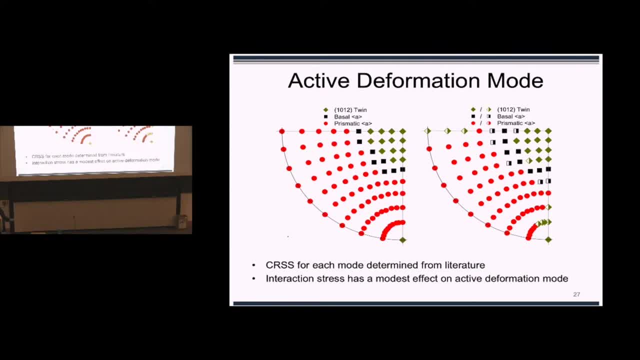 I'll sort of do this easily on one slide, So I can take the reported critical resolve shear stress for each of these deformation modes from the literature, and then I can go for every single one of my simulations. I can calculate what is the resolve shear stress. 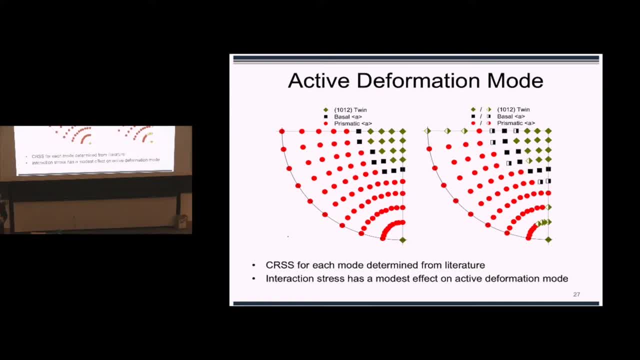 on every single one of them, And then I can do a little deformation system And I can say as I increase, increase, increase, increase stress, which one's the first that I hit Right, That's the mode that would be active in that orientation. 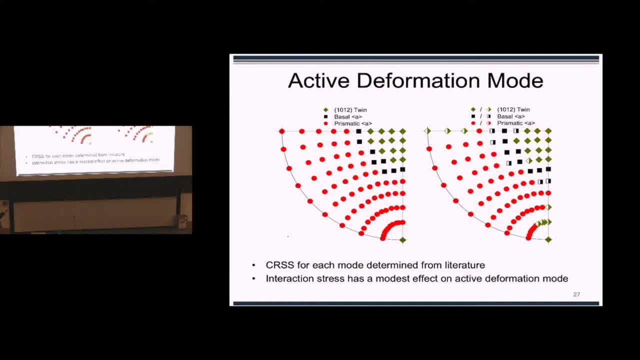 So that's what I've done here, So you can say I have twinning near the poles. I have a little stripe of basal slip and then mostly prismatic slip And, for those of you who work in particularly low, aluminum titanium alloys. 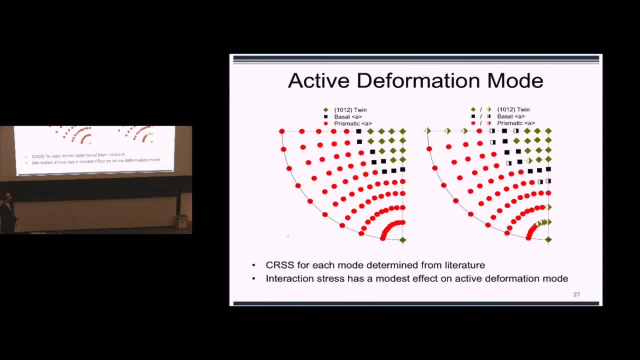 you see, mostly prismatic slip, but a little bit of twinning. So that's good, That feels nice. So this is purely geometric. And now what I can do is add the effects of elastic interaction stress, which I've done here. 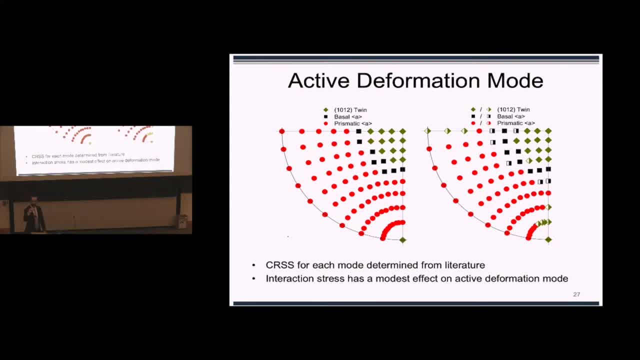 And those symbols that are half full are locations where the deformation mode switched because of the elastic interaction, And so what I see is a few locations where the deformation mechanism switches to twinning, a few locations where the deformation mechanism switches to basal slip, and this is where I leave it to you to decide. 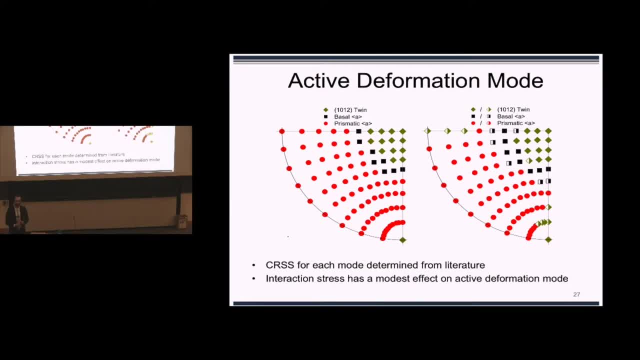 whether or not these interactions are actually responsible for that twinning. I will tell you that, since having finished this and kind of being involved in the community that works on twin nucleation and twin mechanics, I think the answer is no. I don't think that this is enough to fully explain. 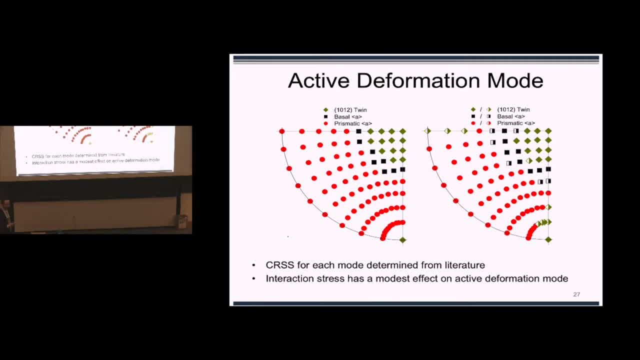 that twinning behavior that we see. We'll talk a little bit, I think actually in the next slide, about what it could be. My advisor thinks the answer is yes, So we agree to disagree. That's okay, So anyway. so let's wrap up this elastic interaction stress. 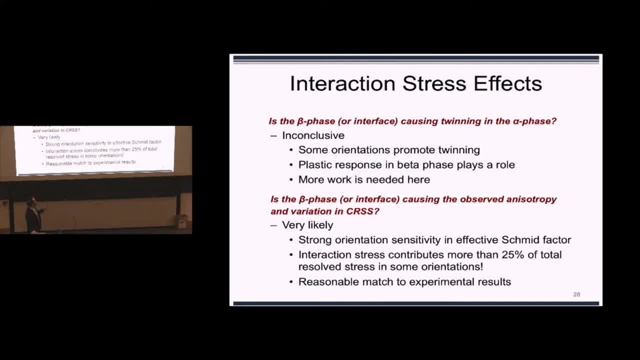 and we'll jump into some oxygen stuff. So, again to summarize, here is the beta phase causing twinning in the alpha phase. I'm going to give my advice. I've been fairly doubtful, calling it inconclusive. Really, the key here, though, is this middle bullet. 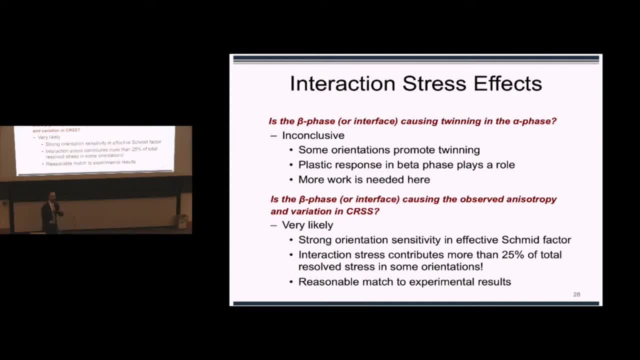 Plastic response in the beta phase has to be playing a role. in my personal opinion, Twinning when a twin forms it is a massively voluminous thing relative to dislocation and the tip of that twin generates very, very large strain fields. 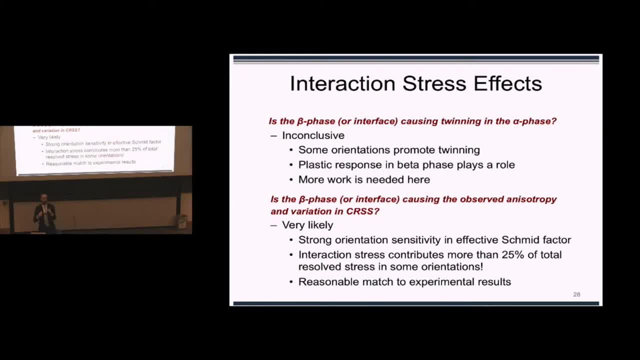 And if the tip of that twin is sitting against beta, there's been more recent research that suggests it must plastically deform beta. So the ability of beta to accommodate that plastic deformation has to be formed. It has to be playing a role. This is a perfectly elastic model. 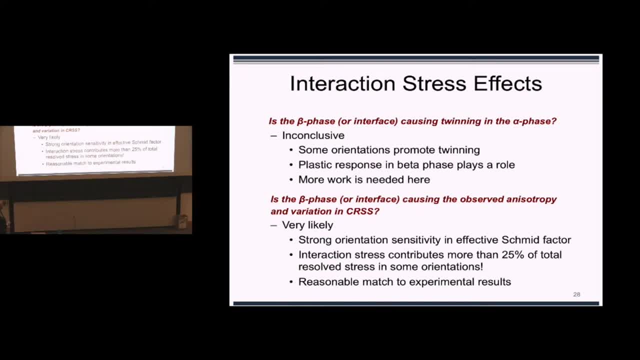 so I don't think we get there, But we've learned something In terms of: is the beta phase causing the variation in CR, critical results, shear stress as a function of orientation? I think it is. I think that the fit between the experiment and the model. 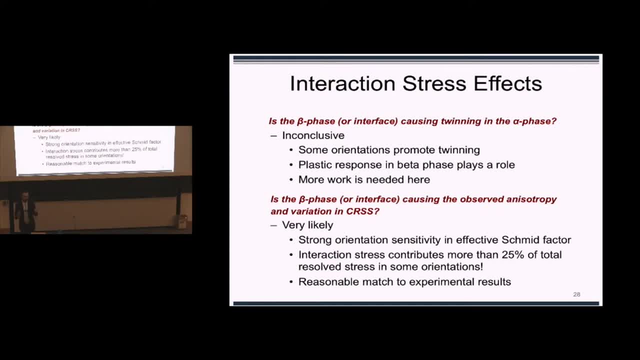 for the high angles is very good, considering what we did, Not just just period, And I think that that tells a story about the importance of these interactions. Still have to figure out that 30-degree test. I don't know what to tell you. 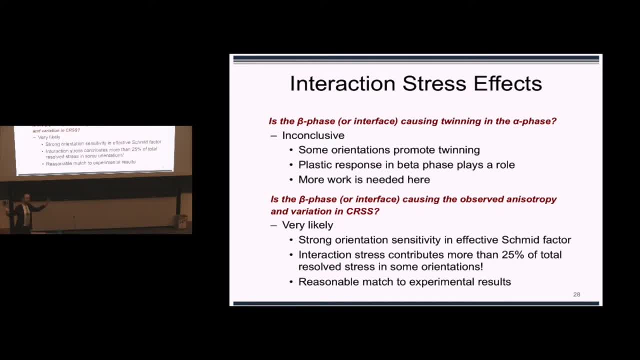 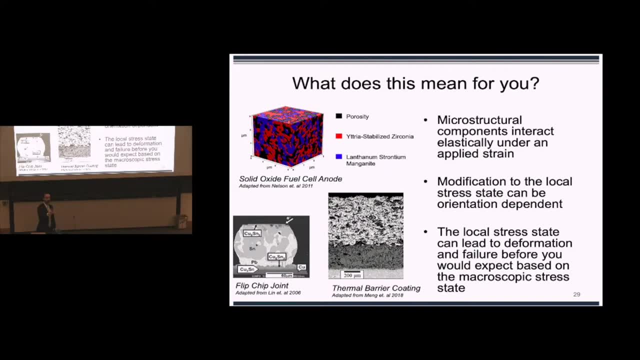 It's worked out. Work to be done. Okay, So we've gone all the way down to the bottom. on elastic interaction stress. I want to bring it back up before we leave this and talk a little bit about what this could mean for you. 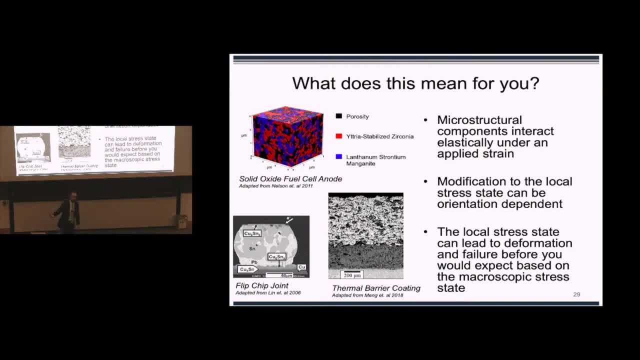 for your research, Unless you've been sneaking in the background of the field. I am not aware of anyone in here who's doing this sort of work in titanium, But I know everyone in this. well, not everyone, excuse me, But I know there are many, many people here who are doing work. 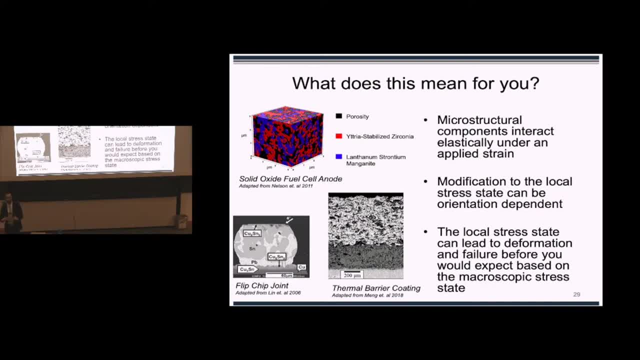 that involve deformation of materials, mechanical behavior and microstructures. So, in those cases, what I want you to take a look at is: take away. what I want you to think about in the application of your own research is: how do these the interaction? 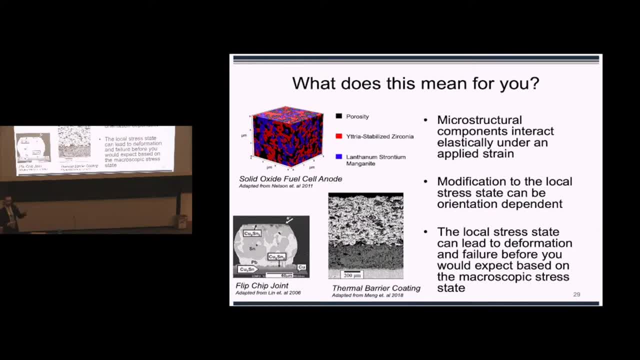 of multiple phases and complex microstructures. this could be in mechanical systems, like I showed, functional systems like fuel cells, flip chip joints, thermal barrier coatings. all of these systems and many others have microstructures that interact elastically when they're loaded. 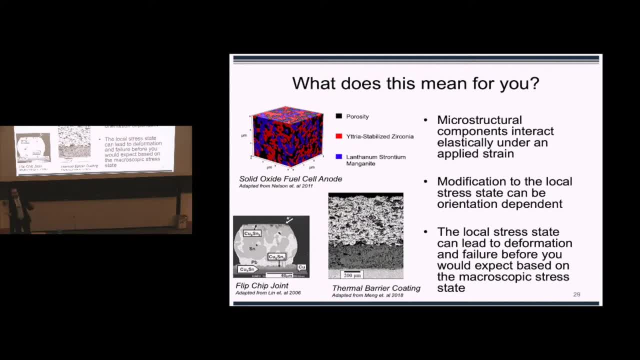 So you probably don't like think about this right before you go to sleep at night, but you're aware intuitively that there are elastic interactions. I don't think I Reveal that to you necessarily, but the thing that I want. 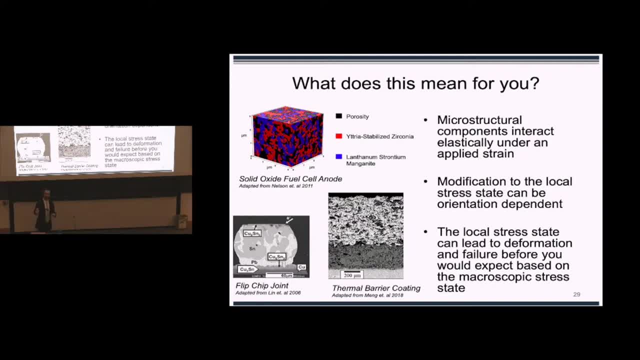 to highlight that might be maybe you haven't thought about is that those elastic interactions can be highly orientation sensitive and that this can lead to a local stress state that causes deformation, failure or fracture, or something well before you would expect, based 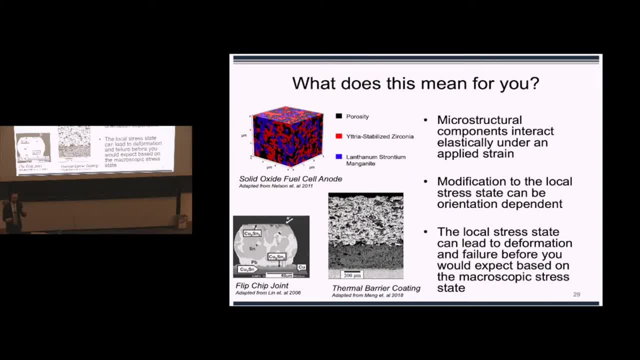 on the applied stress alone. And the last thing, before I switch off of this topic, I've kind of couched this as a: it's a bad thing, these interaction stresses are detrimental, but there may be other opportunities here You can imagine, for example, 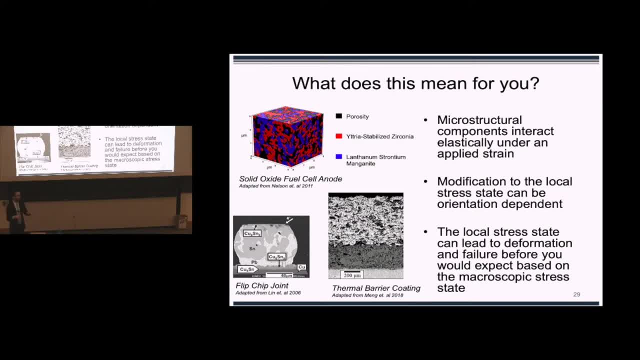 a battery anode. well, let's not use a battery anode. let's use a TBC thermal barrier coating in a jet engine. So as the jet engine heats up and cools down that thermal barrier coating is on a substrate, it bends. 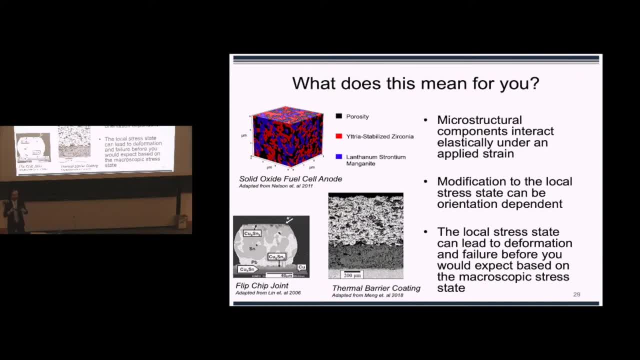 and unbends, it bends and unbends. that stress state is relatively repeatable. it's actually a relatively simple stress state as a function of time. Could I imagine orienting my microstructure using these elastic interactions, knowing the directionality of that stress state, to either stay away from hot spots? in elastic interaction space or, even better, introduce cool spots. I didn't talk about them too much, but there are places where the elastic interaction is actually negative enough. Could I use that to my benefit to actually give me a little bit of added durability? 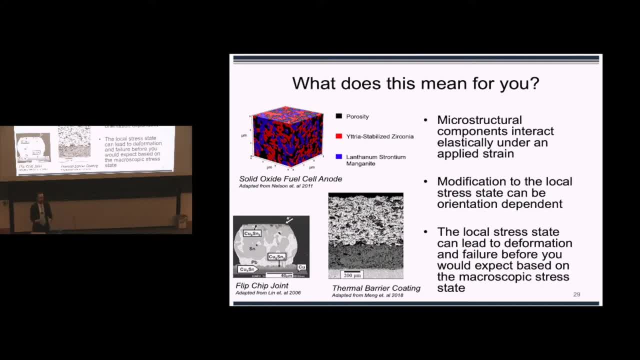 In titanium? yeah, I think you could. You've got to figure out how to deal with the texture and how to make that happen, but maybe in some of your systems you can too. So something to think about. Maybe it's helpful, maybe it's not, but I hope it is. 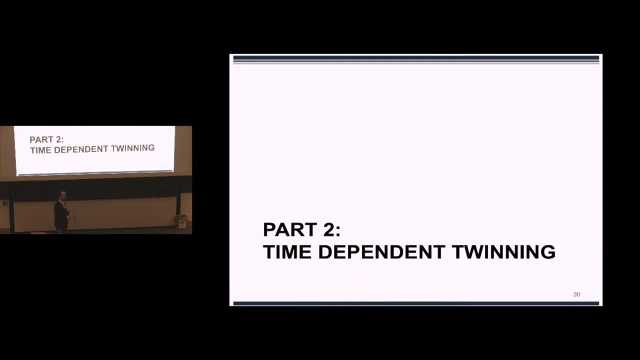 Okay, part two. this one's much shorter. I do want to talk, then, about the oxygen interstitial effects and time-dependent twinning. So again, there's a question of how to. how is twinning a problem? How is twinning a creep mechanism? 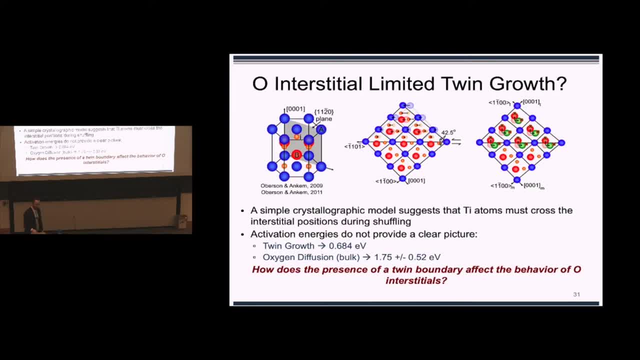 Twinning happens at the speed of sound in the metal. This couldn't be possible. So several years ago, Marilyn, before my time, there was some work looking at the impact of oxygen interstitials and twinning in titanium, And so basically what Greg and my advisor did was they made some. 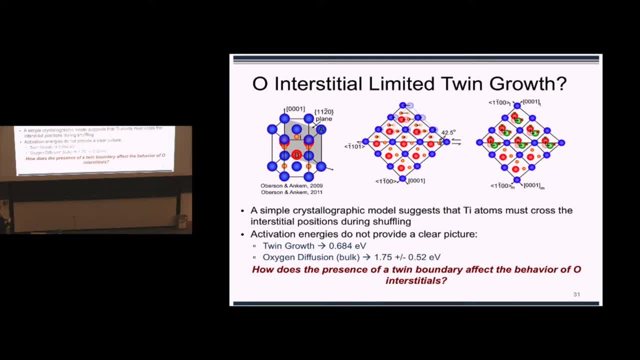 ball and stick models. right, these are not atomistic simulations of titanium. And they said: hey, look at this. So in the titanium lattice we have titanium atoms in blue and red, in the alpha, beta or A and B and A sites. 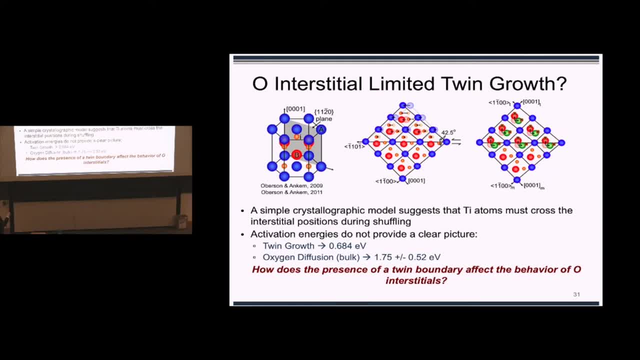 right the stacking sequence of the HCP, And then we have these oxygen interstitial sites in I. So if I line this up so that I'm looking at one of the particular twin planes twinning an HCP, atom almost always happens as a two-step process. 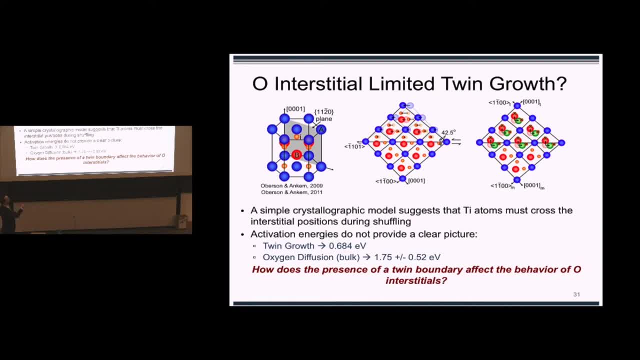 So the first step is a shear. So there's a. it's a homogeneous shear, which means that every single atom in the system shears the exact same amount, has the experience of the exact same shear strain. But it turns out you can't get the exact same shear strain. 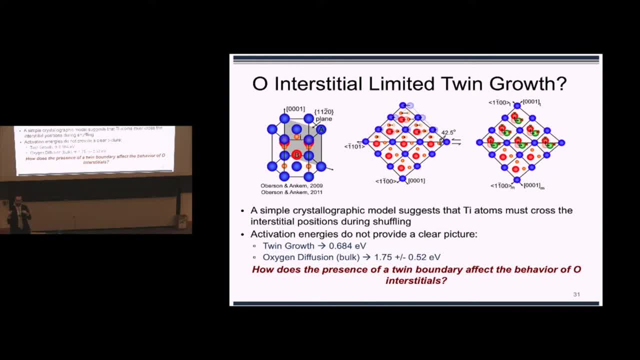 get the atoms quite into the right shear- excuse me, lattice positions using a pure shear- unless the C to A ratio is ideal, which it's not in any of these. So there's a second step in twinning that's called shuffle. 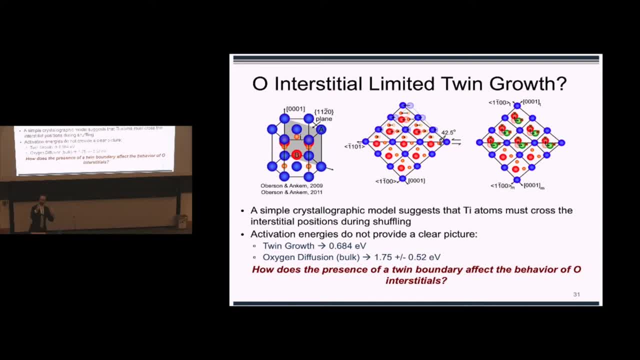 So first the atoms shear. they're almost in position, but they have to move just a little bit and they shuffle. And the shuffle of these B atoms crosses the interstitial sites In order for the B atom to get to its final location. 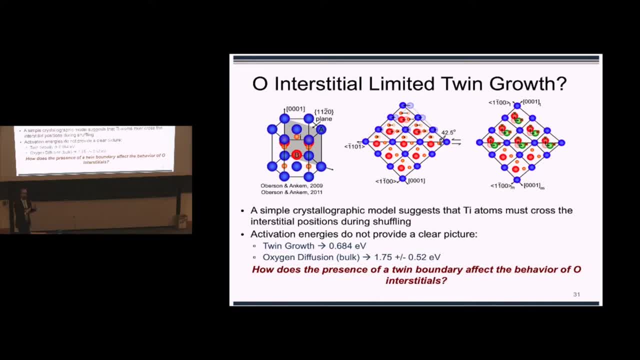 it has to get across an oxygen interstitial, And so what Greg and Dr Inka thought was: hey, if there's an oxygen interstitial site, it can't- or it just can't- make that transition, And so the twin gets stuck. 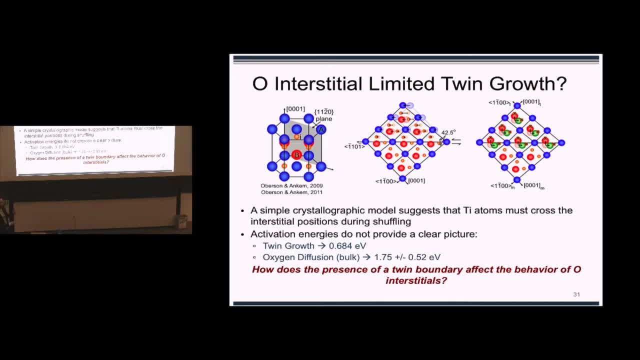 and you have to wait for oxygen to diffuse away. Great idea. it was a good publication. The one downside was this: The activation energy that they measured for twin growth was like 0.7 eV, and the reported activation energy for oxygen diffusion was 1.75, so they're different by a lot. 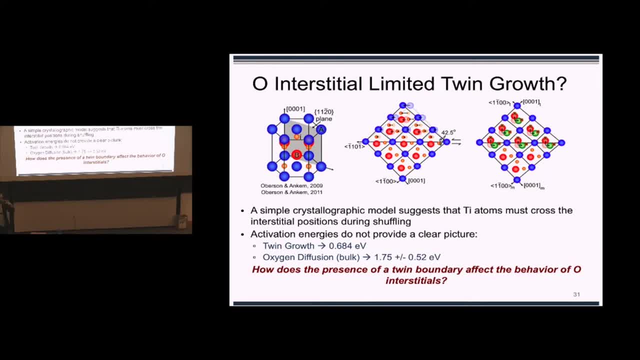 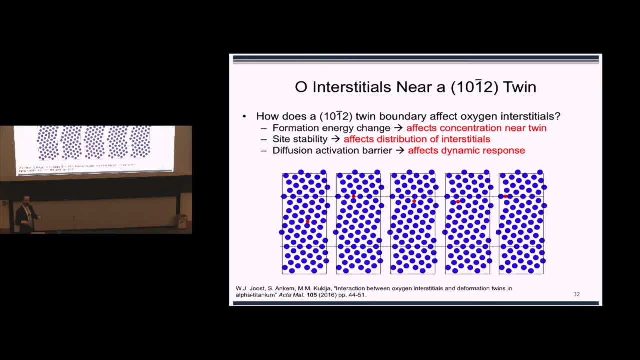 So it maybe isn't so simple, as you wait for oxygen to diffuse and then the twin grows and you wait for oxygen to diffuse. There's gotta be something else here. So what we did was approach this using computation, material science tools. We'll talk about specific tools here in a sec. 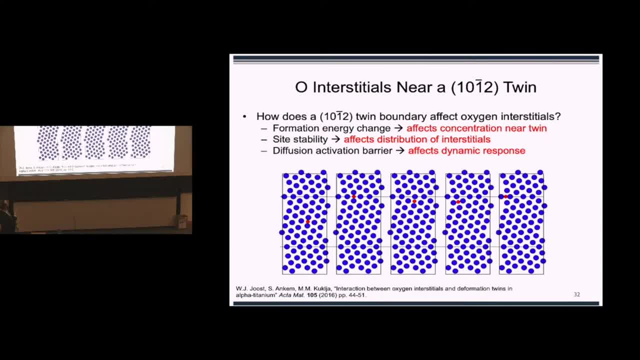 But the basic idea is we wanted to calculate three things: Formation energy of these interstitial defects near a twin. If the formation energy goes down, that means the free energy of the system when it forms these defects goes down and you would have a preference for oxygen interstitials. 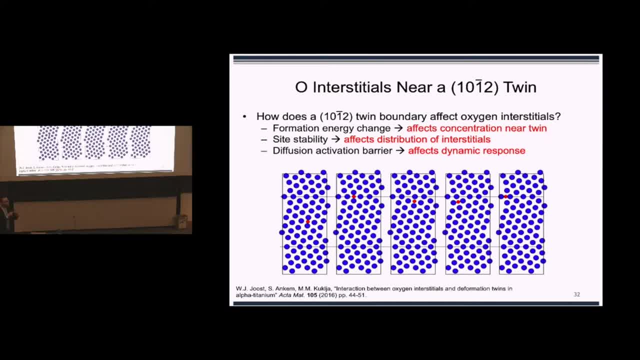 to form at the twin, so that we wouldn't get you know. Site stability- where can oxygen actually live in the lattice? And then, importantly, diffusion barrier. Right that 1.75 eV, that's in the bulk. No one measured it at a twin. 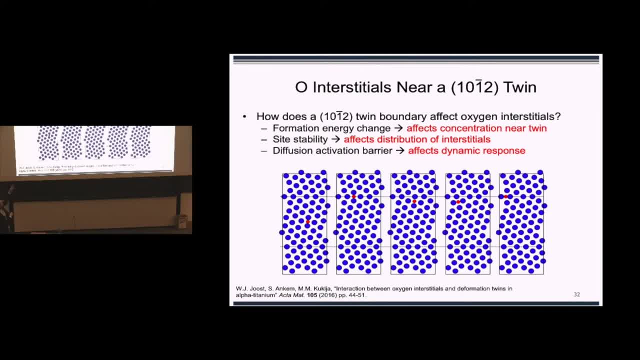 I don't know how you would. it would be very difficult. So the question was: can we calculate these three features: formation, energy site stability and diffusion activation barrier for oxygen interstitials near a twin? I'll point out if this is something. 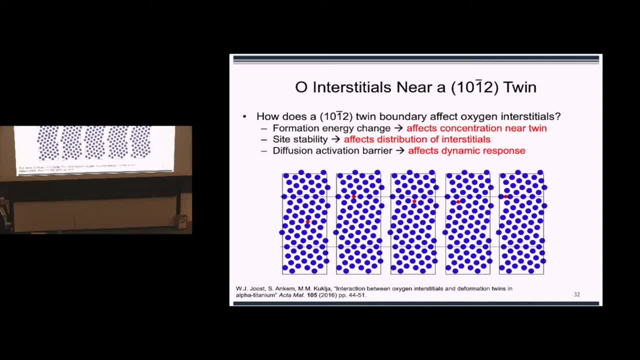 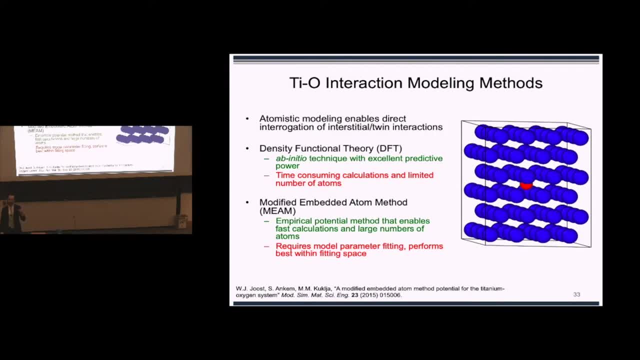 that gets you really excited, and I hope it does. you can find our paper in Actomat a few years ago, but it's still good. So the computational techniques that we used here were twofold, so we stuck with atomistics, right. 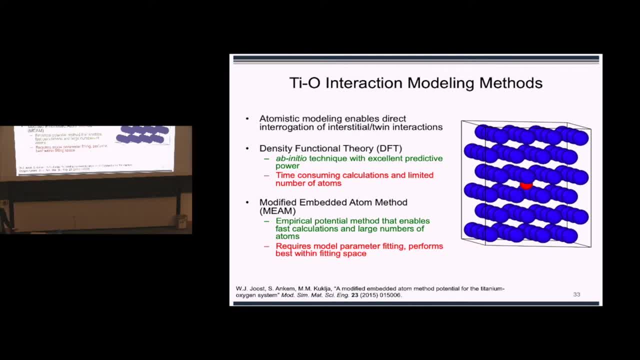 We're interested in studying how the atoms interact. so we're just gonna model the atoms explicitly. We're gonna do that two ways. We're gonna use what's called density functional theory. This is an ab initio technique. It's if you look at the equations. 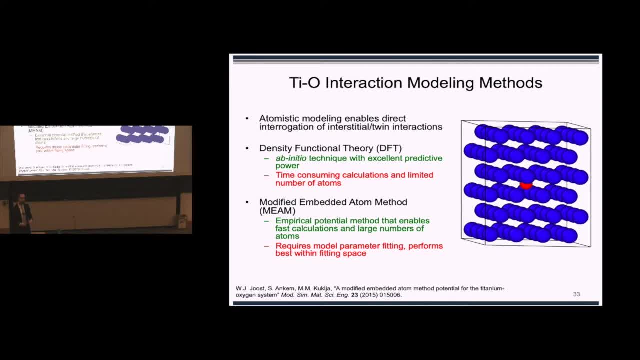 they look sort of like Schrodinger's equation. They aren't technically the same. But the nice thing about density functional theory is that it's sort of a parameter-free model. For all intents and purposes it is parameter-free. I don't have to fit anything. 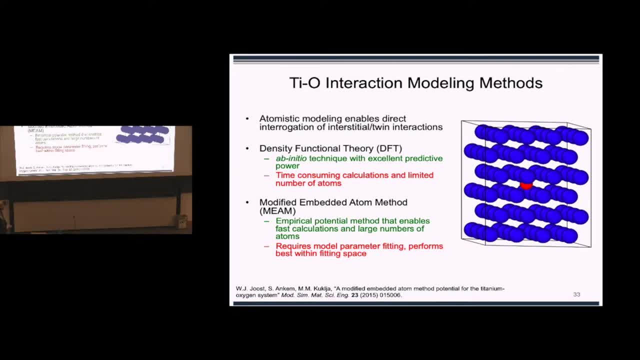 I can just put the atoms in the box and let them relax and get some kind of. The bad thing is that it's very, very time-consuming. These are expensive calculations. So in addition to this, we used the modified embedded atom method. 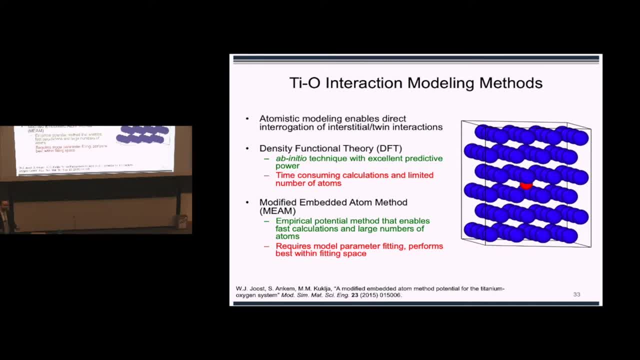 This is an empirical potential method, so it's lots of parameters you have to fit, But it's very, very fast. Unfortunately there was no mean potential for titanium and oxygen, so we had to fit one. So this is published in MSMEA, MS, MSE. excuse me. 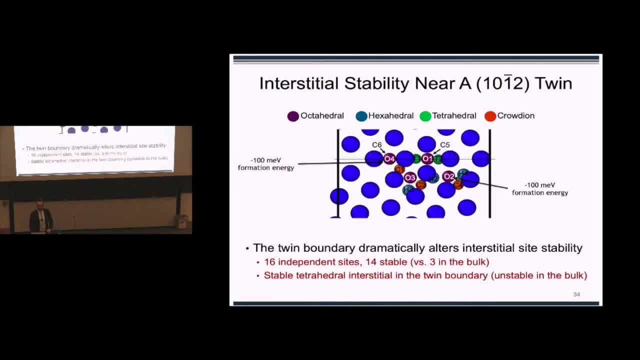 And so if you wanna simulate titanium and oxygen, you'll get it Anyway, okay, So the first thing is site stability and formation energy. So what we do is we take a twin, so you can see we have a twin boundary here. 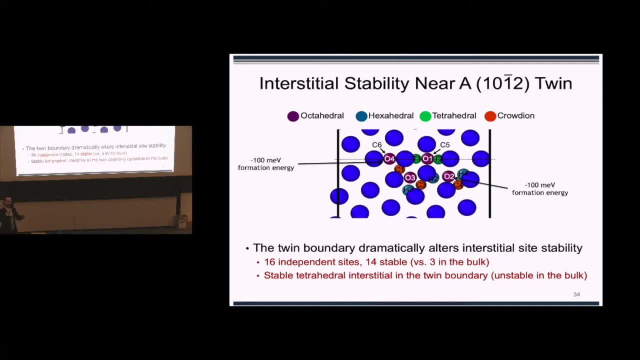 and we've gone in atomistically and placed an oxygen atom in all the different sites or in all the possible sites around here, one at a time. So what I'm showing is all the sites together, because I don't wanna make 16 pictures. 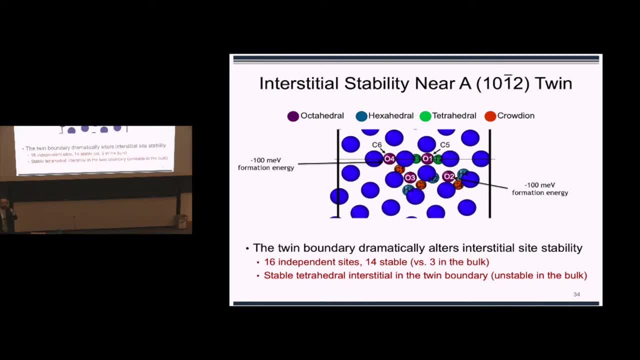 They'd be too small, But these actual simulations of an individual oxygen interstitial. And so what we find is that there are 14 stable interstitial sites near between In bulk titanium there are three octahedral, hexahedral and crown. 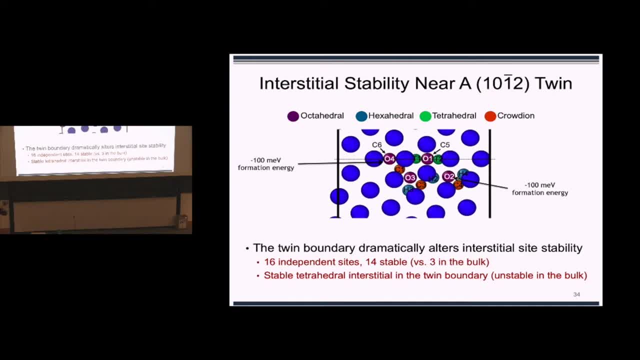 So this twin, this unique geometry, creates a whole bunch of different symmetries that don't exist in the bulk, A lot more sites where oxygen can live. Very importantly, two of those, these two octahedral sites, have a formation energy. 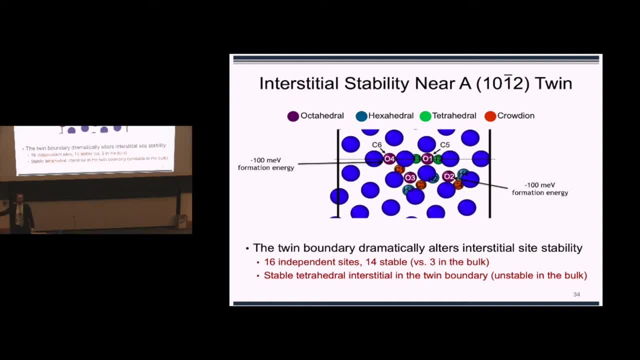 that is 100 MeV lower than the formation energy of oxygen in the bulk. So this means that oxygen will in thermal equilibrium. this means that oxygen will be attracted to those sites with a higher concentration of oxygen at the time. So this is the first piece. 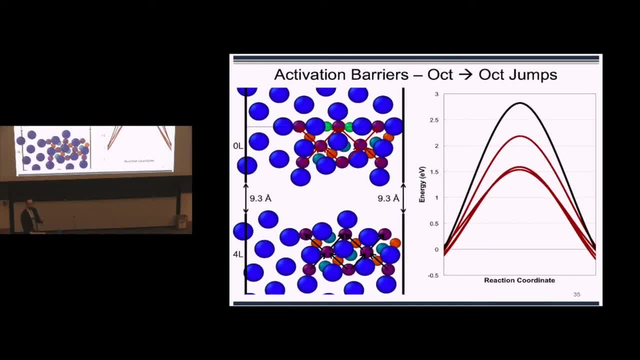 And then the second piece is again calculating these activation barriers. So the way that we did that was we ran a whole bunch of calculations And I'm gonna show a few slides that look like this, So I'll spend some time on this one explaining what it is. 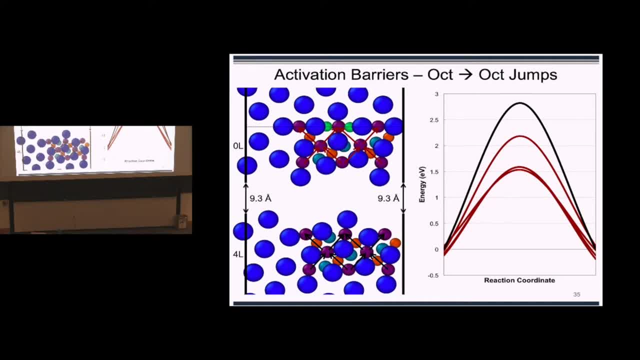 And then we'll kind of jump through the next few. So what I have here is a relatively large simulation cell. I don't have to put the whole thing up here, But basically I have some body of material that's four layers away, four twin layers away from the twin. 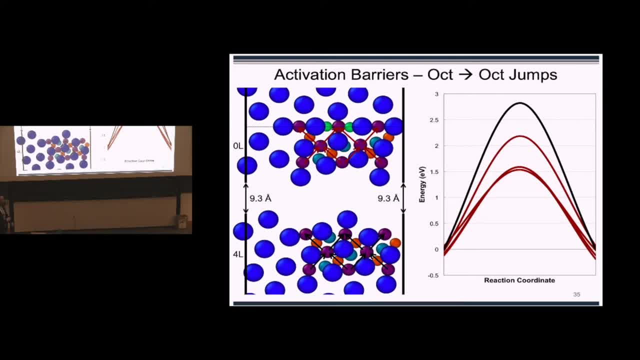 So I'm 10-ish angstroms, And so the first thing I wanna do is I wanna calculate the activation barrier for a jump of an oxygen interstitial in an octahedral site to another one, But I wanna do that for all of the possible octahedral sites. 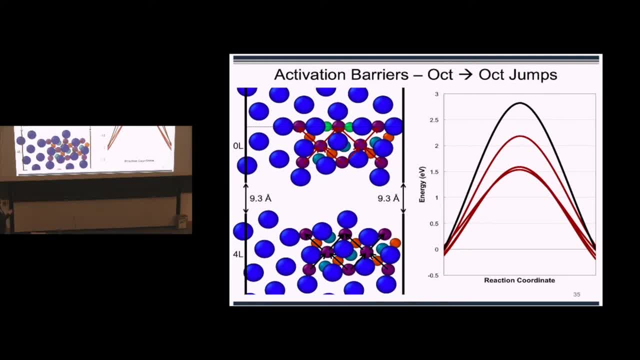 way down here in the body of the twin. So I run these eight calculations And I simulate, I guess, the activation barrier for that diffusive jump And what I get is this value: 2.7 eV. There are eight lines there, right. 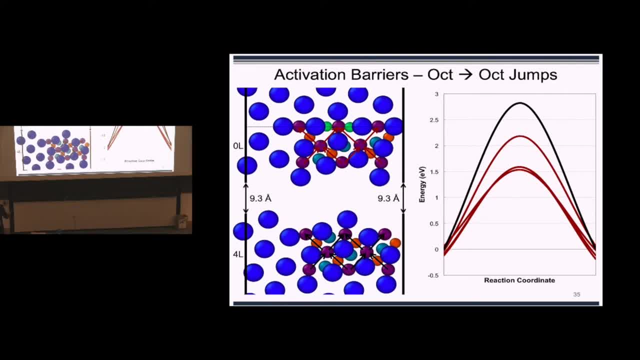 You just can't tell because we're far away in the bulk And, like I said, there's only one octahedral site in the bulk, So each of these is symmetrically equivalent. So really, what this does is it tells us that our model is working reasonably well. 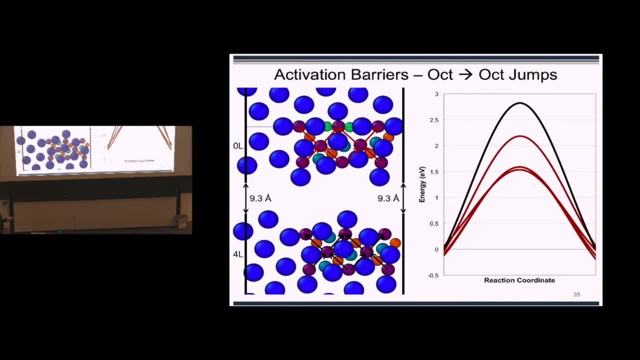 Like far away from the twin, we should get one value, And it's the correct value, However near the twin. I can do the same thing. I can calculate the activation barrier for diffusion for every single one of these jumps, And what I get is the values shown in red here. 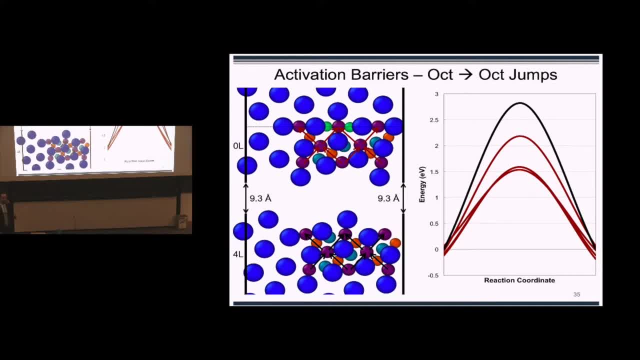 I get a significant decrease in the activation barrier for diffusion of oxygen near the twin right- One more than one eV. That is a very, very large number when you consider the fact that this is an Arrhenius process, right. 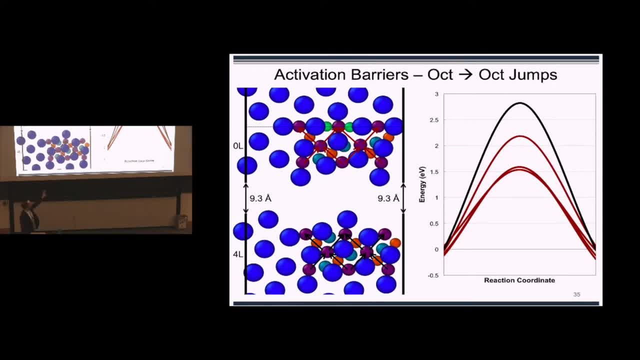 This is an activation barrier type process. So I do this for all the octahedral jumps. I do this for all the octahedral crowd ion jumps, And so what I see here is that I get some extra jumps to some new tetrahedral sites. 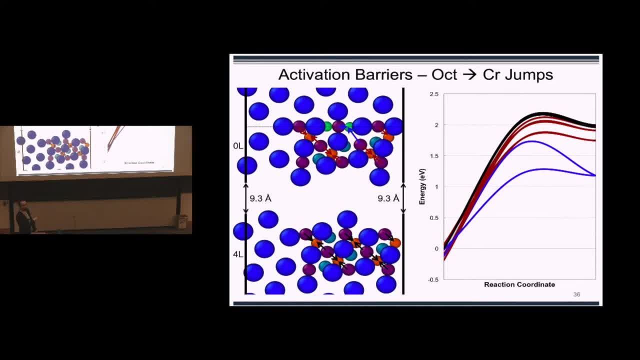 The important piece to take away from this slide is again: I have the diffusion. activation barrier in the bulk is relatively high And as I get close to the twin I get this new network of sites that I can jump between that have a much lower activation barrier. 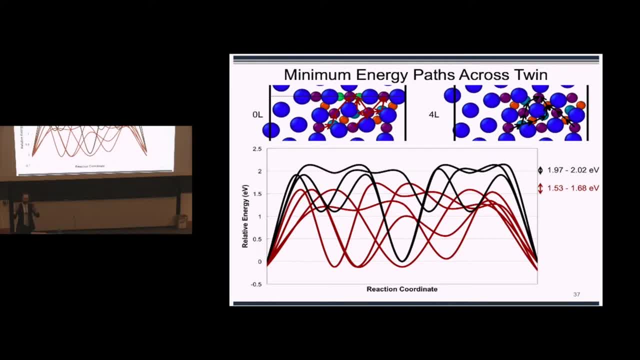 So I do this again and again, and again and again for every possible site-to-site jump far from the twin and close to the twin, And so this is many, many hundreds of simulations. This is a place where having some capability in Python or whatever your scripting tool of choice is, is very helpful. 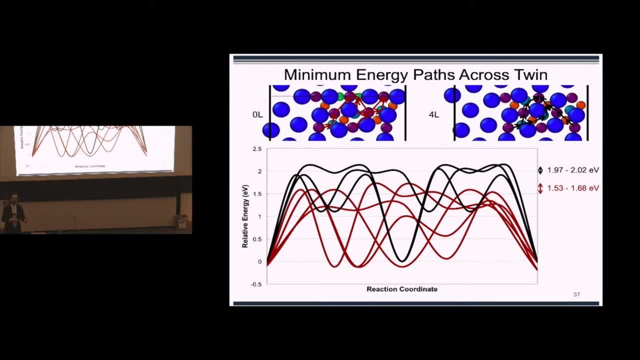 It's hard to run 500 simulations by hand. It's a lot easier to write a script To run 500 simulations. we did that here, And so what I'm showing is far away from the twin. I've calculated every single diffusion barrier. 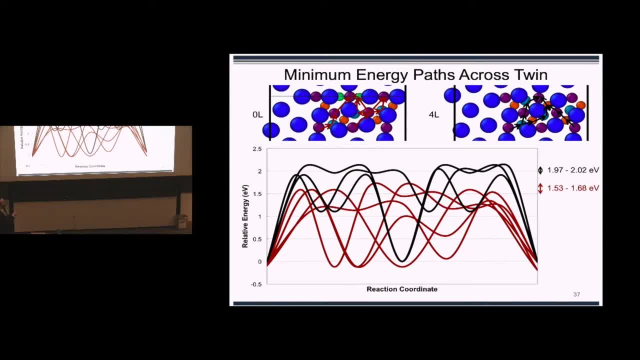 And I've shown those handful of paths that are the lowest energy paths to get from the bottom to the top, to make sort of one layer move of oxygen across. And so there's all these paths shown in black here And what you can see is for each one of those paths. 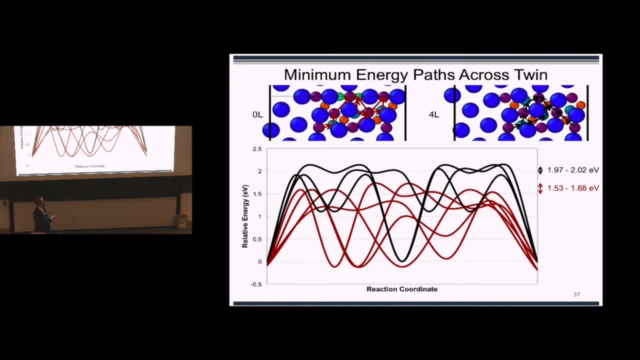 the highest barrier that the system has to go through is about 2 eV And I do exactly the same thing Far away from the twin and I get all these different activation barrier paths And I find that- or excuse me- close to the twin. 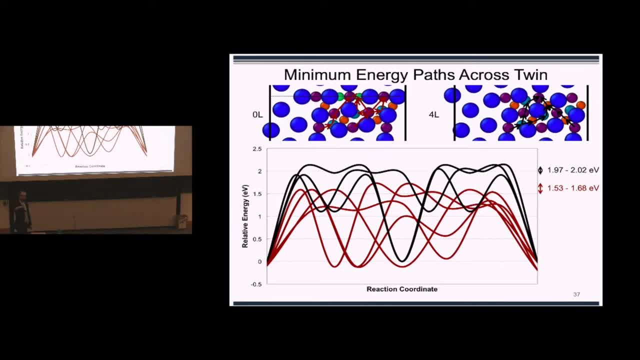 And what I find is that, close to the twin, the maximum value of the activation barrier that the oxygen has to get over is much lower: 1.5 to 1.68 eV. So we have indeed reduced the activation energy for diffusion. 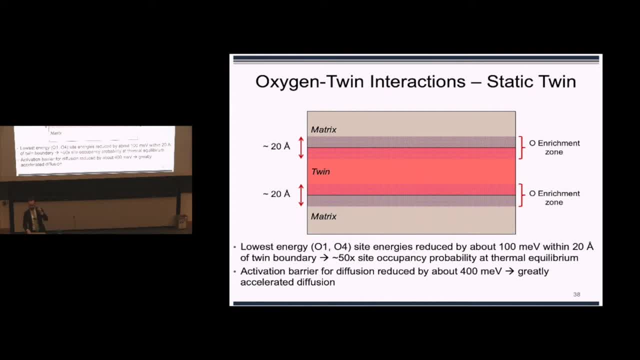 by proximity to the twin. So this gives me two results that help understand what's going on in the system. So the first one is this: Oh, Apologies, The colors are a little different up there than they are down here, But that's all right. 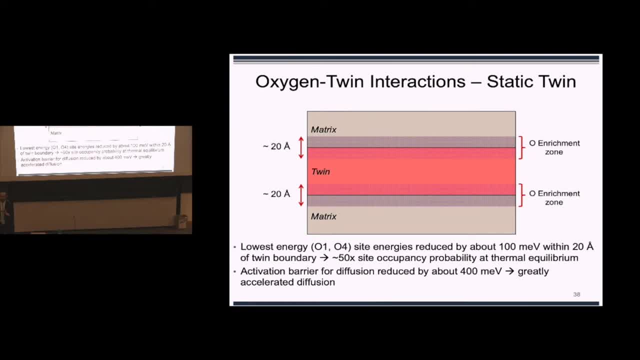 So I can use this information to say two things about what's going on here. One: is there oxygen at the twin? Is there an opportunity for oxygen to interact with the twin? And the answer there is absolutely yes. So what we find is that there are lower energy. 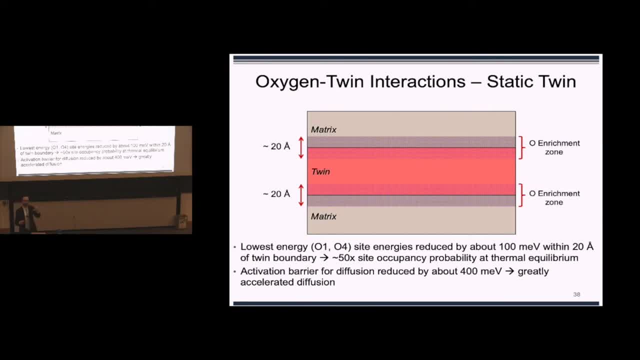 interstitial sites. it's about 100 meV lower And those sites extend to about 10 angstroms from the twin down here. So what that means is there's going to be a 20 angstrom region around that twin boundary with a much higher concentration of oxygen, if you actually 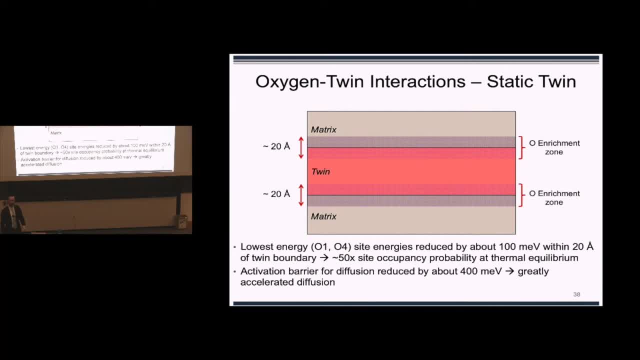 calculate it for thermal equilibrium: 50x site occupancy near the twin. So what we should have is this sort of band of oxygen enrichment around each of the twin boundaries. So there's absolutely an opportunity for oxygen to interact with the twin. Now the question is: is the process now? 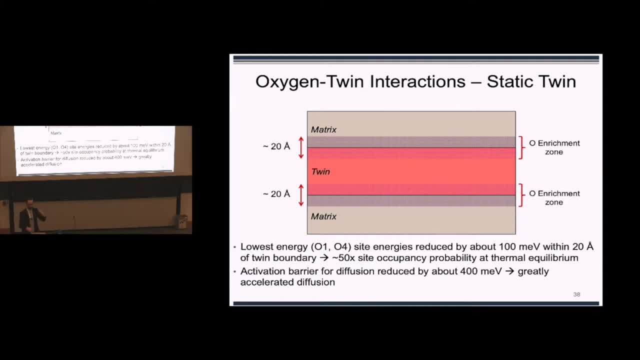 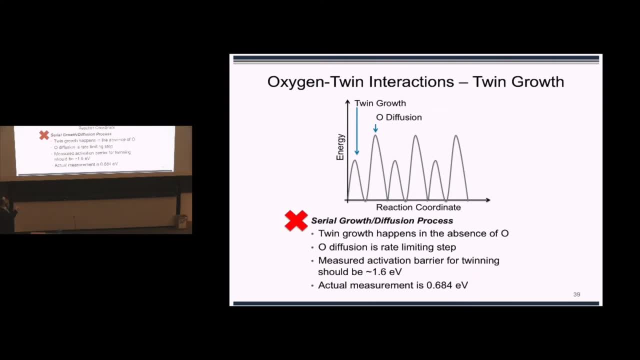 that the oxygen has to diffuse and the twin grows. the oxygen has to fuse and the twin grows. I think in that case the answer is no, And here's why. So if that was the case, the energy of the system as it moves along would look like this: Twin growth: diffusion, Twin growth. 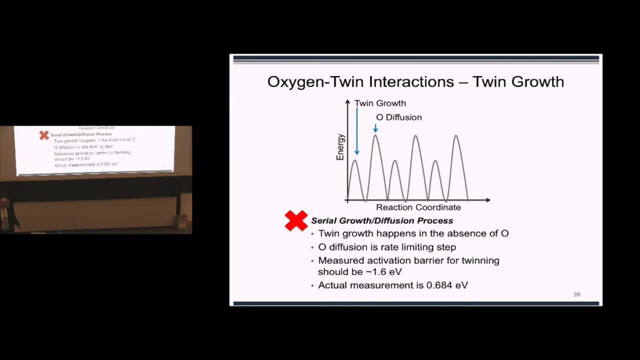 diffusion And I would measure the sort of overall activation area of that system to be that of oxygen. So in the simulations I just ran I got a value of about, let's say, 1.6 dB. So that's lower right. The reported values in the bulk are 1.75.. My calculated values in the 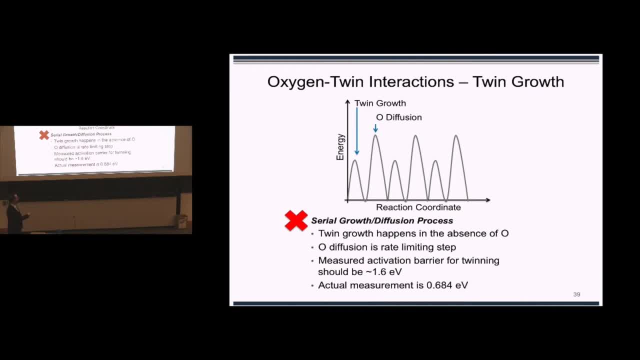 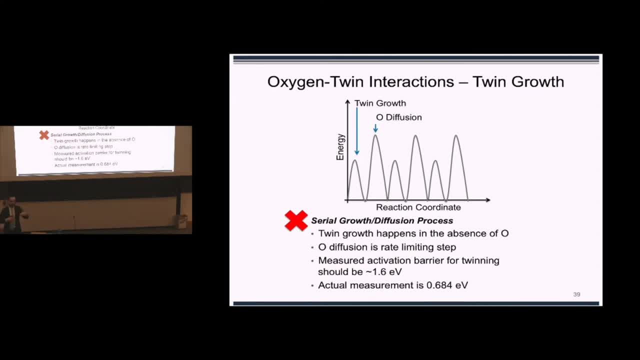 stepwise process where the twin grows the oxygen diffused, the twin grows the oxygen diffused. that's probably not what's going on here. What we have is a dynamic process where the oxygen interstitials and twin growth are moving together right, And these are static calculations. We can't 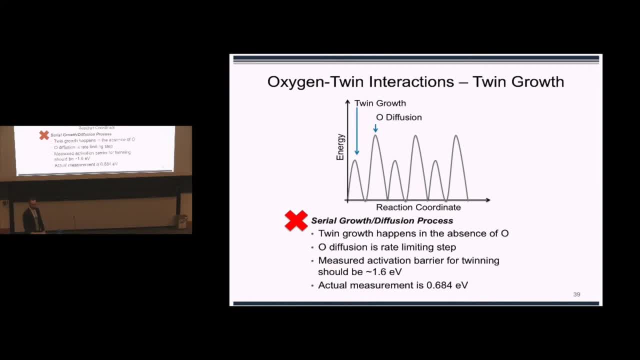 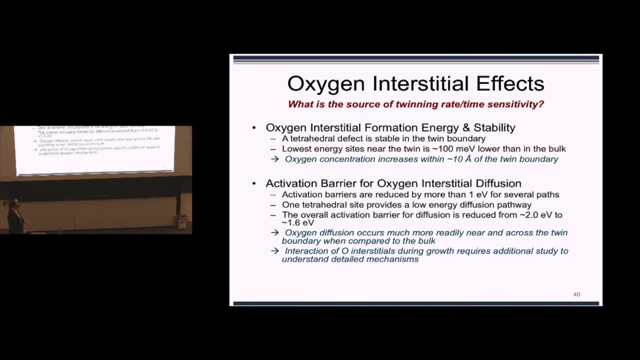 see that in these sorts of calculations. So wrapping this oxygen interstitial bit up, basically what is the source of twinning time sensitivity? So definitely there is an opportunity for oxygen to be influencing. We have a strong concentration of oxygen near that twin boundary. The formation energy is very low. There are a ton of sites. 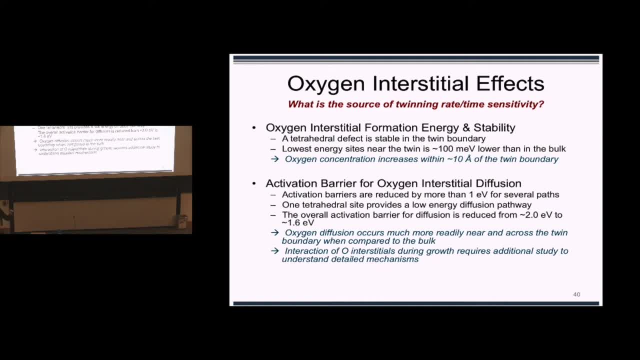 relative to the bulk. However, the activation barrier story is not as clean, And so, basically, yes, it's easier for the atoms to diffuse, But no, it's not 0.6 dB. It's not that value that we measure. the activation barrier for twinning that we measure experimentally, And so that tells. 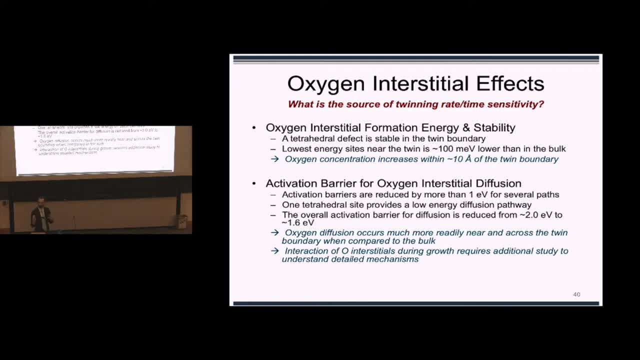 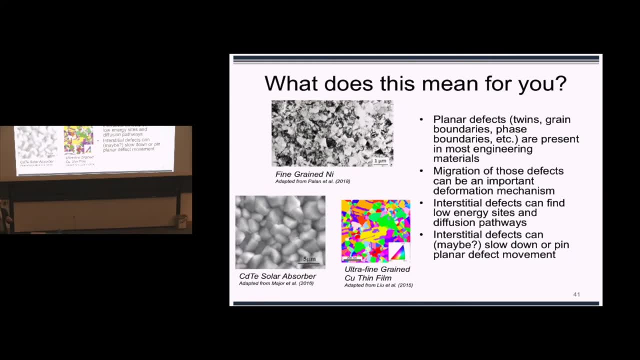 us that this is probably a dynamic process and that these static calculations aren't really kind of good. So I'll wrap up with this, similar to the elastic interaction piece. right, I talked about how those- how you might incorporate those in your research, And we'll talk a little bit. 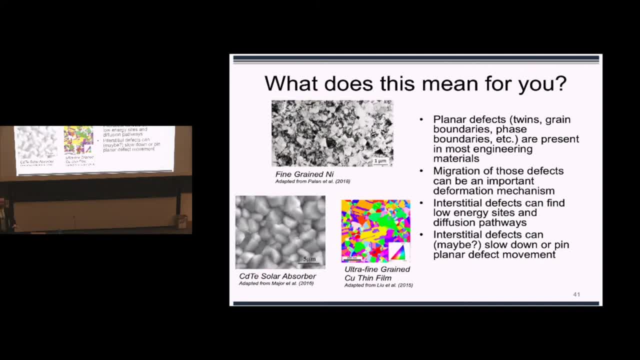 here Twins are planar defects. Brain boundaries are also planar defects. There are a lot of planar defects in engineered material systems that influence their behavior. Here we find that oxygen has some sort of influence that we're still kind of trying to understand. But you may find in 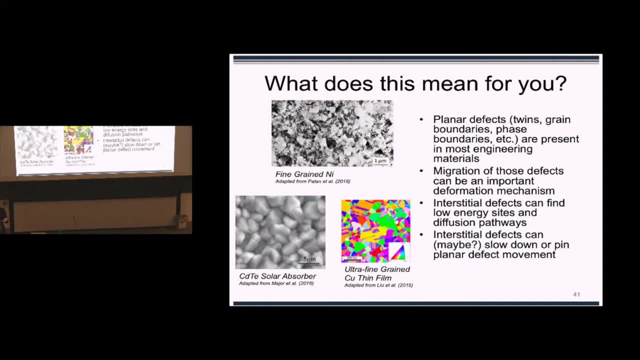 your own systems, that interstitials have an influence that you would like to understand or you would like to manipulate. So I've shown in particular, some very fine-grained systems or cad-tel solar observers, which, to my knowledge, are sensitive to grain size, And so these sorts of mechanisms are available for you as 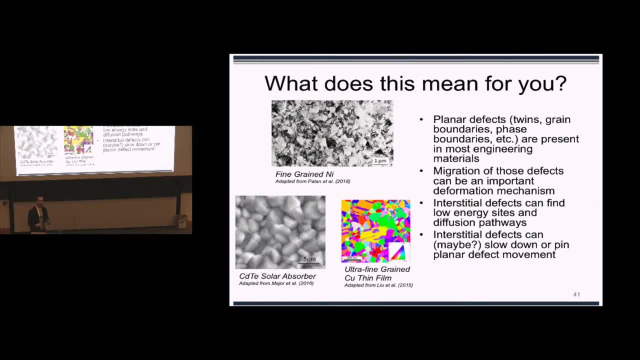 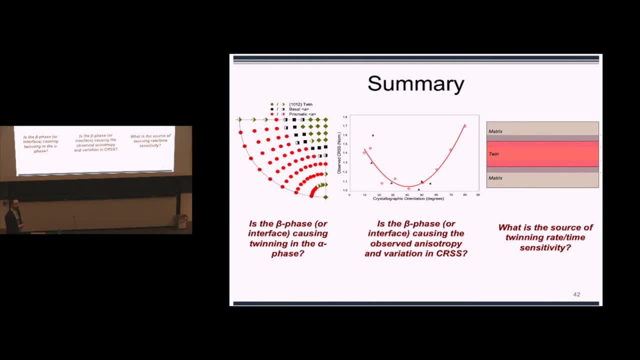 materials engineers or as people who practice materials engineering to make your systems better. So with that I will just put up this summary of those three outcomes. So is the beta phase causing twinning in the alpha phase? I personally don't think so. I think there's some. 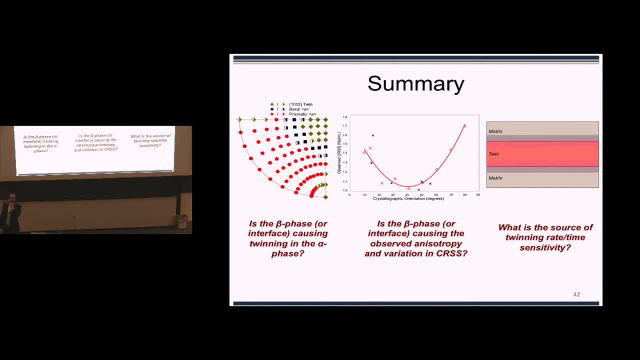 work to do. there Is the beta phase causing the observed variation. Is the beta phase causing the reduction in critical shear stress in alpha as a function of orientation? Yes, I do think it is. And what is the source of twinning rate and time sensitivity? I think it's still up for debate, but we absolutely have oxygen in very 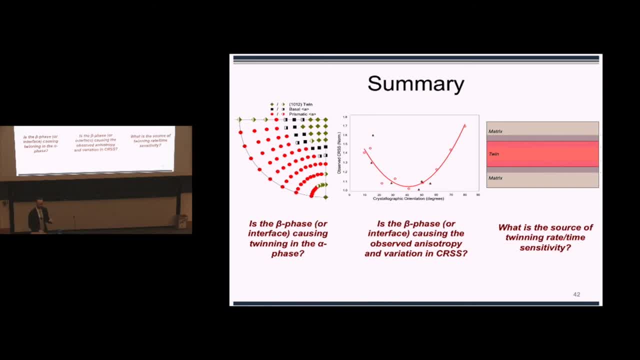 high concentrations in that twin. that could play a role, and very well may. So with that, I will leave it right there and I would be happy to answer any questions. Thank you, Thank you. Well, I'm fascinated about the growth of twins and all that's calculated, But as I vaguely remember in the models early on about twins going sideways by the passage of 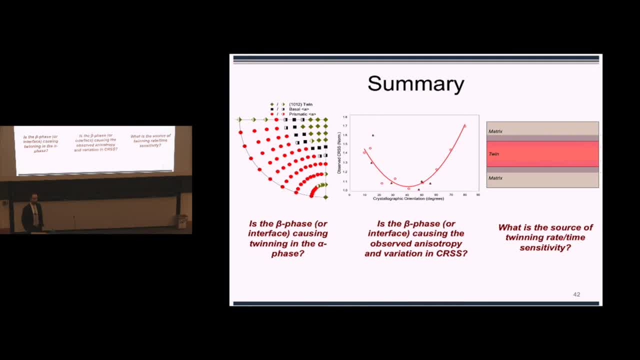 partial dislocation, one after another. the whole rabbit grows the twin by super-closing forced partial dislocation Right. Couldn't it be that in the partial at the twin boundary there are special sites in the oxygen that have a different energetic profile? 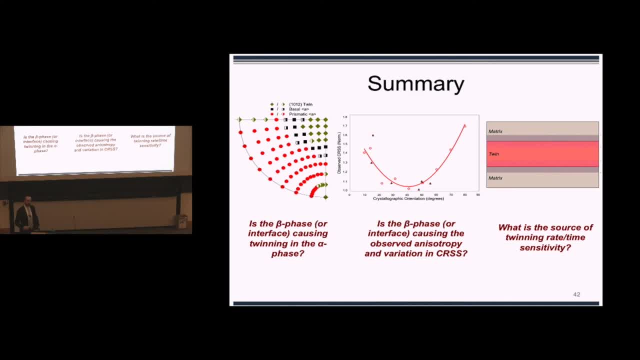 Yes, it absolutely could be. So in the case of FCC metals the passage of partials to form the twin is established right. That's concrete. In HCP metals there's actually some debate in the field still about: is it partials, Is it some kind of? 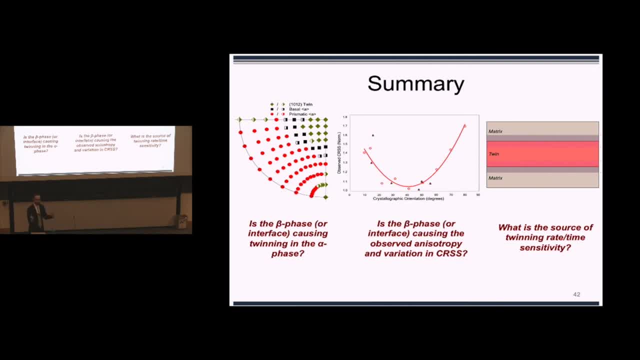 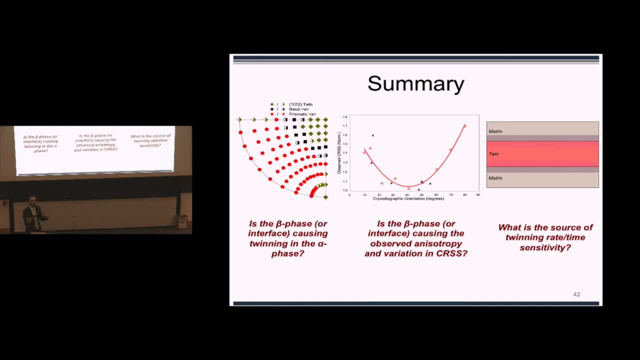 So again, that's part of kind of an artifact of doing these in a very static way. You know, we've sort of shown that before anything happens at the next time, this is what's going on at the twin boundary, But the next step really is to move into. okay, now with growth, how does it interact? 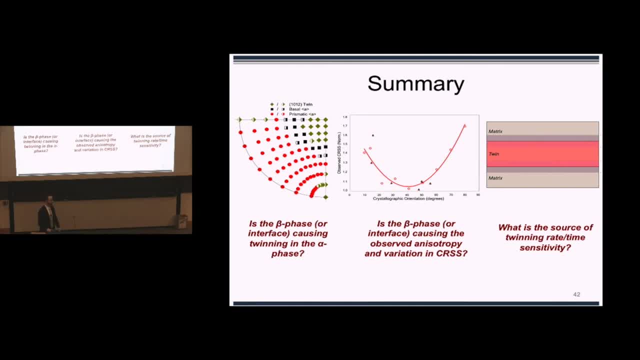 Yeah, Yeah, Yeah, Yeah, Yeah. or it's like: how do you handle it? Yeah, So can the model actually tell you what's the equilibrium, concentration or solubility near those things or things like that? Yes, 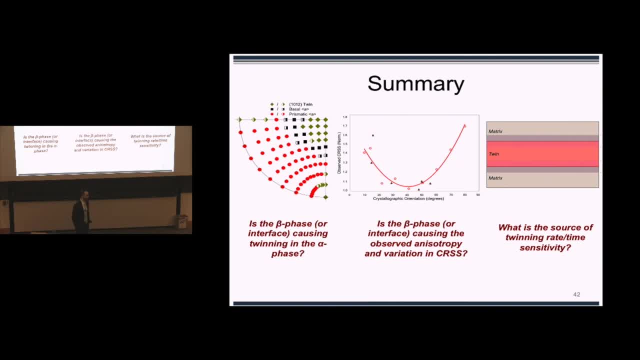 Yeah, equilibrium, absolutely Okay, Yeah, So what's the rough number? What's the concentration of? I do not remember. All I remember is that at the twin it's 50 times higher. Oh, I see, Yeah, but I don't remember what the baseline is. 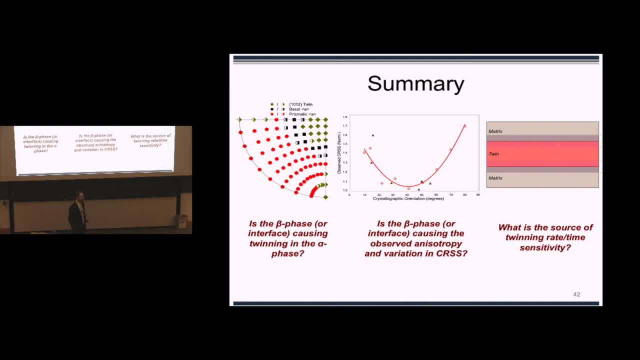 So it's very dramatic. Yeah, exactly, It's very dramatic. yeah, But to your point, you know that sort of simulation. you know if I was to have to do that for copper in, you know whatever, some 3-5 system. 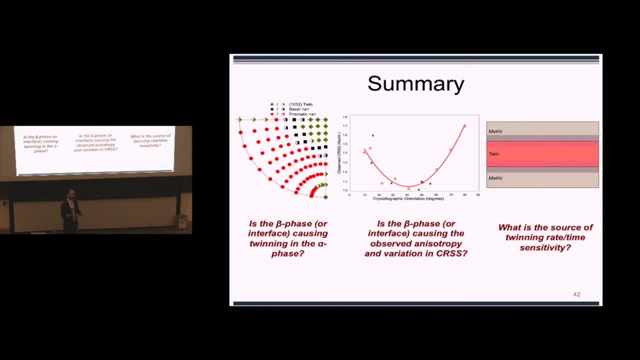 that's a place where you can really go straight to DFT. You can fit. grain boundaries are nice in DFT because they're periodic simulations and you can just line the grain boundaries up, put the edges and they continue to infinity. 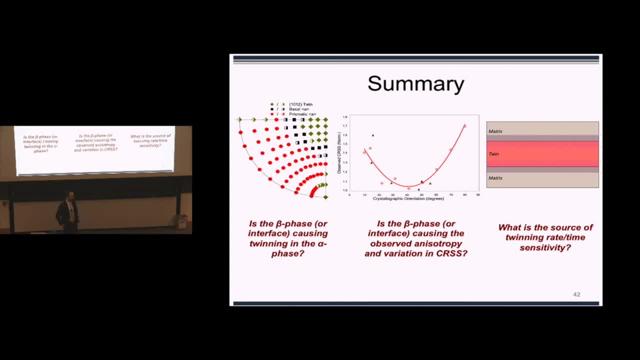 So those sorts of calculations are fairly approachable. Yeah, Good question. Sure, How do people avoid the decrease in titanium alloy? So the best way to do it- and indeed this is in general how it's done, whether intentional or not- 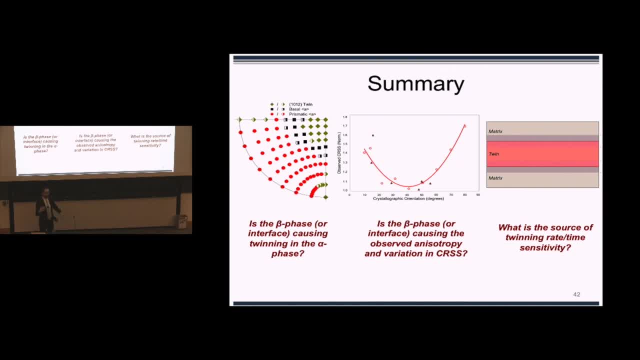 is to alloy with aluminum, which is a very common alloying element in titanium. So when you add a sufficient amount of aluminum to titanium, it increases the stacking fault energy in the alpha phase And the propensity for twinning is strongly associated with the stacking fault energy. 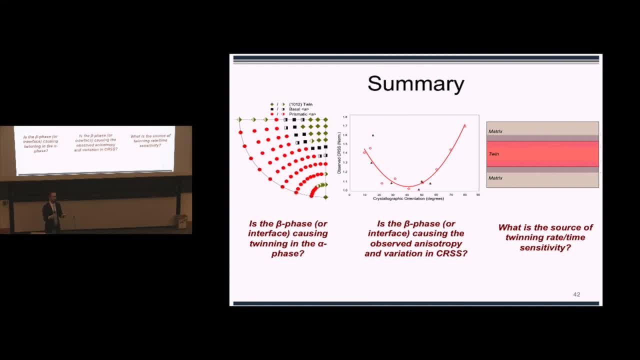 It's I forget which stacking fault, but essentially it changes the energetics so that the system is strongly prefers to form dislocations. You don't get these connecting twins and you get away from creep. Titanium 64? Titanium, yeah, titanium 64.. 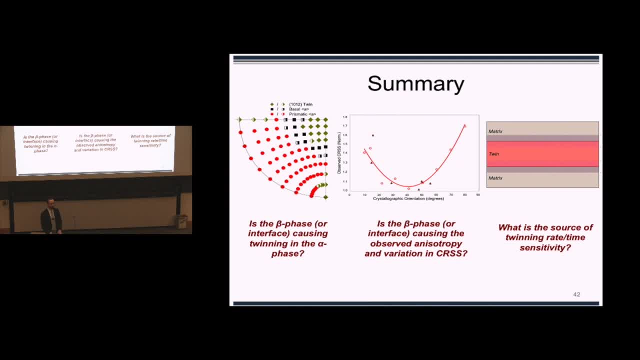 The threshold is usually about four weight percent aluminum. So in the case where you cannot use that- for you know systems where you're exposed to particular caustic atmospheres or whatever else it is, then you're stuck with this problem. 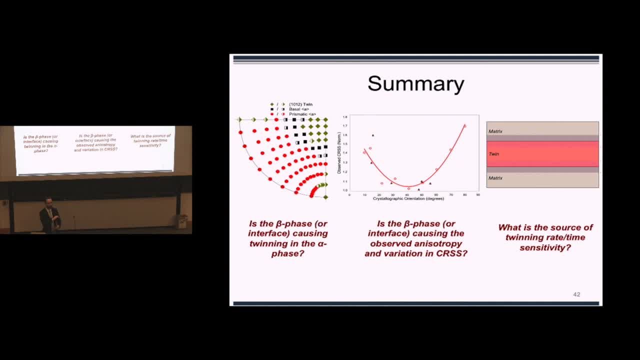 But for jet engine components, for example, we just put enough aluminum in there and that pretty much goes away. I have a question about the altitude content. So presumably you can't get titanium with a value of altitude content, so you don't. 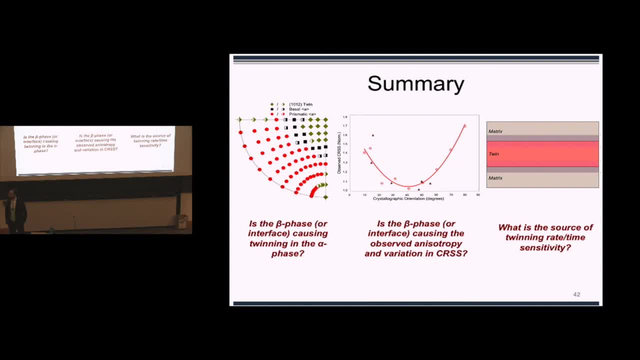 Right, exactly. So that would be. the perfect experiment to run would be to have six, nines titanium Boop, So it's the other way around. Presumably you do get the strength of that, so you can see the yield stress. 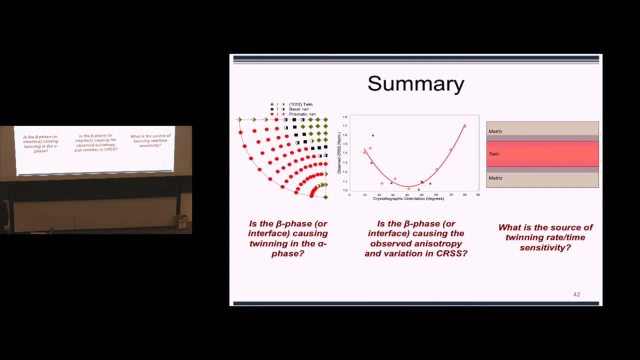 You do, yeah, Yeah, And there's some interesting interaction there between variation in yield stress and the variation in propensity of twinning. So you kind of meet micromechanics problems and you can connect the volume fraction of twins, their results, to your stress. 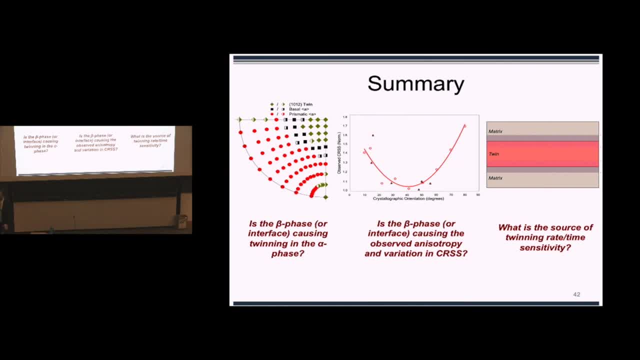